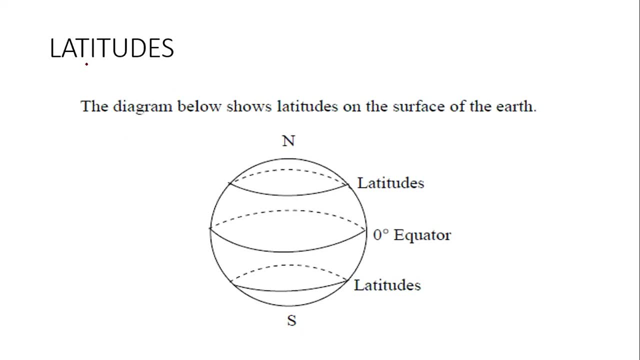 So latitudes are imaginary lines that are drawn on the Earth's surface, and they run from east, from east to west, like this. So now, here, as you can see, this is a solid line that has been drawn. Then behind is another dotted line here. 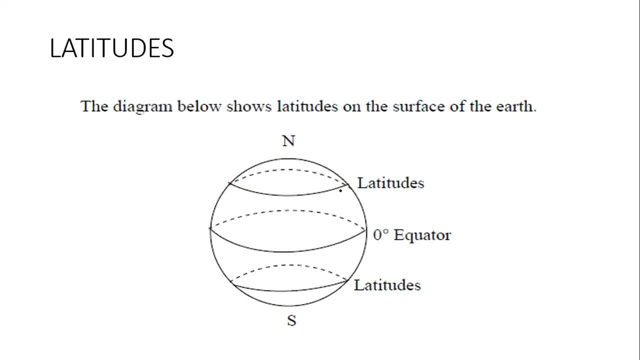 So now, this simply shows that this is the front and this is the back. So this is the same latitude. So at the center of the Earth is the equator. So the equator is the one that is drawn. The equator is the one that divides the Earth into two equal parts, which is the Northern Hemisphere and the Southern Hemisphere. 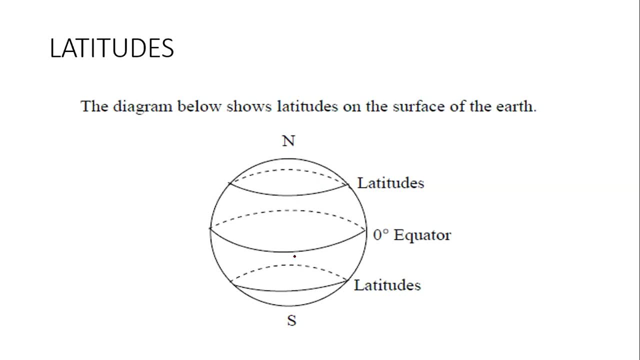 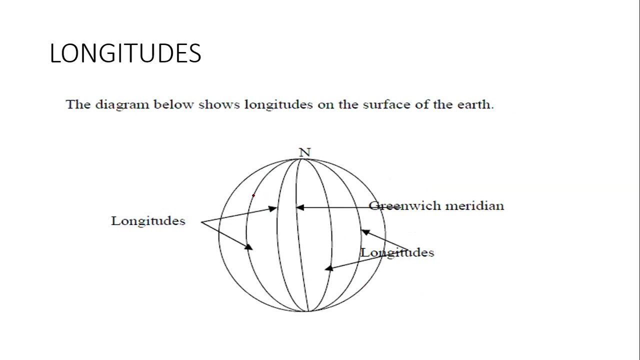 So the equator is the middle latitude that will divide the Earth into two equal parts. So remember latitudes, the latitudes, they run from east to west. All right, Then we also have what we call longitudes. So these are imaginary lines that are drawn on the Earth's surface, and they run from north all the way up to the south. 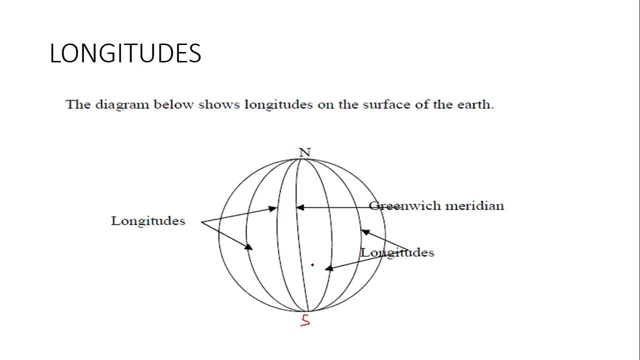 So the longitudes, they run from north all the way up to the south, And these longitudes, they are very useful when it comes to calculating time. So longitudes are useful when it comes to calculating time. The longitude that will divide the Earth into two equal halves, into the western side and the eastern side. 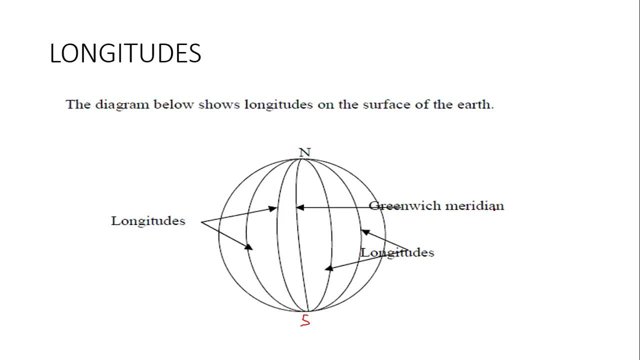 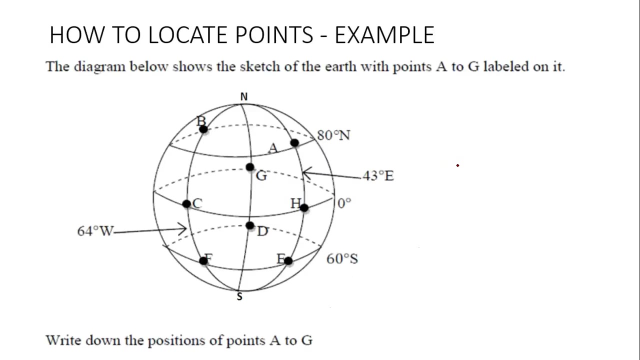 This is called the Greenwich Meridian, And most of the time, the times of the world are calculated from here. Hence the name GMT, which simply means Greenwich Meridian Time. Okay, So we begin to look into our issues, which is how to locate points. 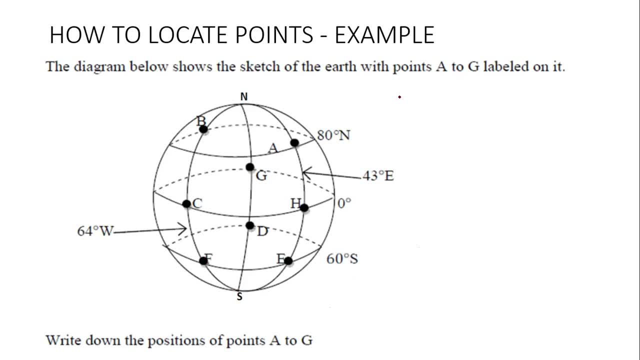 Now, how do we locate points on the Earth's surface? So point number one here is: always remember when you are locating the points that are located on the surface of the Earth. we always write them in forms of coordinates, Just like the way we write the x- y. 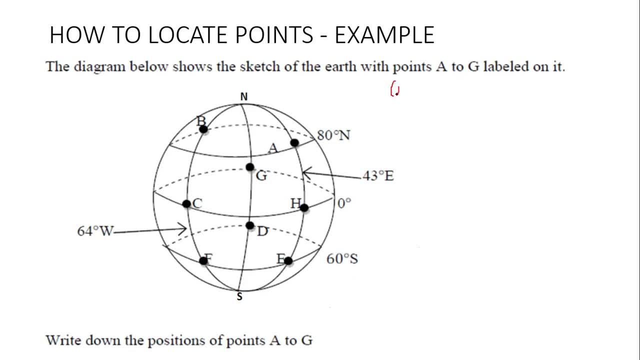 But when it comes to Earth geometry, here we are going to write latitude, Okay, So latitude, longitude. So that is how we write our coordinates: Latitude, longitude, For example, this question they are saying: write down the positions of the points A to G. 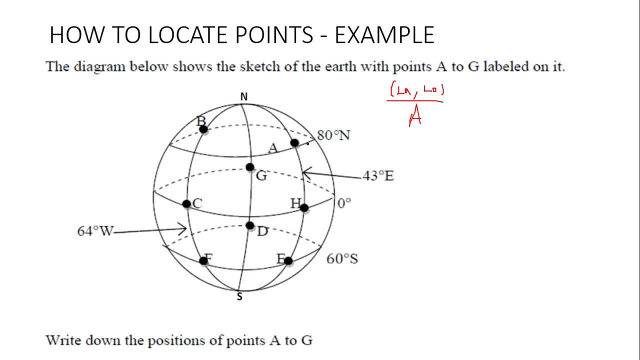 So if we are locating A, we first of all have to check where is our A. So our A is right here. right here, This is where our A is, And here you can check the latitude that is, there is 80 degrees north. 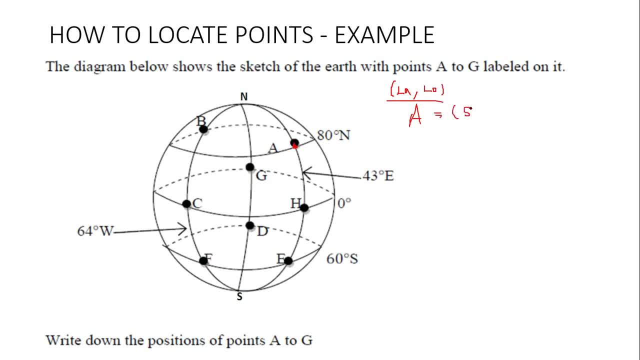 So A? here you write 80 degrees north, So this is 80 degrees north comma, So this is latitude. Then what longitude? So the longitude is this one here, this one here, as you can see, And it is labeled as A. 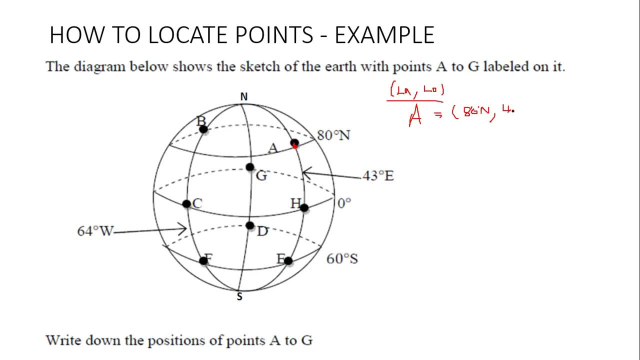 43 degrees east. So we have our 43 degrees east. Alright, Then we go to B. B also, like I said, since this one is just a dotted line, it shows that it is behind this one that is in front. 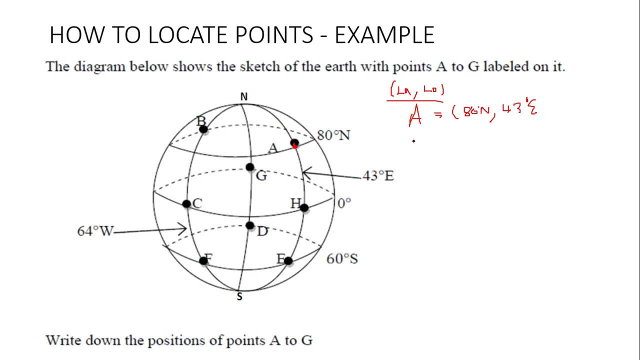 So it is also equally 80 degrees. what North? So if we are to locate the point B, this one will also be equal to okay, so that is 80 degrees north, 80 degrees north, Comma. So we check this one. 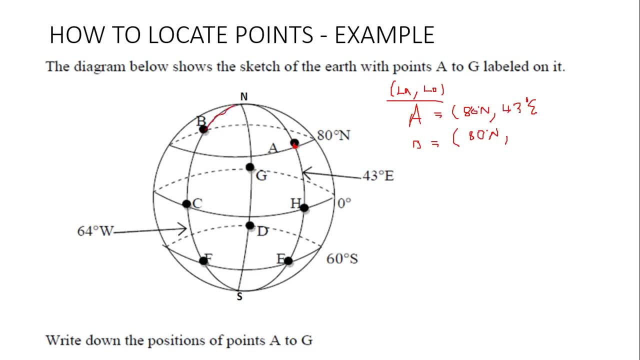 It is on this latitude here. Okay, So this is the latitude, We follow it. We follow this latitude. You can see it is labeled this one here, which is 64 degrees west. So we have our 64 degrees west. 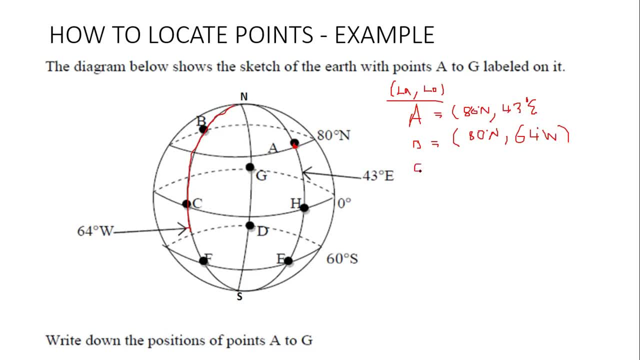 Okay, So that is B. We can proceed C. Let's locate C. C is here, So C is actually on the equator here. This is zero degrees, So zero degrees. there is nothing like it is northeast or whatever. 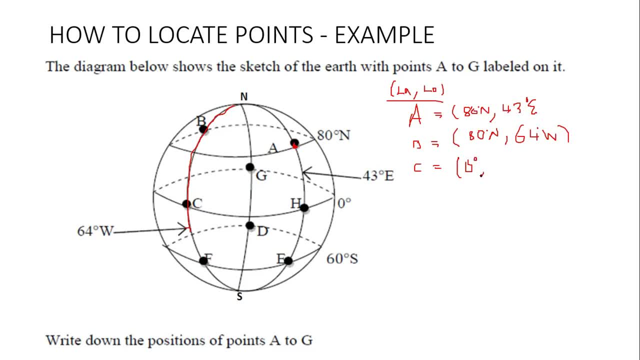 It has got no sign. So we just write zero degrees comma and we look at the longitude. Okay, The longitude is to be 64 degrees. what West? So please- I am emphasizing, I don't need to check through everything- 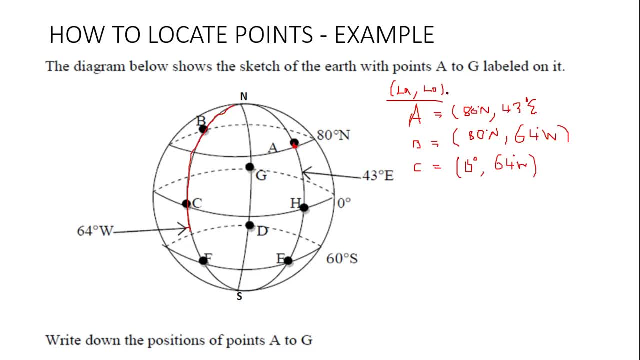 But the point is you have to say latitude, comma, latitude, longitude. So when you check this point, the latitude here is zero, Then the longitude is this one, which is 60. This one which is 64. Hence that one. 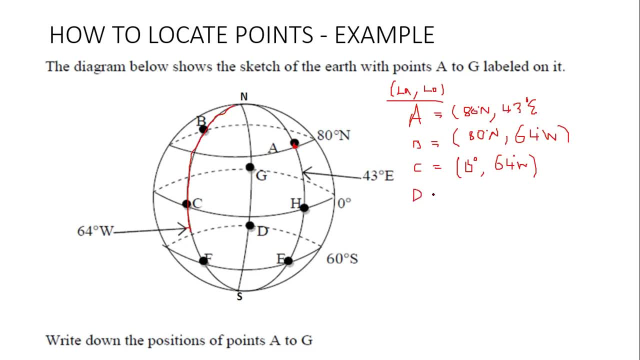 Let's try D, So D will be equal to okay. so point D is here. Now this is behind this one here And when we check, this is 60 degrees what South? So we write: this is 60 degrees south. 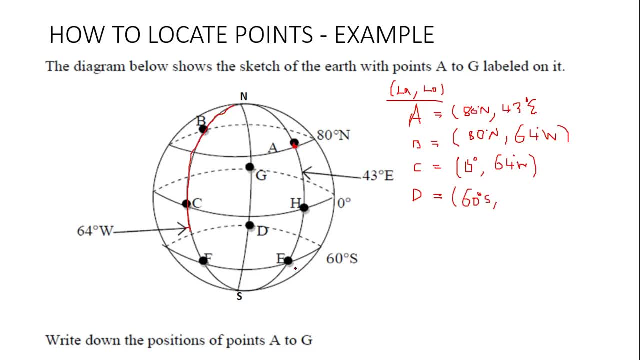 Okay, 60 degrees south comma. Then this is D. D is on what longitude? So when we check the longitude, that is right here. Okay, D, we check the longitude. Okay, Has this longitude been measured? Has it been labeled? 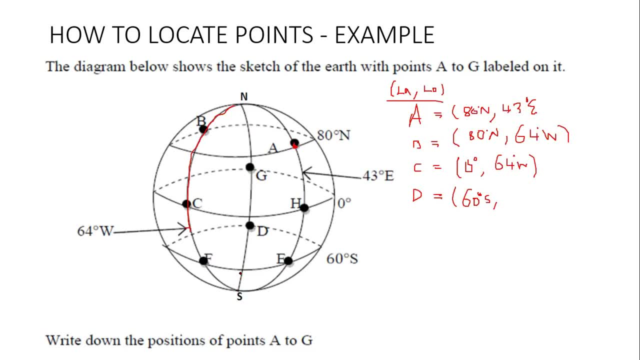 Okay, So this is the longitude that we have there. It has not been labeled, Okay. So let's see on what we have here, So that one is actually the middle, So the GMT, the middle one is also the zero degrees. 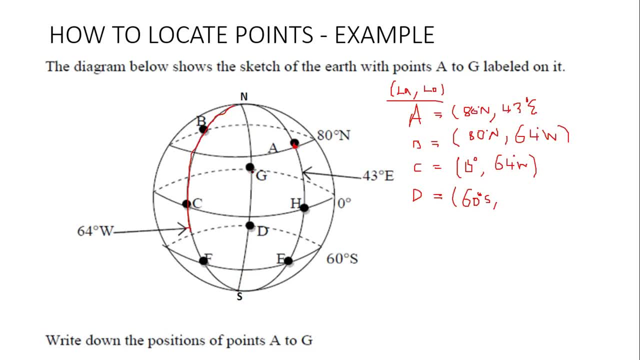 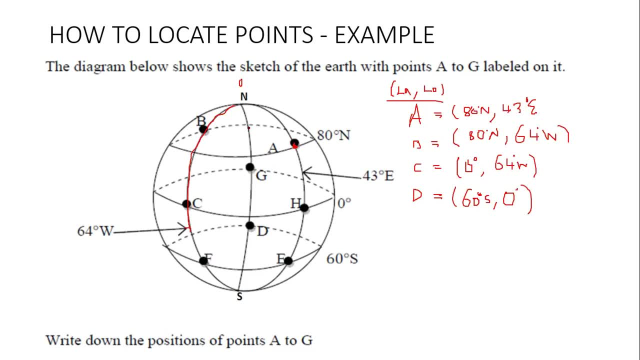 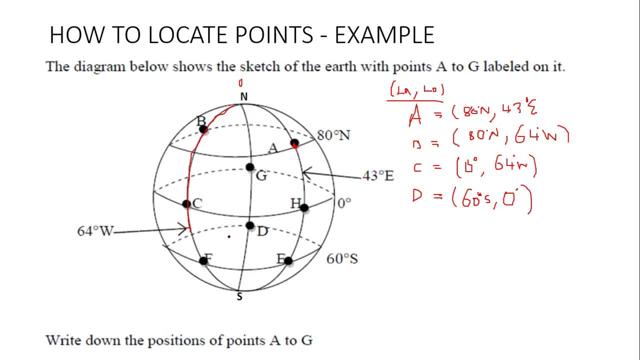 Okay, Okay, Okay, Okay, Okay, Okay, Okay. g is only uh, also zero degrees. so g was zero, comma zero, zero degrees, comma, zero degrees. so, please, locating point is very important, because from locating point we are also going to be able to. 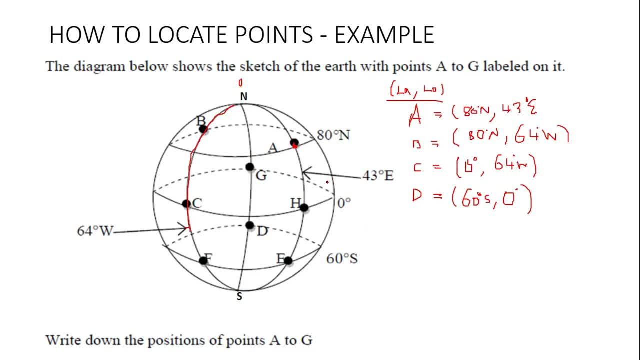 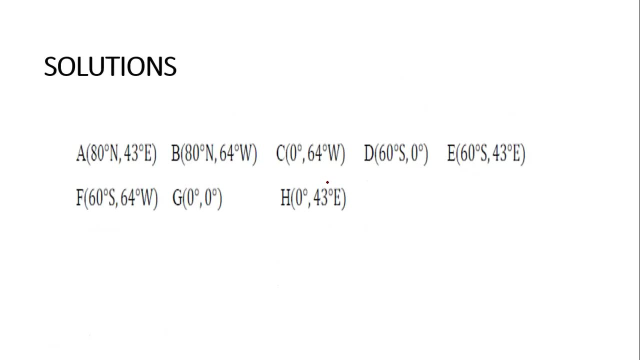 calculate the distances. all right, so you can just go through. these are the answers that we were dealing with. okay, these are the answers that we were dealing with. confirm through and just make sure that everything is correct. so, otherwise, the concept here is this: one is always latitude comma. 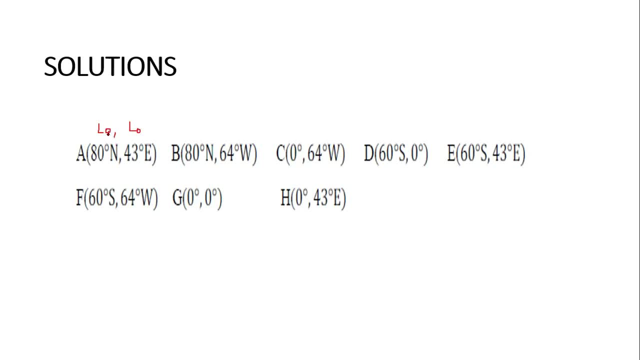 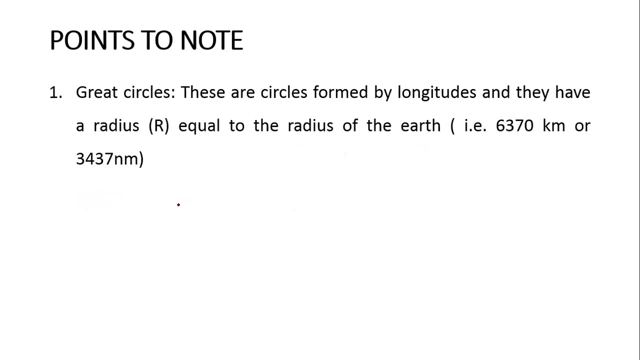 longitude. okay, so latitude, comma, longitude. that is how it is always supposed to be. all right points to note as you are trying to dive into this subject and just calculate all the concepts. the first one is that great circles are circles that are formed by longitude. so there are two circles. on the f, we are saying the f forms two circles. 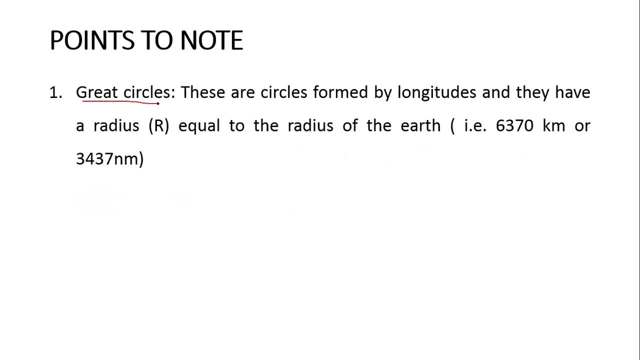 there is what we call the great circles. now, the great circles, these are the circles formed by rt longitude, so a circle along a line of longitude is known as a great circles. and these great circles, their radius, are equivalent to the radius of the earth, which is 63 uh, 63, 70 kilometers or 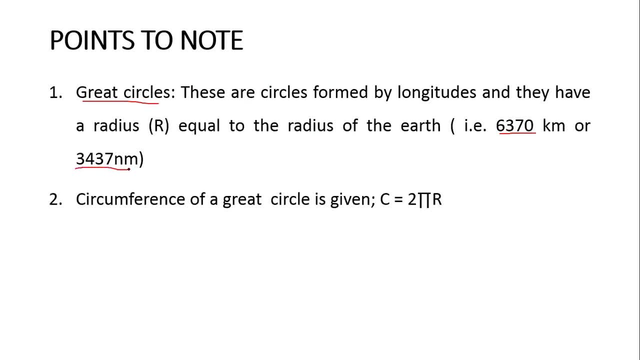 34, 37 kilometers. all right, we also have, uh, the circumference of a great circle, which is given by this formula here. so this is just two multiplied by the pi, multiplied by the error, which is this one. so calculator r is always that one there or this one in nautical mouse. all right, then we also have what we call a. 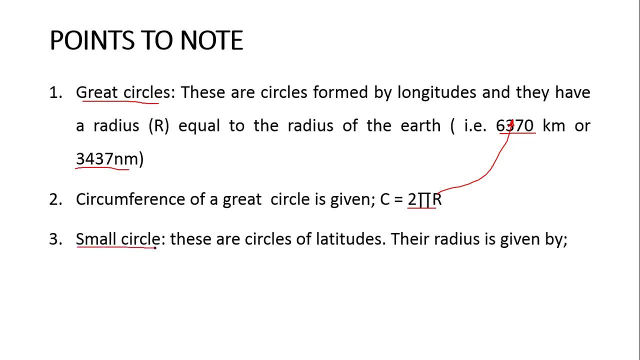 small circle. so a small circle is simply a circle along a line of latitude. so small circles are circles along a line of what latitude and their radius is given by r. uh, small letter r is equals to calculator r, cos, c, x. now, this calculator r we are talking about here is the 63, 70 provided you are dealing with. 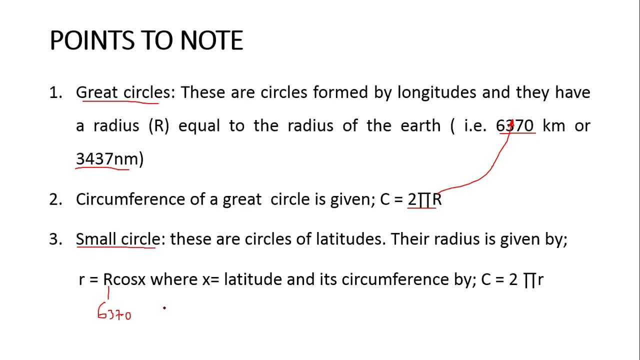 kilometers, then cos x. here it's cos latitude, so that same latitude you've been given. that is it the x that we are talking about here. all right, so the circumference for a small circle will be given by two pi, small in r. all right, and we know that small, small letter r will be given by this one here. all right. so these 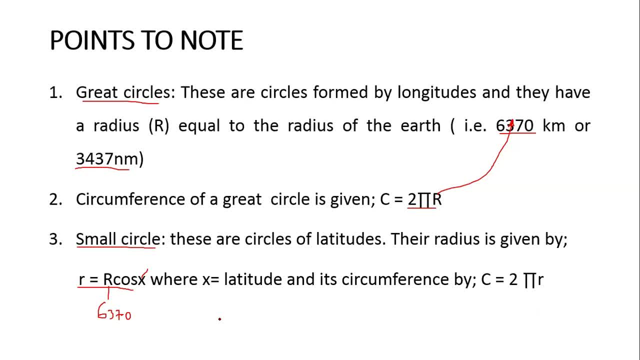 are the few points that you really have to note, as we are going to continue with the calculations of things such as distance along a great circle, and also we calculate distance along a small circle, then we are going to calculate the shortest distance and, finally, we'll conclude this topic by 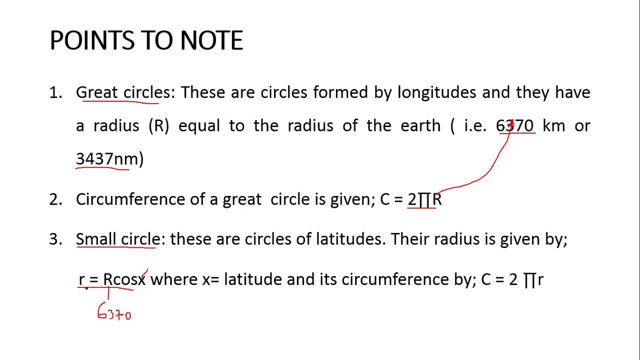 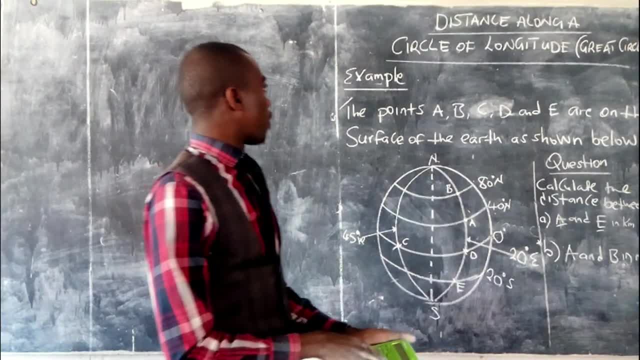 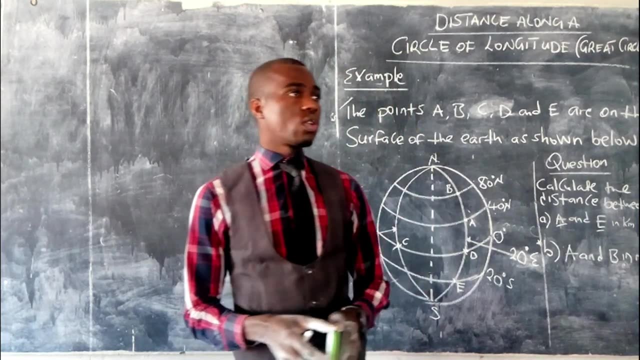 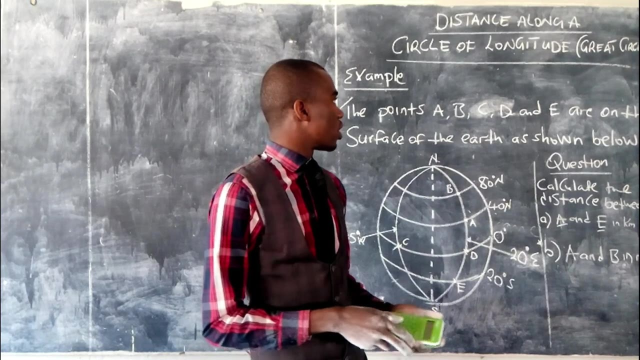 selecting time and also speed. so please enjoy as i take you through these concepts. okay, so I want to know how to find the distance along a circle of longitude. now, distance along the circle only is also known as great circle, so distance along longitude is also known as the great circle. okay. so now we want to use this example to know that when one of your circles is going to be something like this, whatever oueful circle you choose, this way- of silver or even something similar in your circle- is also known as great circle- you cannot know that the distance along the circle of longitude is also known as great circle. so 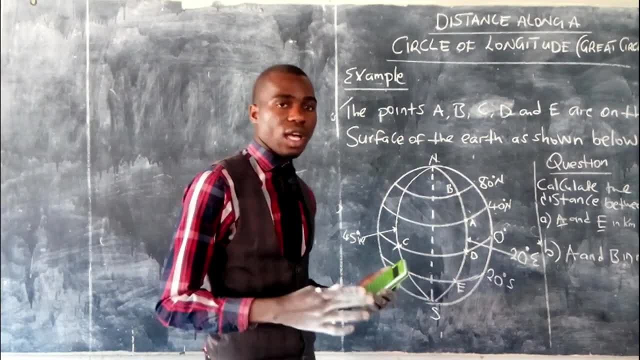 you cannot know that the distance along the circle of longitude is also known as great circle. so now we want to use this example to read it. We are going to use this example just to see how we can calculate the distance along the grid circle. So let's look at this example. 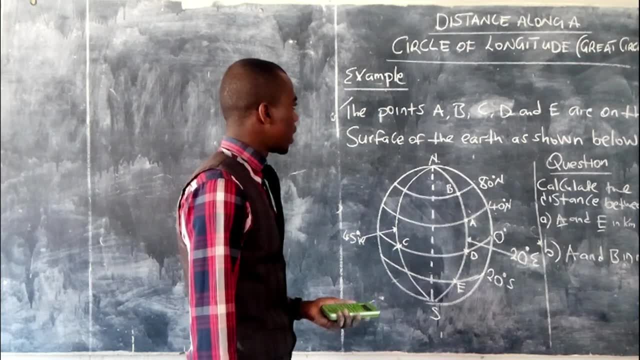 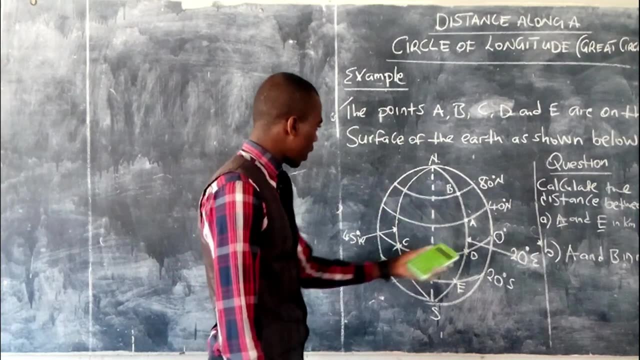 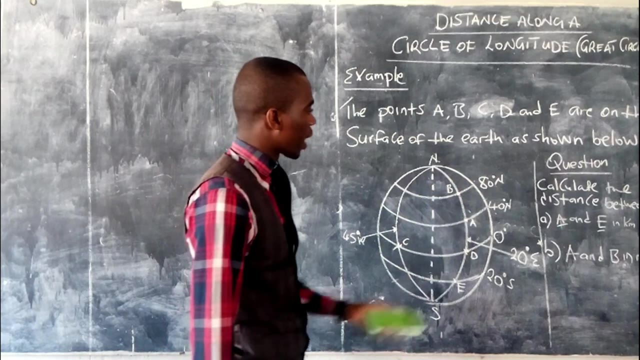 The question reads: the points A, B, C, D and E are on the surface and the head, as shown below. So this is what we have shown here. We have our A, B, C, D and E And the question reads: calculate the distance between A and. 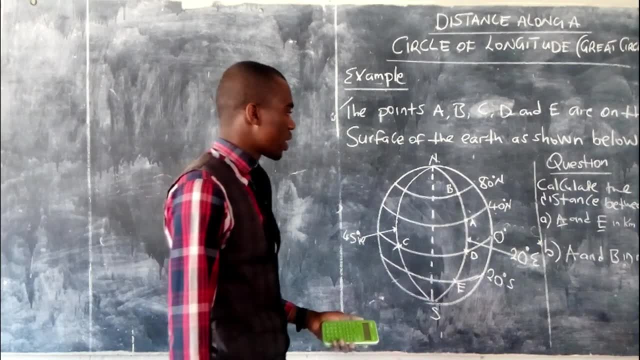 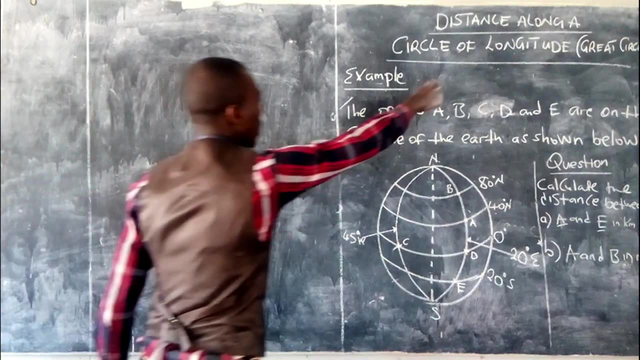 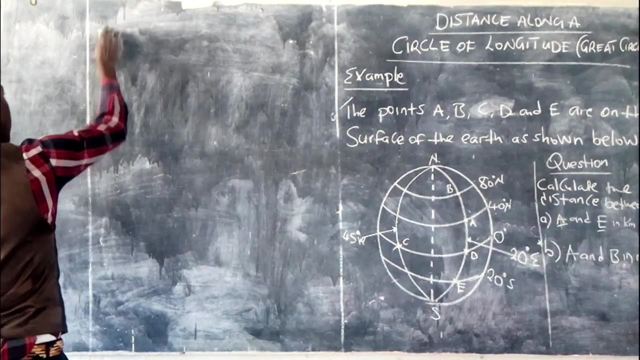 B in kilometers, then B calculate the distance A and B in wattage, not equal miles. Now the distance, as the title suggests. we are dealing with the wattage, not the truth. So the formula to use here is simply distance. okay, 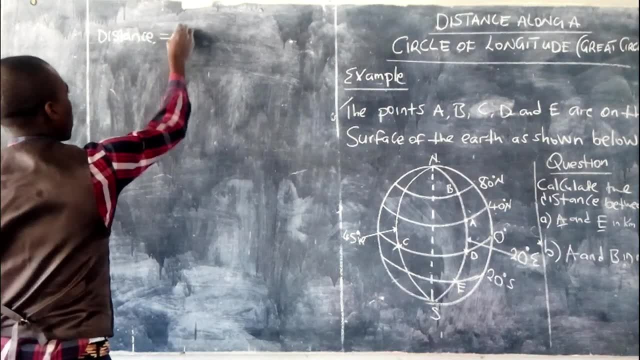 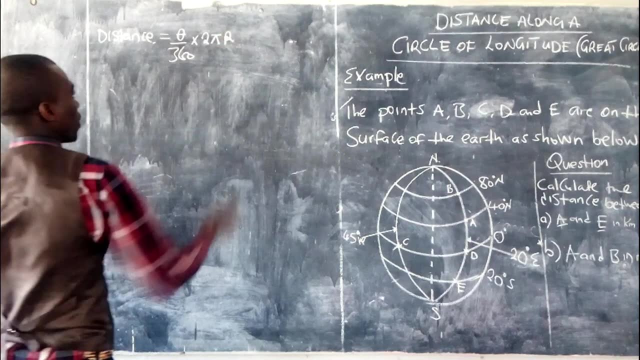 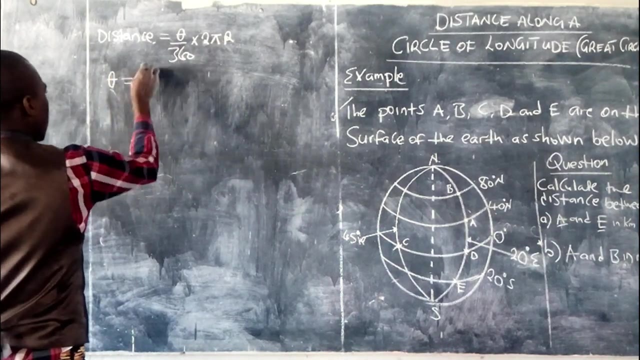 So the formula to use is simply: distance is equal to feature over 350 multiplied by 2, multiplied by 5, multiplied by calculator. Okay, So now let's look at the meaning of this formula, This figure here. it means difference, okay. 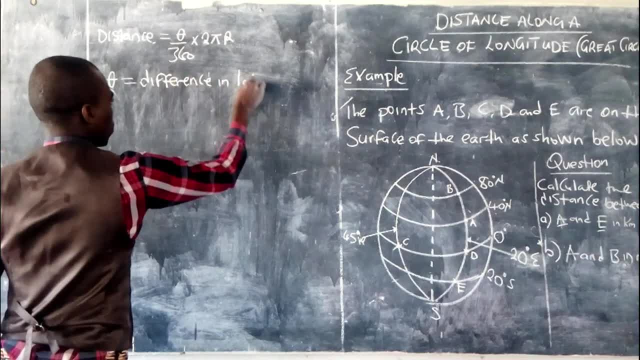 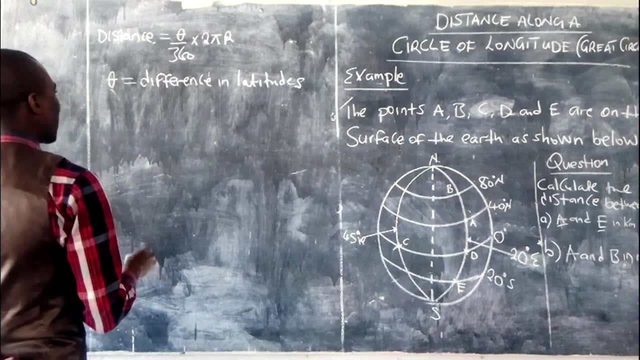 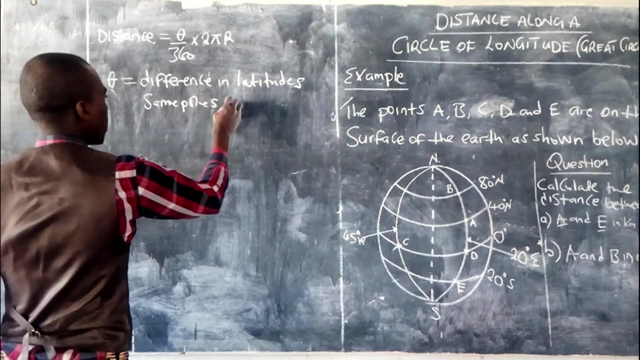 It means difference in latitudes. Difference in latitudes, Now, when we are finding the difference in latitudes, if you are dealing with the same poles. so when you are dealing with the same poles, when you are dealing with the same poles, you simply subtract, okay. 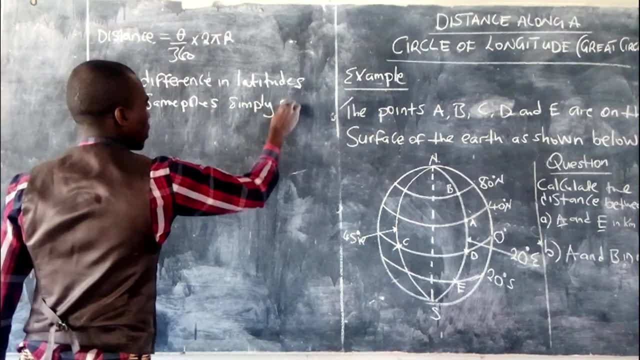 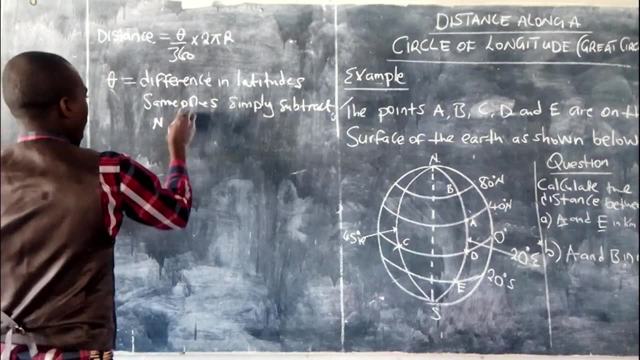 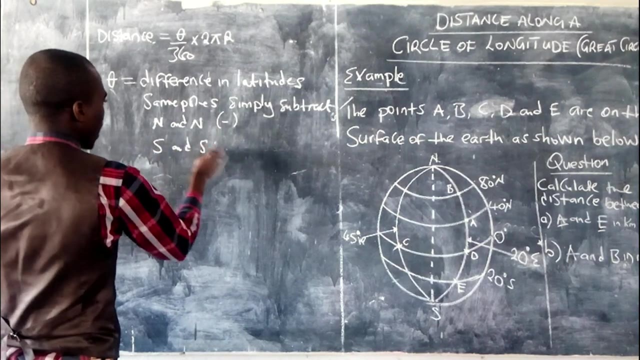 So simply subtract. So, dealing with the same poles, simply subtract. What do I mean? If you have been given north and north, then you are going to subtract. If you have been given south and south, you are simply going to subtract. 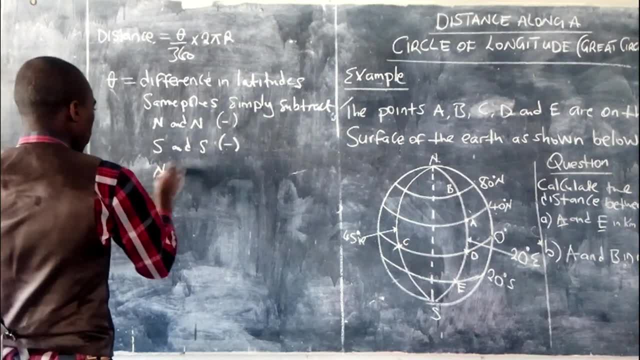 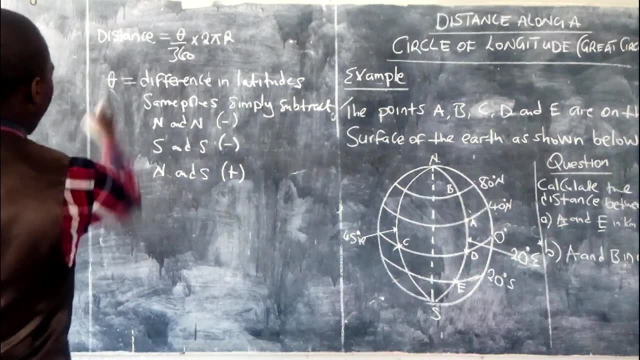 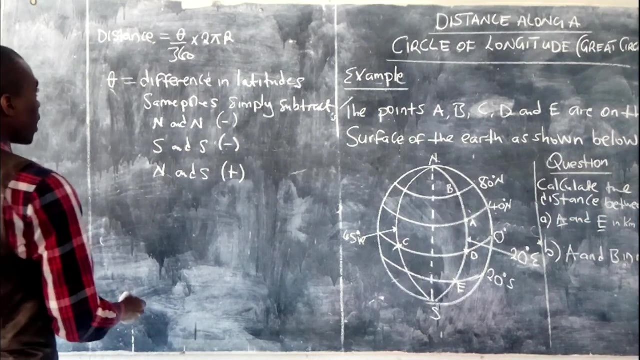 But if you are given a situation like north and south to find the difference in degrees, you are supposed to add. So that is about difference in degrees, as you are going to see in the examples. All right, Then we also have pi. 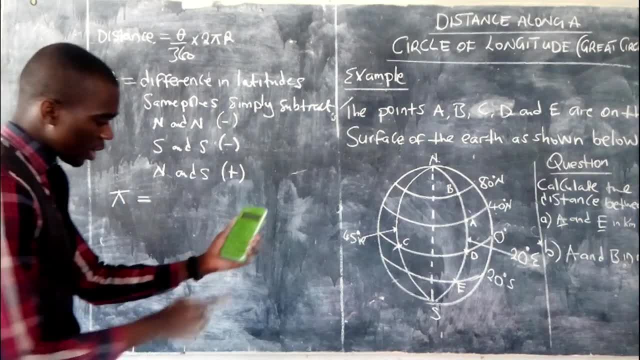 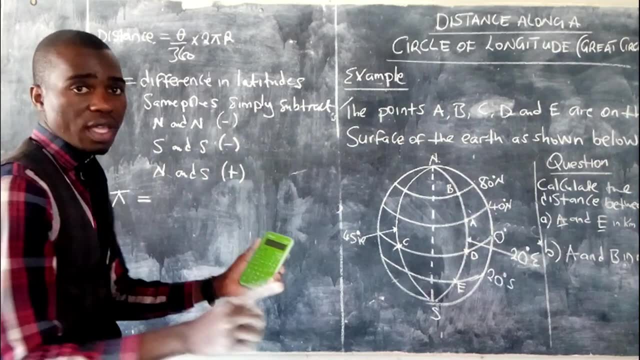 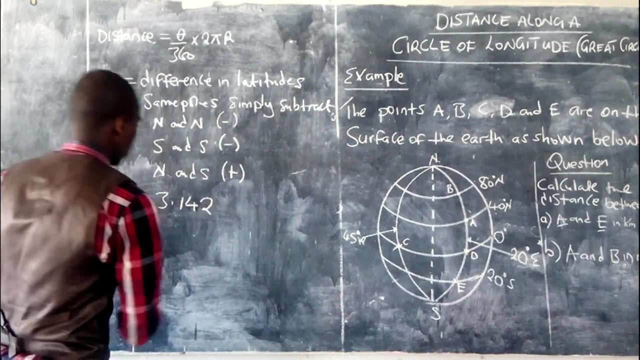 So this value of pi, we have it on the calculator right here. Just press shift and then pxp pi will come. But in the example they are usually going to be giving this value as 3.142.. Okay, Then, lastly, in the formula we have r. 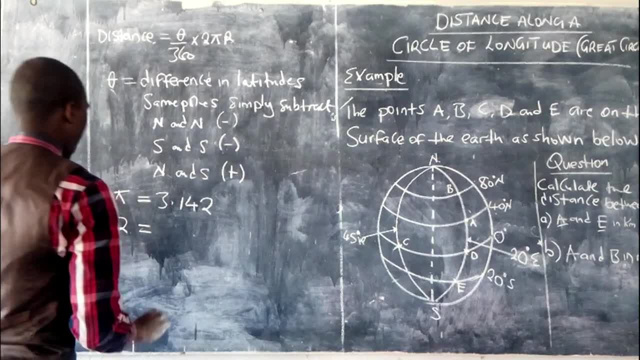 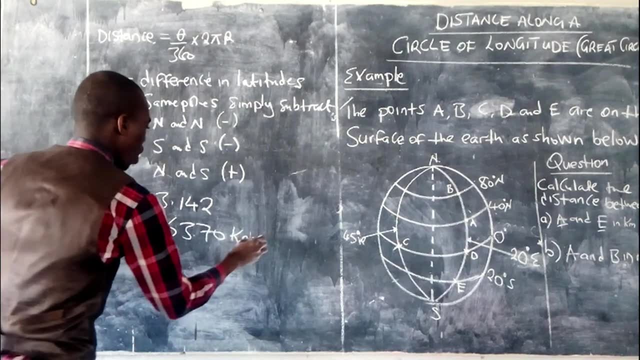 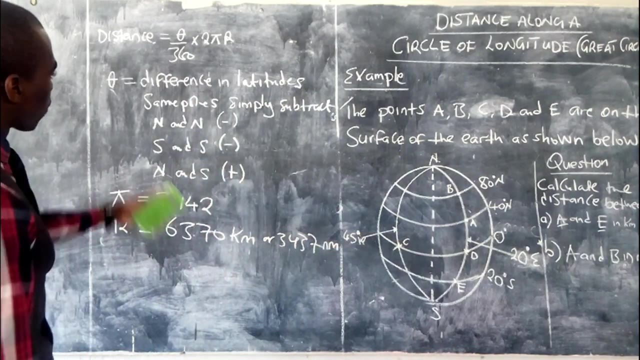 So this r? this is the radius of the x-surface, which is given as 6370 kilometers or 3437 in nautical miles. So we have to know this information for us to successfully solve such a question. All right, 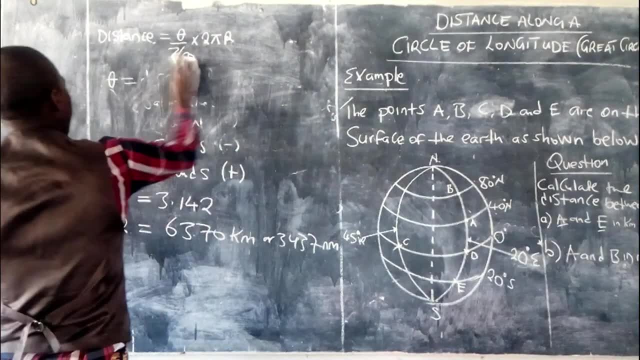 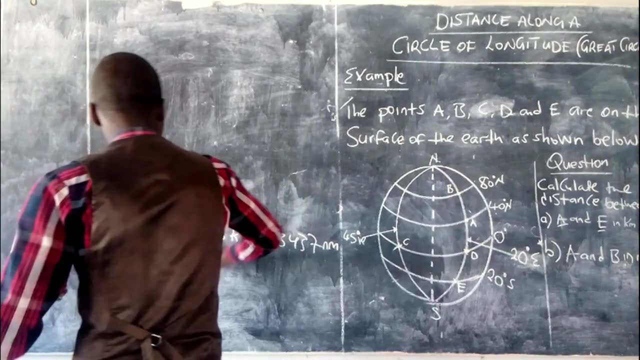 Let's now see how we can apply it. Now, the question that will come is: what is this? The question that will come is in the example. they won't tell you like the way I would like them to say. we are dealing with the circles, the red circles. 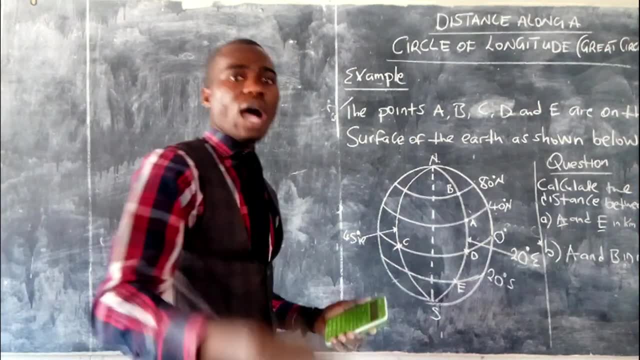 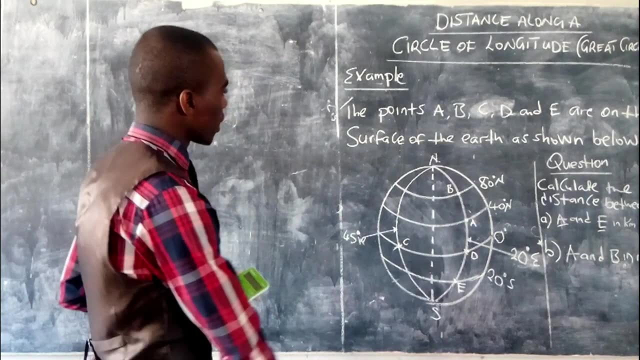 They won't tell you. It will be you to figure out. And how do you figure out? Please follow me. How you figure out is when you collect the data. Data is simply collecting the information that you have been given in the question. 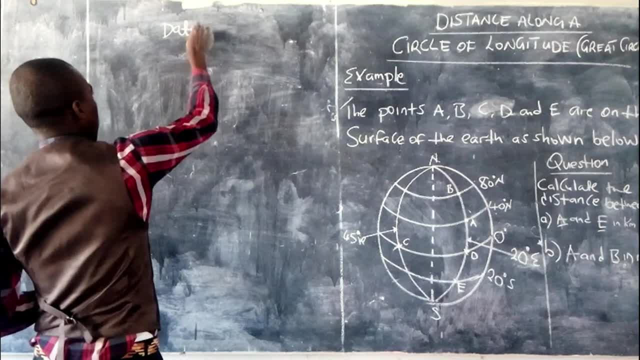 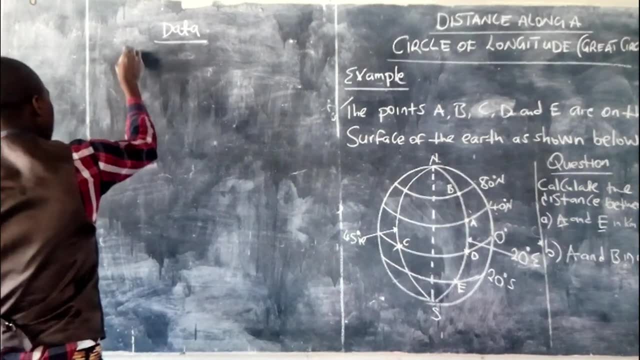 So let's collect the data for a. So here they've told us we are finding distance between a and b, So you have to collect the coordinates for a, The coordinates for a. here we have 40 degrees north, 20 degrees east. 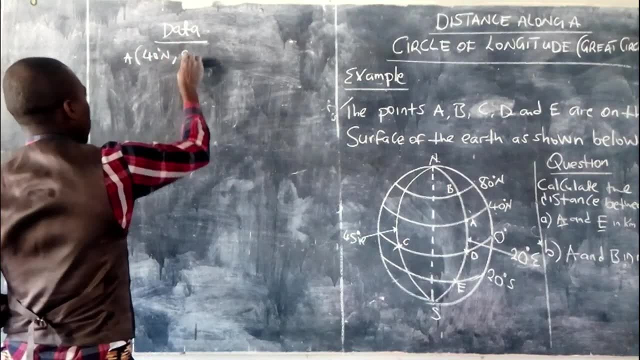 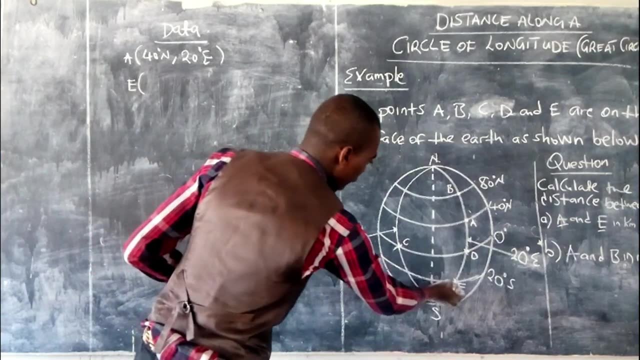 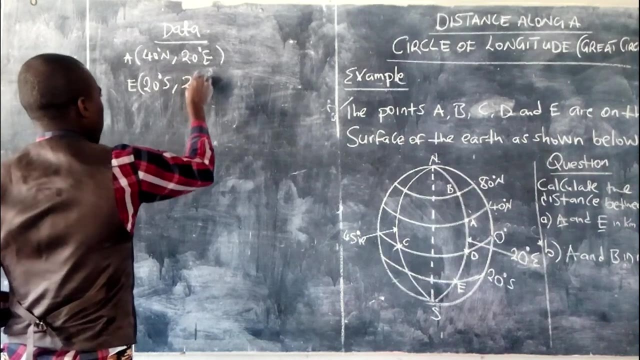 So this is 40 degrees north, 20 degrees east, Okay, And then e we have, so for e we have, this is 20 degrees south, Okay, So 20 degrees south, 20 degrees east. 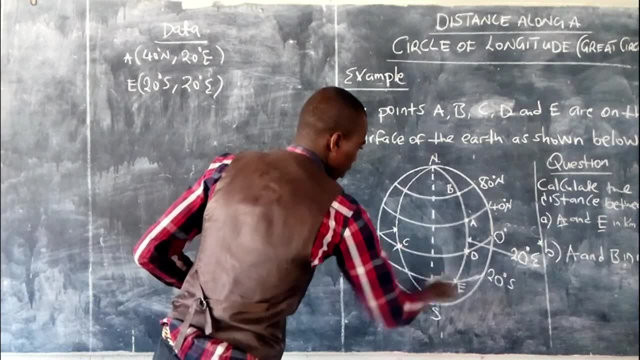 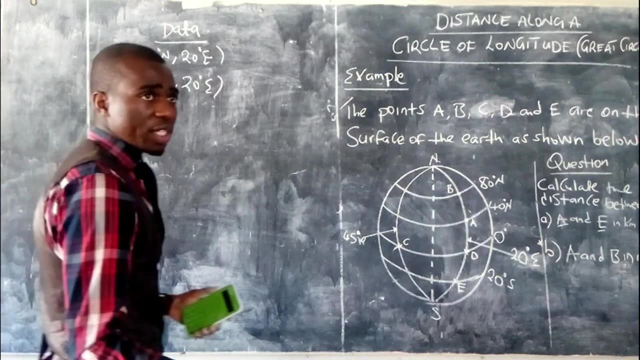 That is what we are having. This one has been labeled for us, And then also that one has been labeled. All right, So we continue Now. I was asking you a question: How do you know that you are dealing with the longitude in the circle of longitude or not? 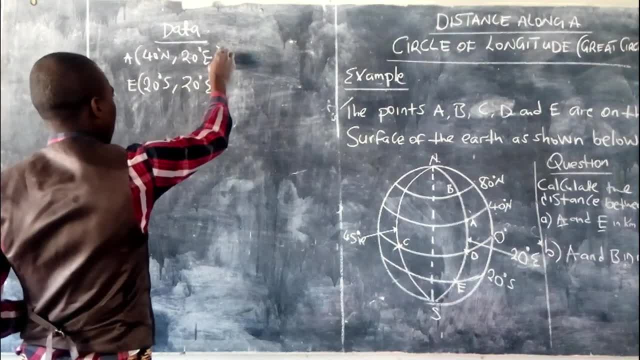 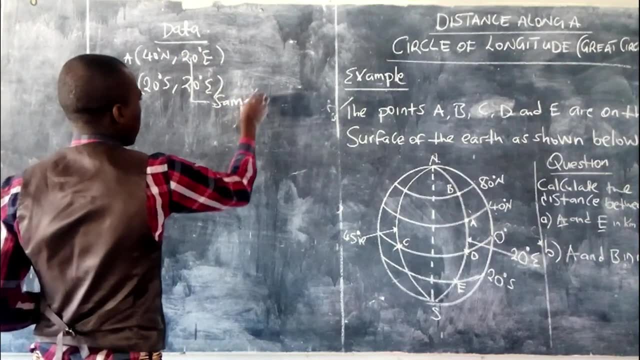 So if you find that in the first letter that we have given you and in the second one the longitudes are the same, Like here, we have the same longitude, So same longitude. So if you are dealing with the same longitude, then you are dealing with what? 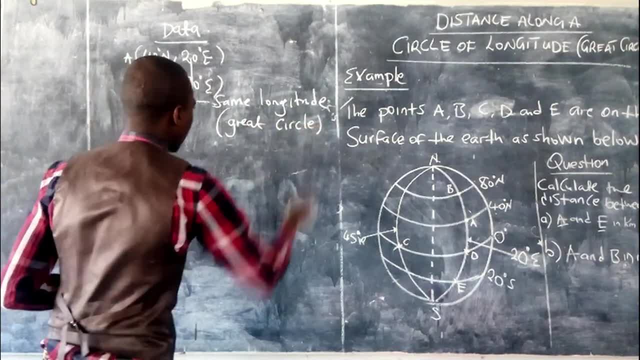 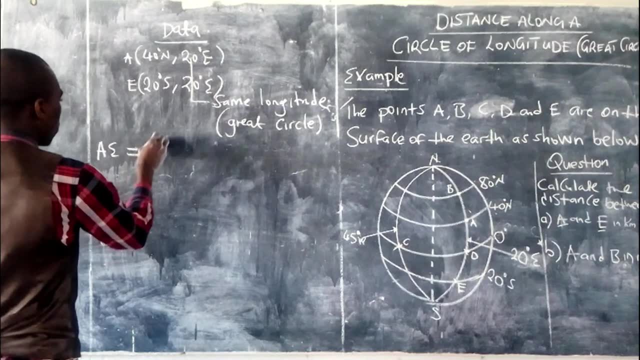 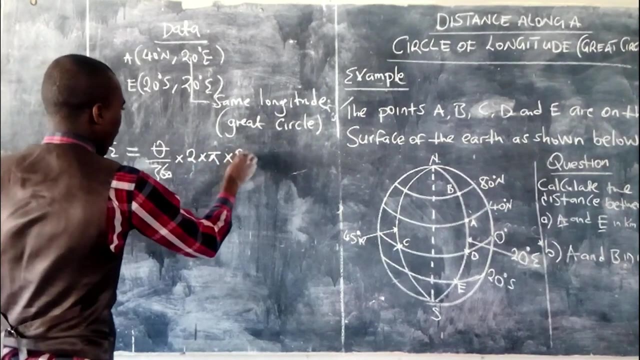 A great circle. Okay, And you are dealing with a great circle, So meaning, automatically, you know that you find a e. the formula to use is theta over 350 multiplied by 2, multiplied by pi, multiplied by r. Okay, So, like we said, this theta here is simply the difference in length. 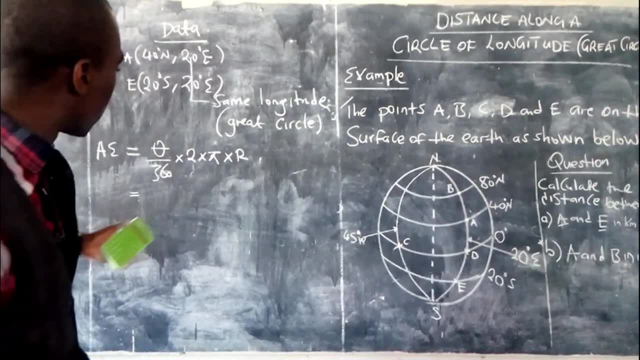 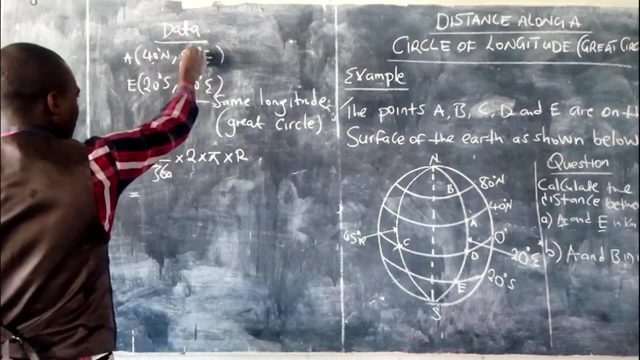 This is simply the difference in degrees. So, since it is the difference in degrees, we are now going to subtract these ones here. These ones are the same. You can't subtract any of these. They are just there to help you identify what you are dealing with. 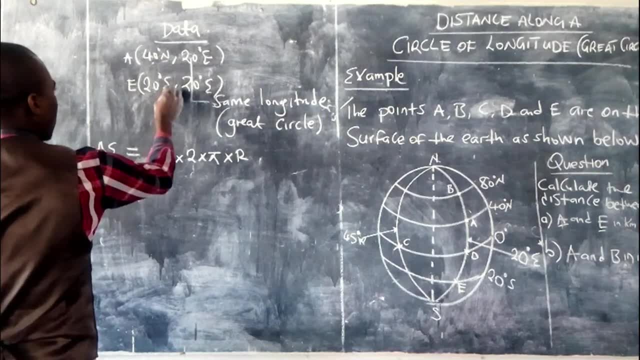 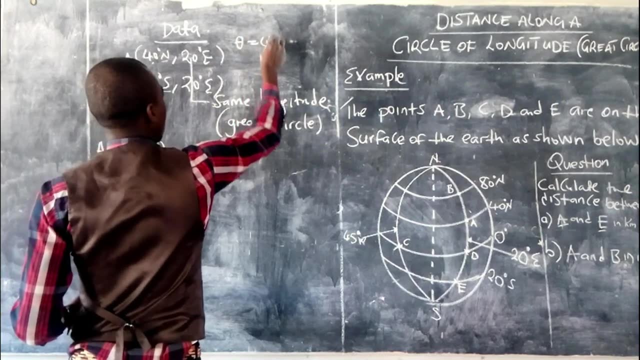 Okay, Then this and this. Like we said, the signs here are different, Meaning, in fact, the difference in degrees there we are simply going to add. So difference in degrees, theta is equal to 40 plus 20.. And this one is going to give us 60 degrees. 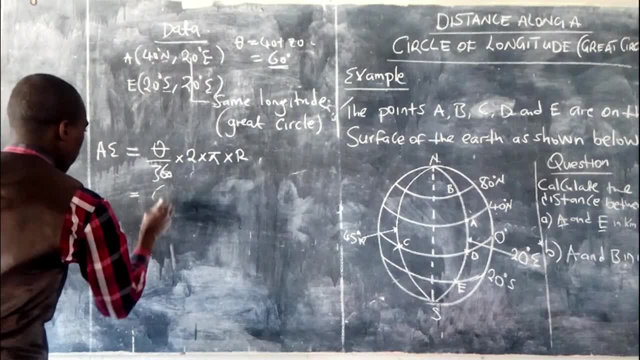 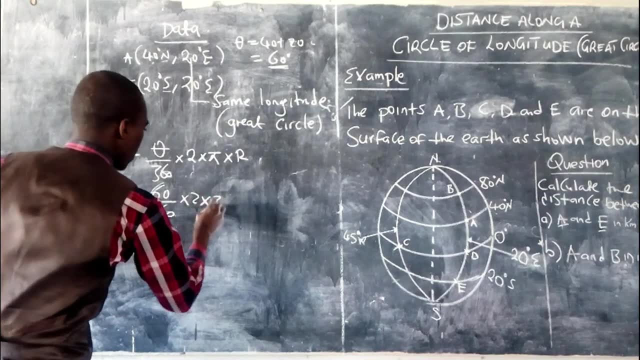 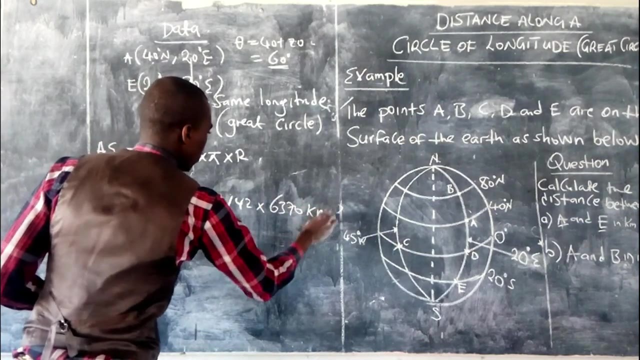 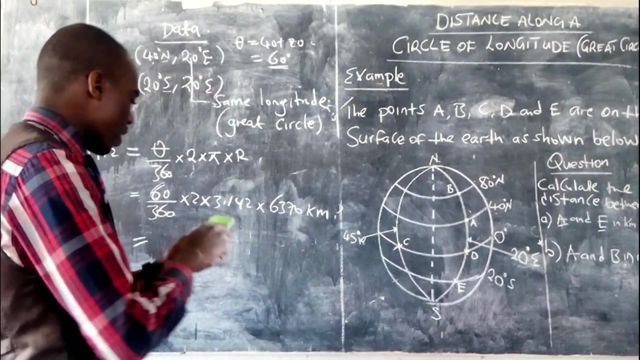 This one is 60 degrees. So this one will be 60 degrees divided by 350, multiplied by 2, multiplied by 3.142, multiplied by 6370 kilo meters. All right, So we continue there. We can punch on the calculator and see what value we are going to get. 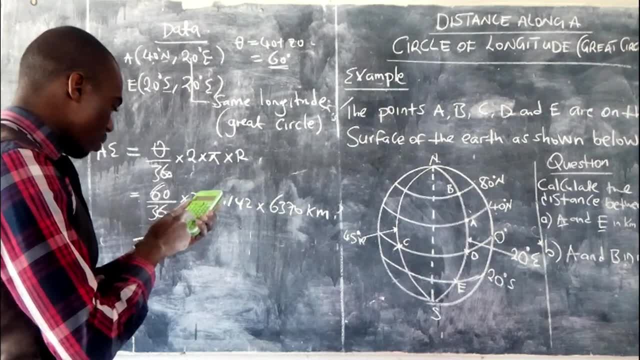 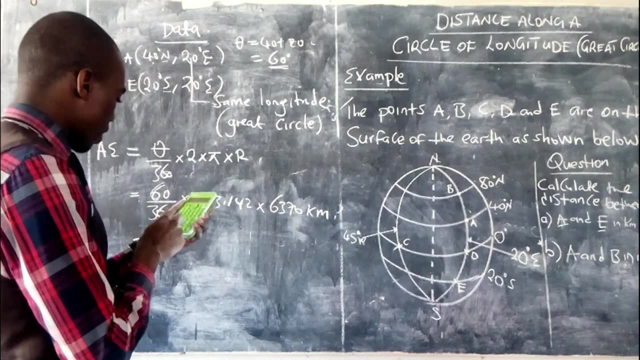 So we are saying 60 over 350 multiplied by 3.142.. And 60 multiplied by 2, multiplied by 3.142, multiplied by 6370.. And this one is giving us. So first of all you have to write the full value. 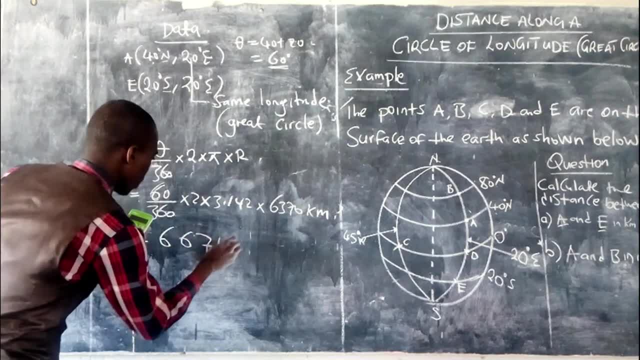 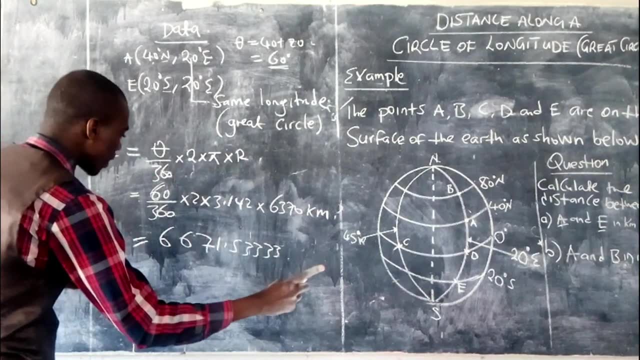 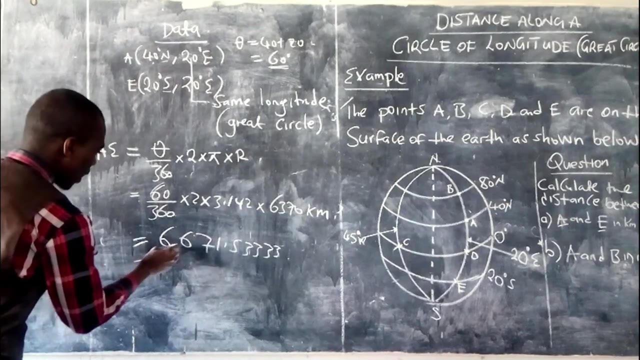 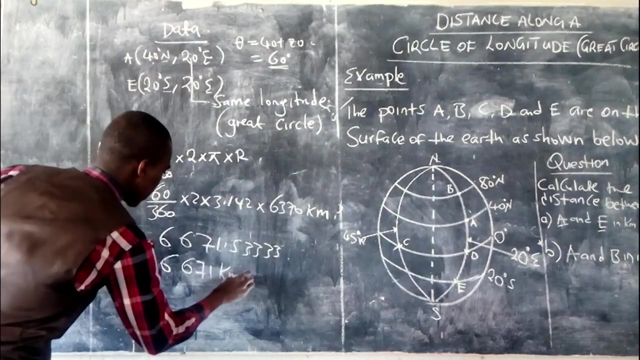 6671.53333.. And now you can write this one to either one decimal place or to four significant figures. Okay, So if your writing is to three stars, If your writing is to three stars, If your significant figures are one, two, three, four, then it is going to be 6671 kilo meters. 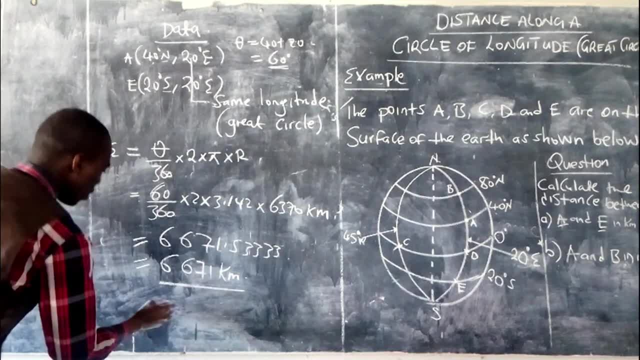 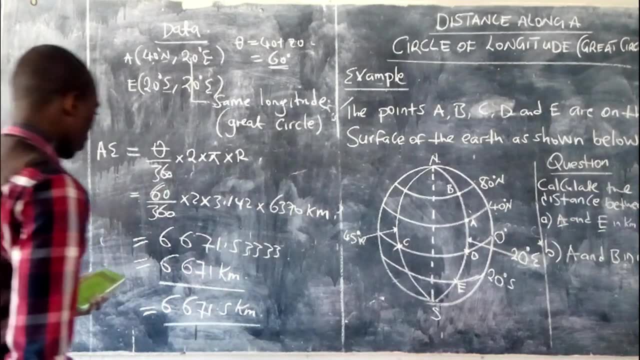 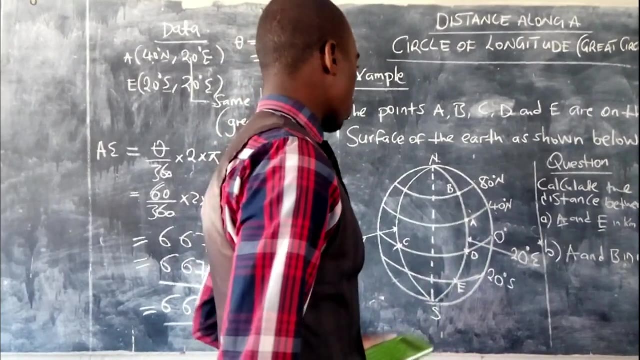 Or if you are writing it to one decimal place, it is also allowed. It will be 6671.5 kilo meters. All right, So that is how you solve question A. Okay, Let us see if we can now also solve question B, Okay. 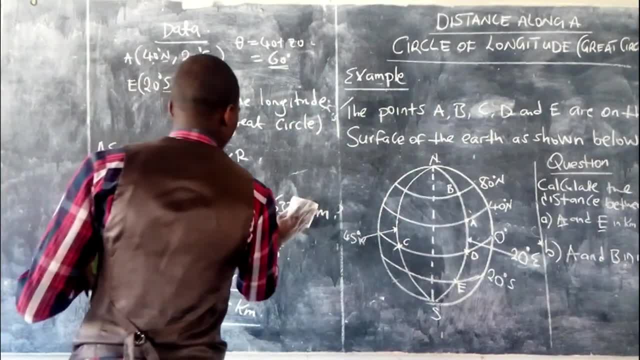 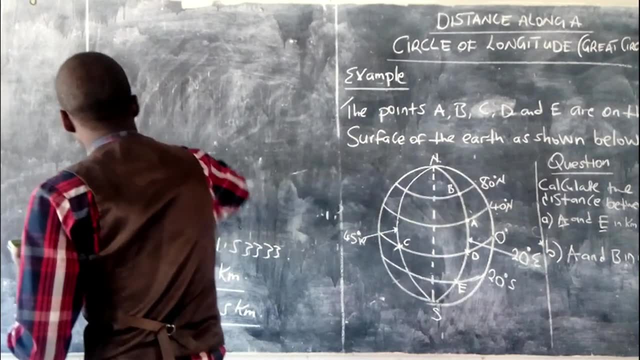 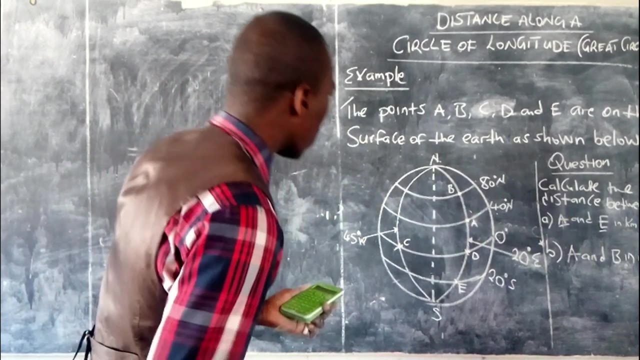 So in question B, let us collect the data as well. Now, in question B, we are finding the distance between A and B, And this one should be in nautical mass. Okay, So, collecting the data, we have our A here, which is 40.. 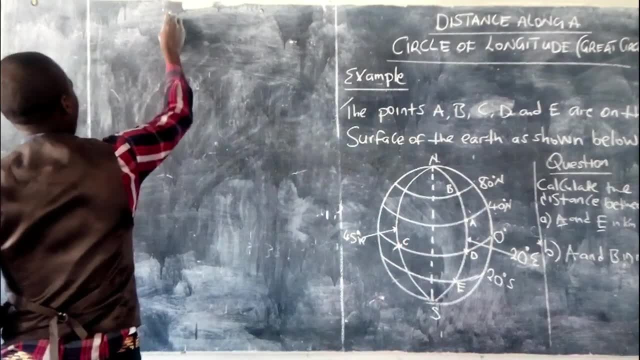 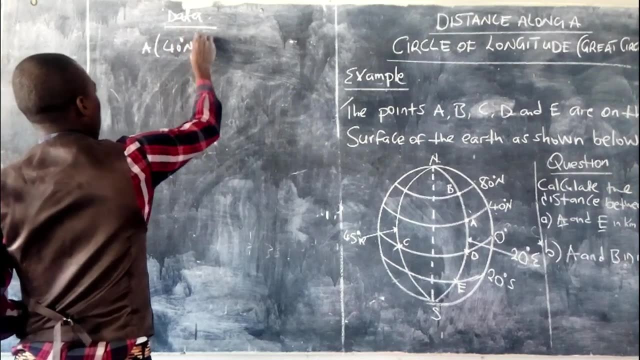 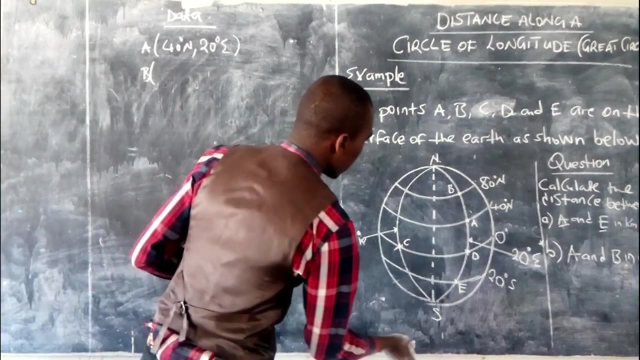 Okay, So 40 degrees north or 20 degrees east. So data there. We are going to have our A as 40. So our A as 40 degrees north, 20 degrees east. Then our B we have. so let us check B: B is 80 degrees north. 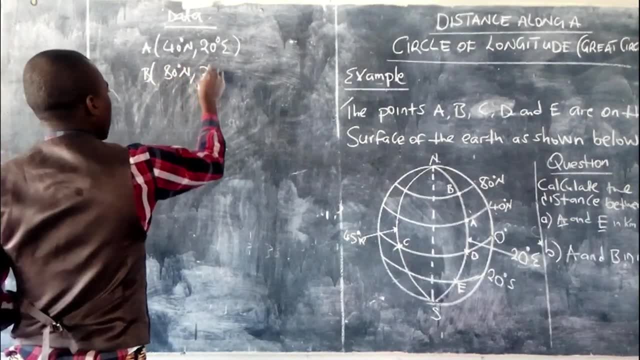 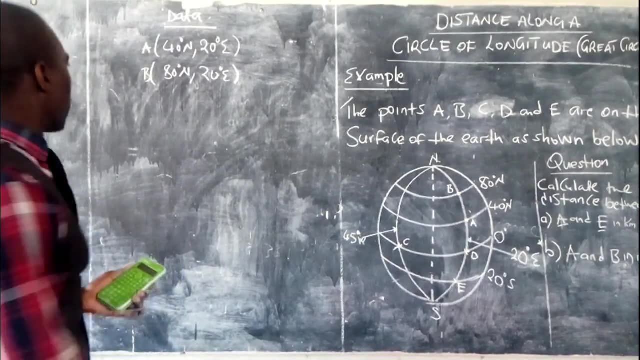 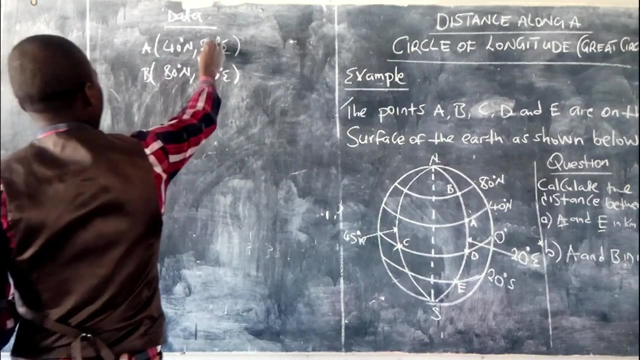 So this is 80 degrees north, 20 degrees east. So that is what we have. So again here in the exam you have a choice to make. Is this the great circle or a small circle? But here you can see the longitudes are the same. 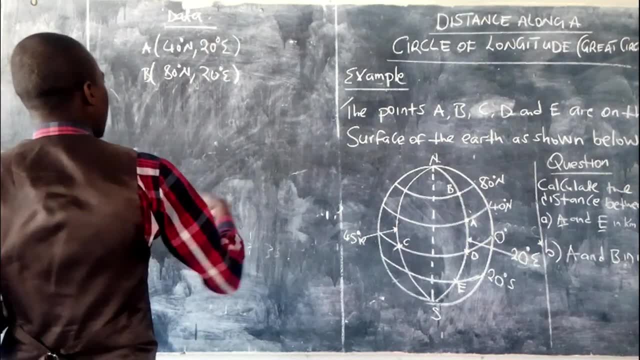 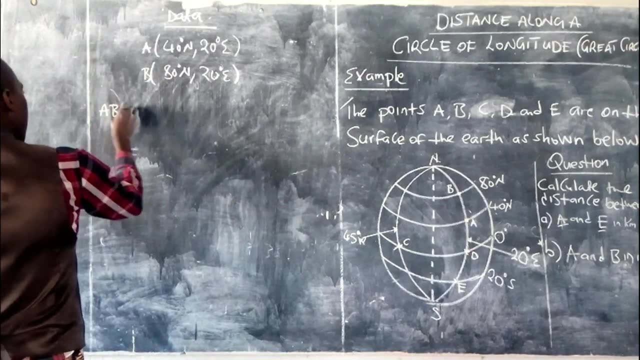 So since the longitudes are the same, then you know that you are taking the distance along the circle of longitude, which is also called the great circle. So the formula to use is: FBE is equal to theta divided by 360, multiplied by 2 multiplied. 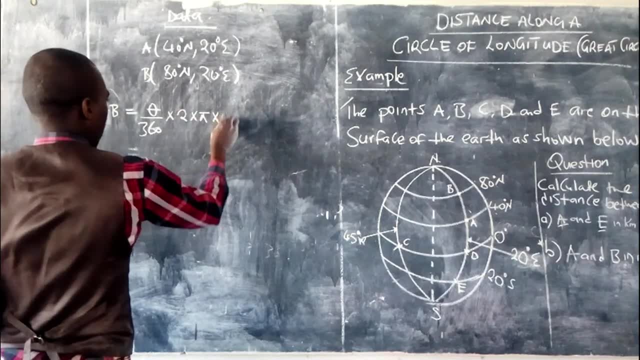 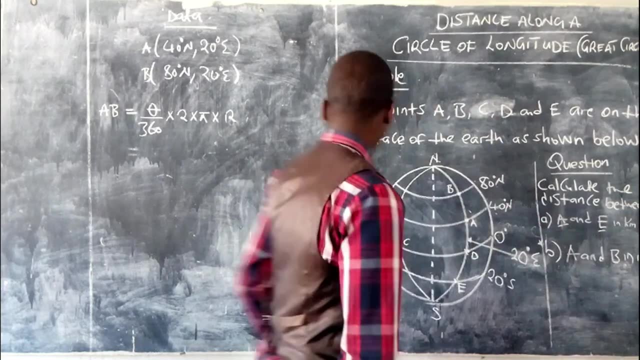 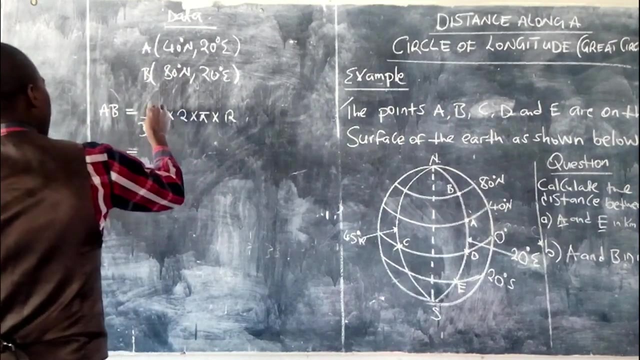 by 5 multiplied by so R. Okay, Now this one. let us say we are finding in nautical mass. So when we are finding in nautical mass, let us substitute here theta. Look at. so the theta we say is the difference in latitudes. 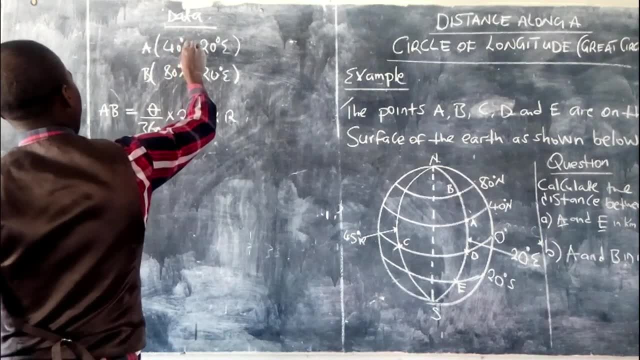 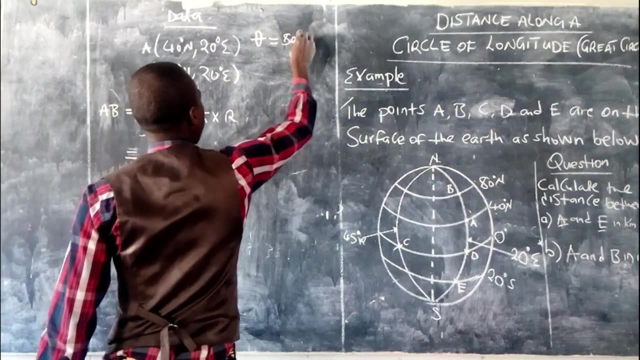 And this latitude here we have. they have the same sign: north, north, the same force. So since it is going north to find that theta there, we are simply going to say 80 minus 40. Okay, 80 minus 40, which is giving us 40 degrees. 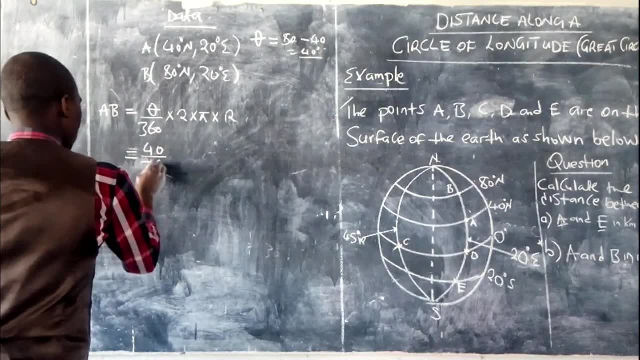 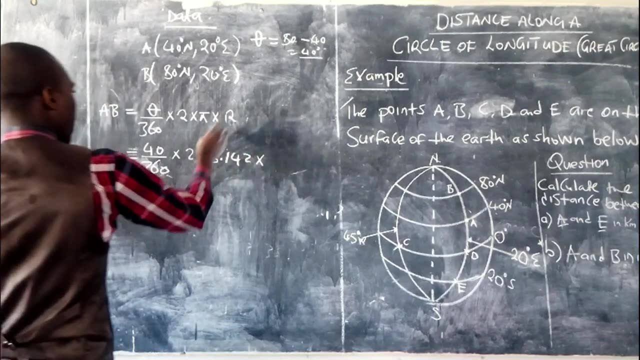 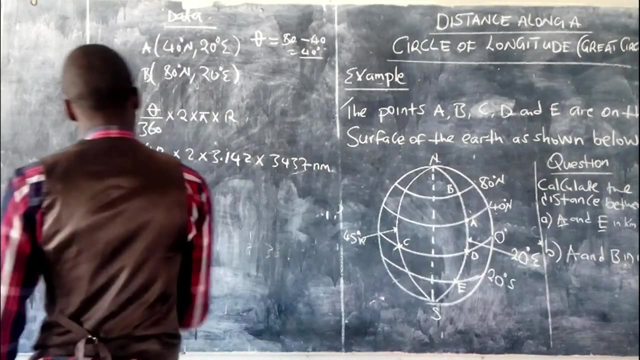 So this one is going to be 40.. 40 divided by 360, multiplied by 2, multiplied by 3.142, multiplied by R- Now R because it is nautical mass- we are going to have 34, 37 nautical mass. 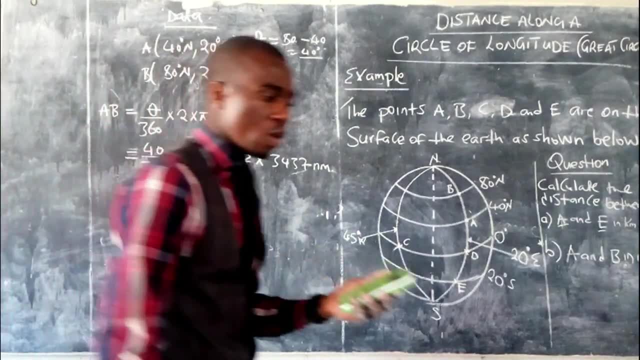 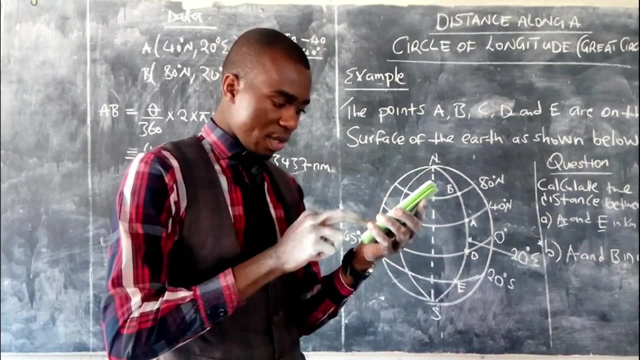 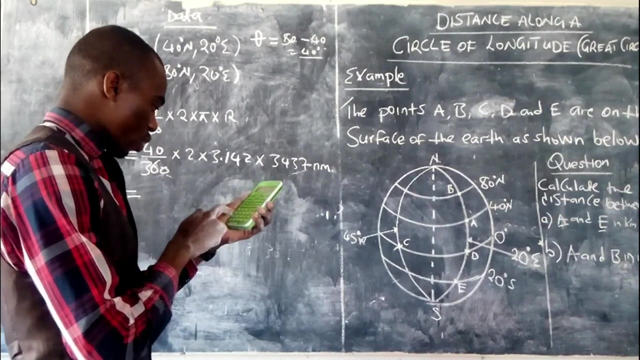 So let us punch that one on the calculator and see what value we are getting. All right, So that one is 40 over 360 multiplied by 3.142.. Multiplied by 3.142, multiplied by 34,, 37 nautical mass. 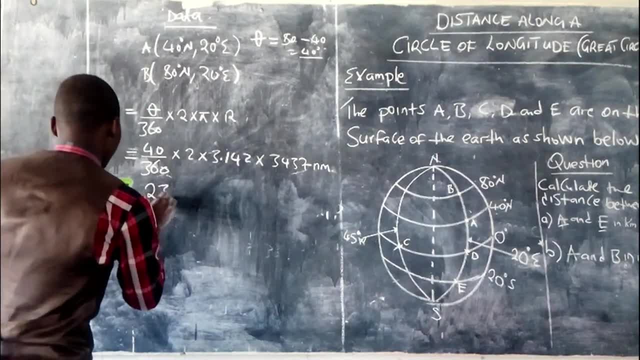 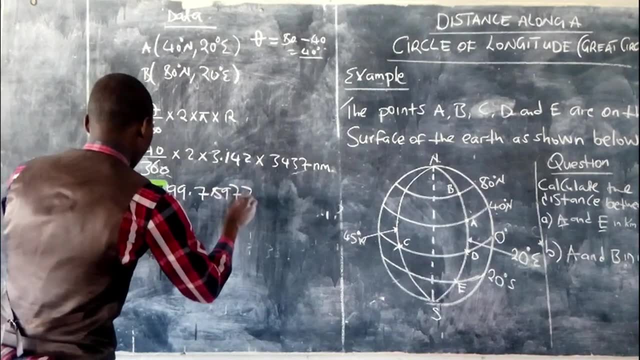 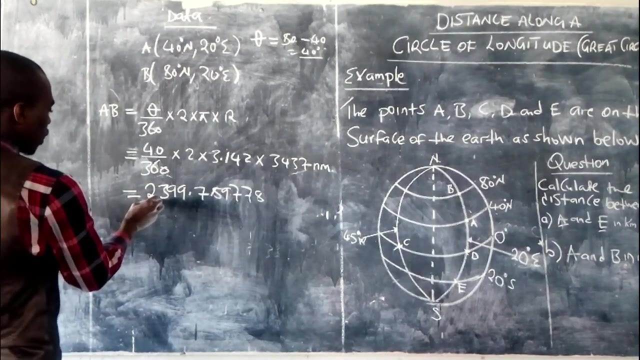 And this is the value we are having: 2399.789778.. So we can round off this one now to 4.. If we are rounding this one to 4, significantly, it gives us 1,, 2,, 3,, 4.. 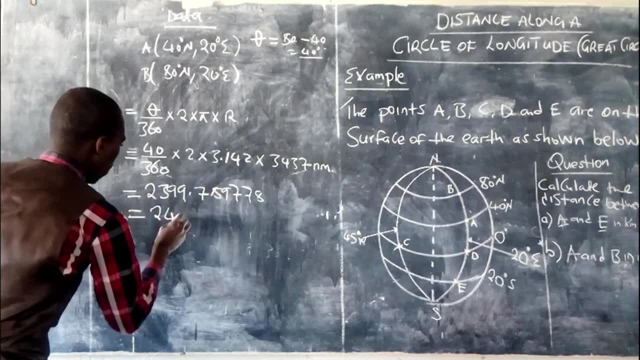 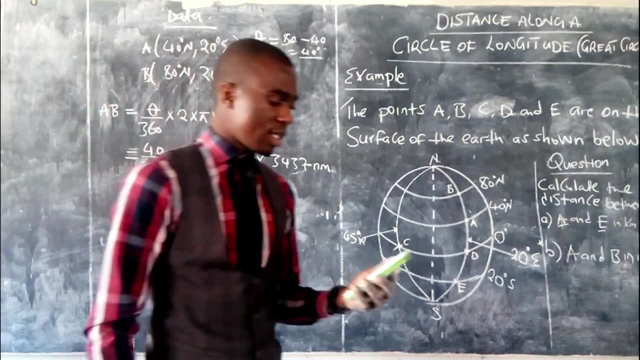 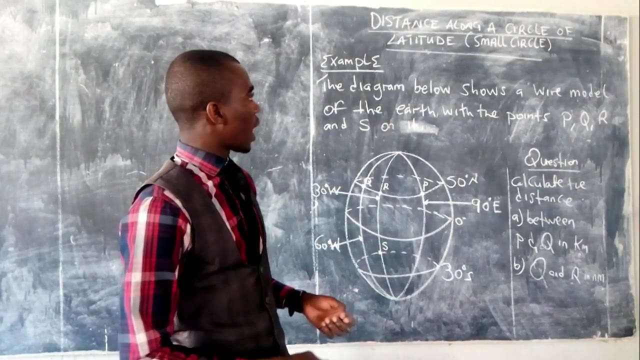 And the value we are going to have is 24 hundredi nautical mass. So that is our answer And the question has been sorted out. Okay, So now we look at distance along a circle of latitude. Now, distance along a circle of latitude. 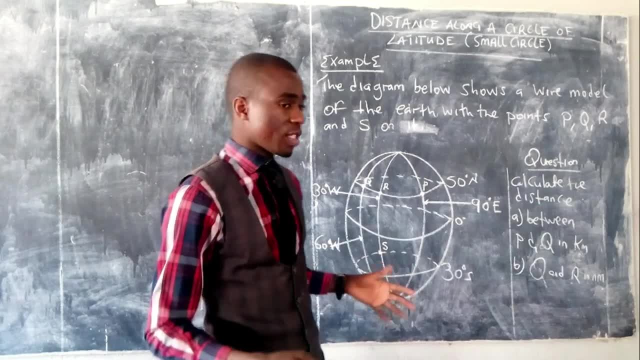 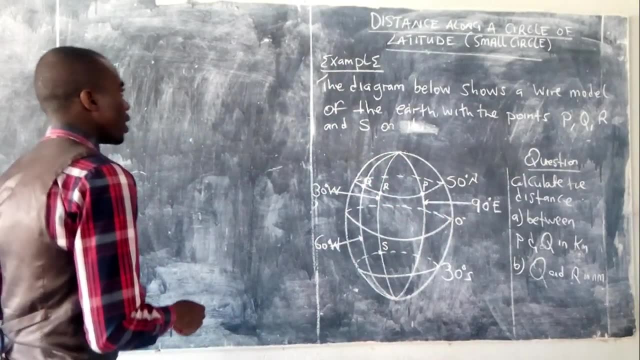 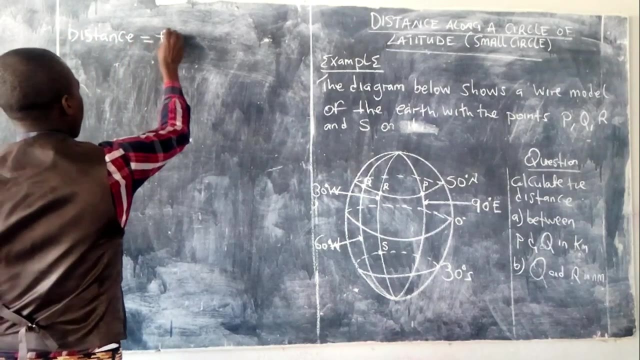 So a circle of latitude is also known as a small circle. So we want to now see how we can calculate that Distance along a small circle. So here the formula now becomes distance. distance is equal to theta over 350 multiplied. 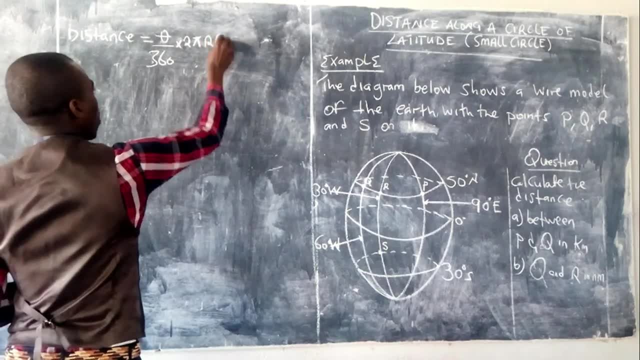 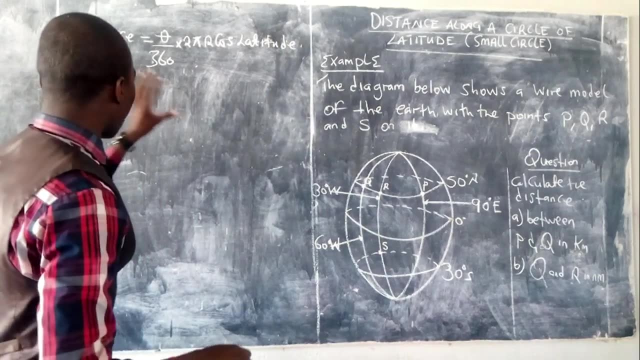 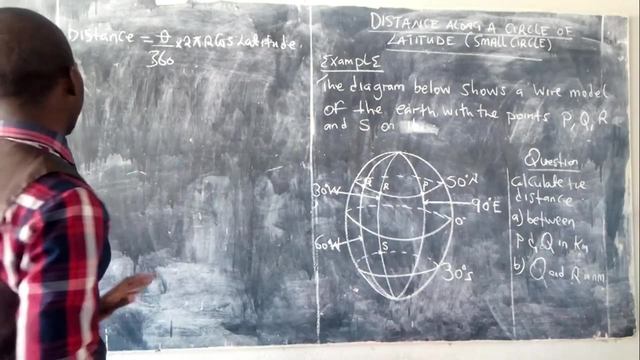 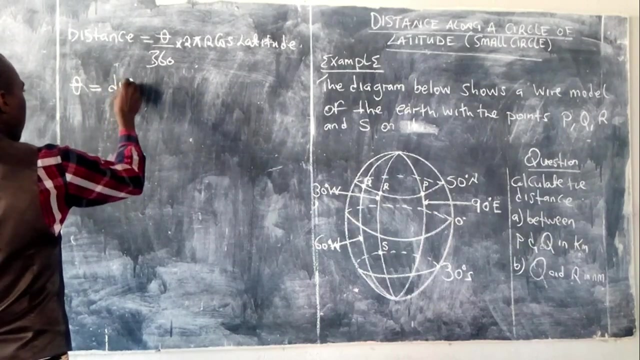 by 2 pi r, then cos latitude. Okay, So this is a simplified way in which the formula can be expressed. Other books will express it in different ways, But this is the best way I can express it now. But now you know that theta in this distance will mean difference in longitudes. 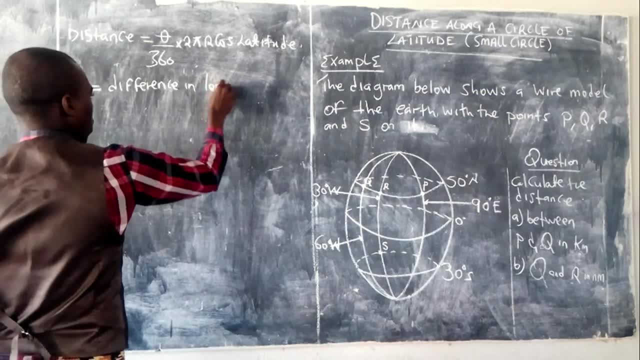 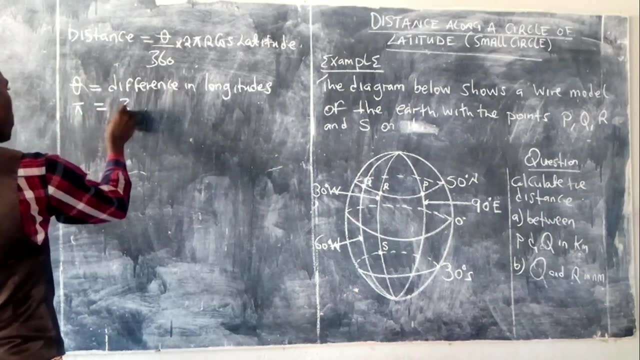 So it will mean difference in longitudes. Okay, So difference in longitudes. Then pi: right now, you know that in books they will be giving us the value of 3.142.. Then r here: r, that is the radius. 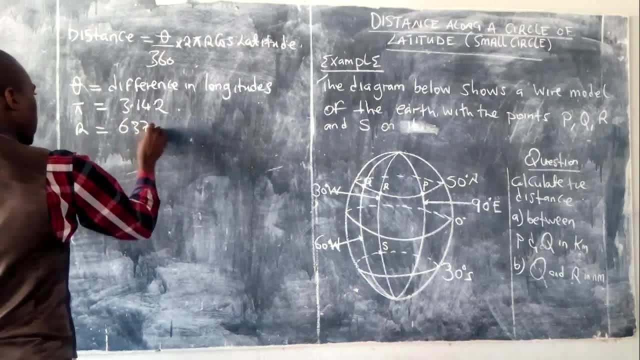 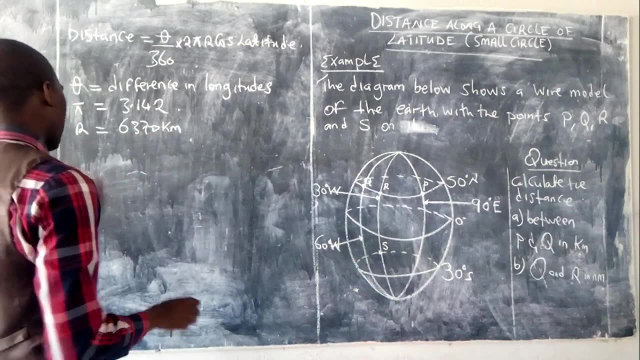 On the edge surface, which is 63, 70 kilometers. So, please, when you are being taught to find distance in kilometers, this is the value to use for r, But when you are being given, when you are being taught to find nautical miles, the value 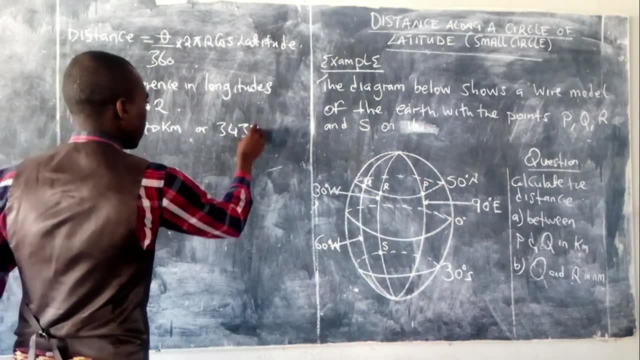 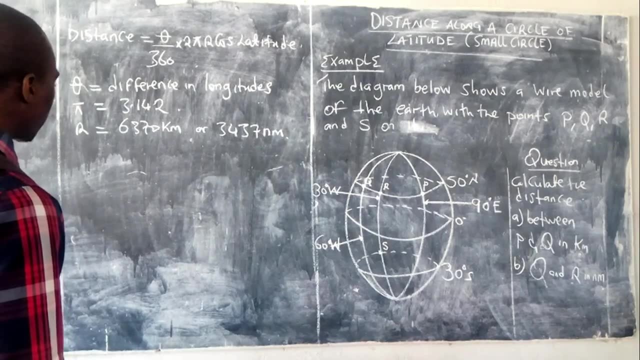 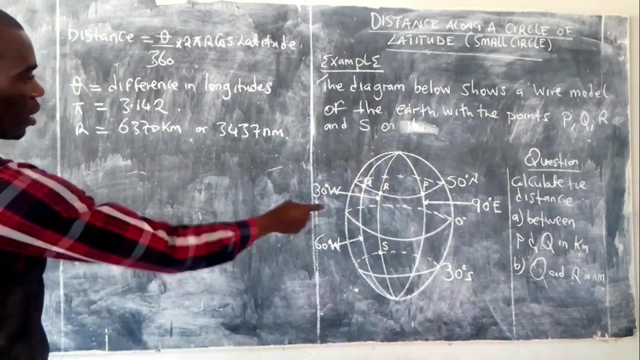 for r to use is 34, 37 nautical miles. Alright, So this is what you are supposed to do. I think to know about the formula. So now, solving the question that we have been given here, let's first of all collect. 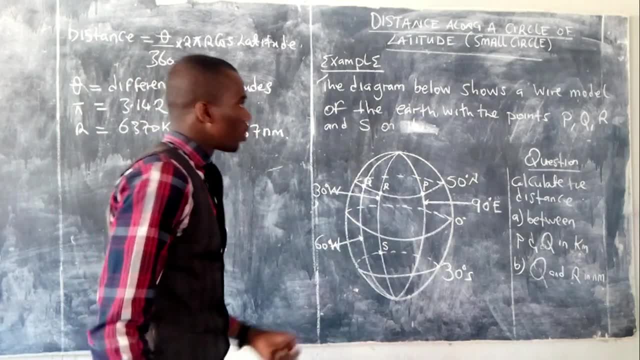 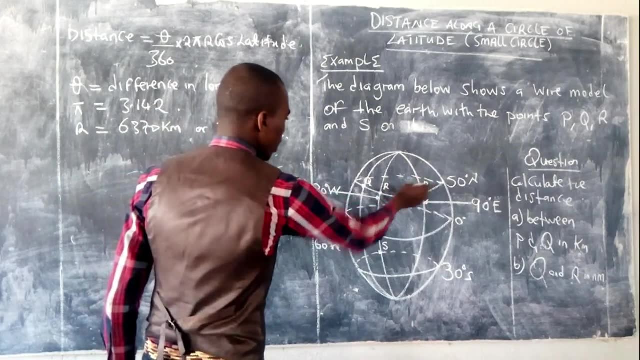 the data. for the first one, The example reads: the diagram below shows the wire model of the earth with the points p, q, r and s. So we have p, q, r and s okay, which are marked on it. 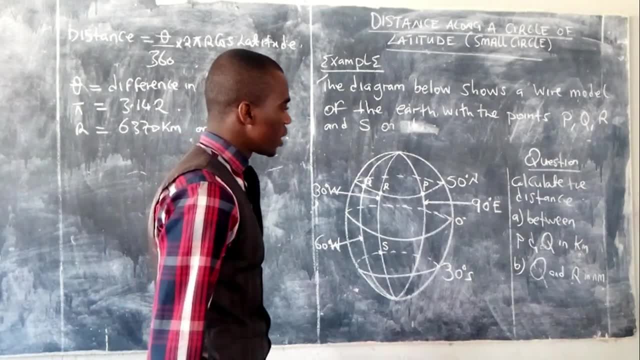 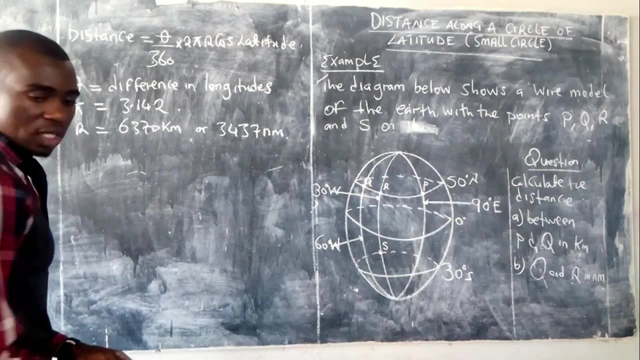 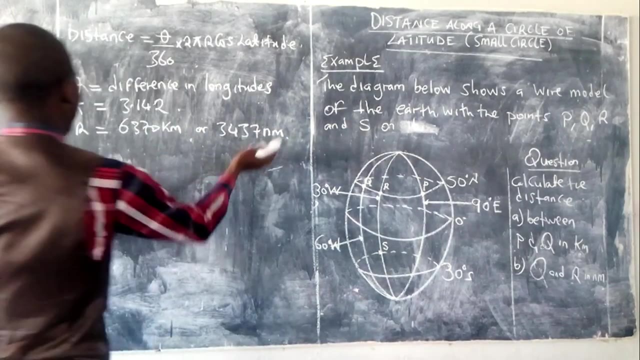 The equation reads: calculate the distance between p and q in kilometers. So a we are finding the distance p and q in kilometers, Alright, So we can get rid of this one. Then we now write the data. So first thing to do is to collect the data. 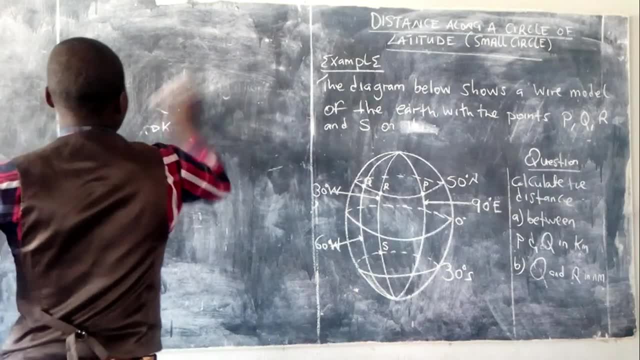 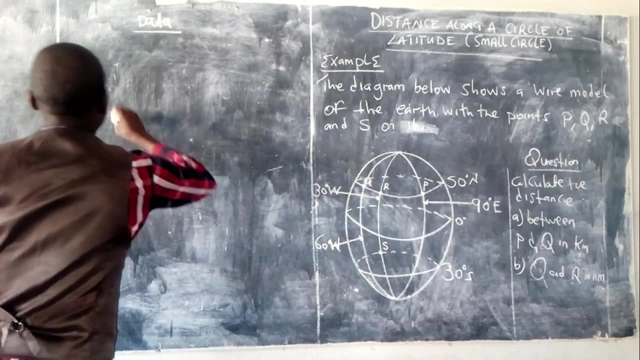 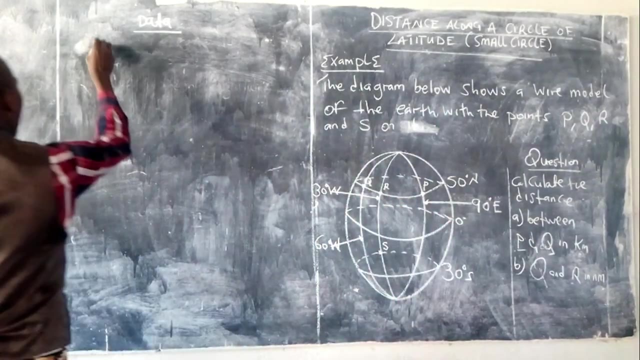 So let's collect the data in solving that question. So we collect the data. This one b Data for a. We know that a for the first one, since they are saying between Between p and q. So we are going to write the coordinates for p. 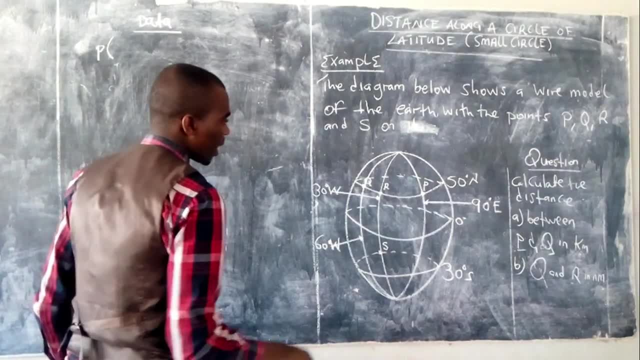 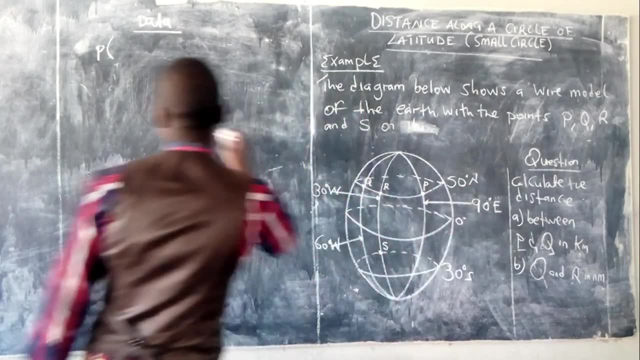 That's the first thing we do. So the coordinates for p here. p is here, The latitude is 50 degrees north and then the longitude is 90 degrees east. So we have to 50 degrees north, 90 degrees east. 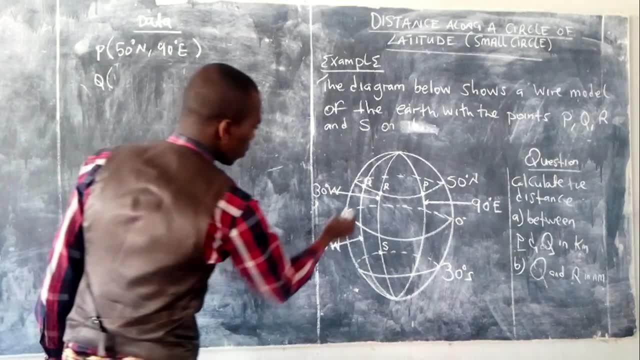 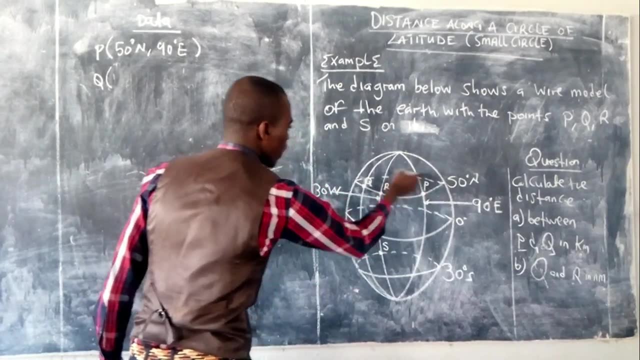 Then for q, let's write for q. q is here. This is also 50 degrees north. Remember this thing: they call a distance. If this is in front, then this dotted line is behind, So we can decide if it is to be the same latitude, which is 50.. 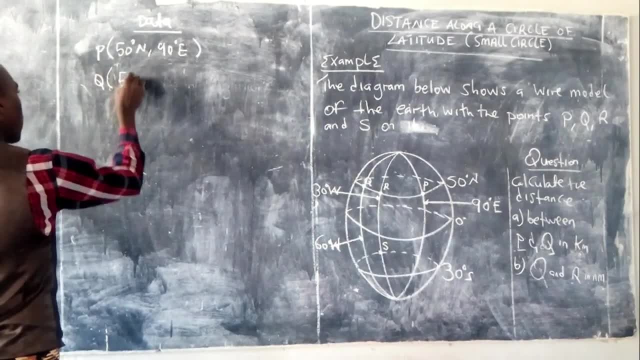 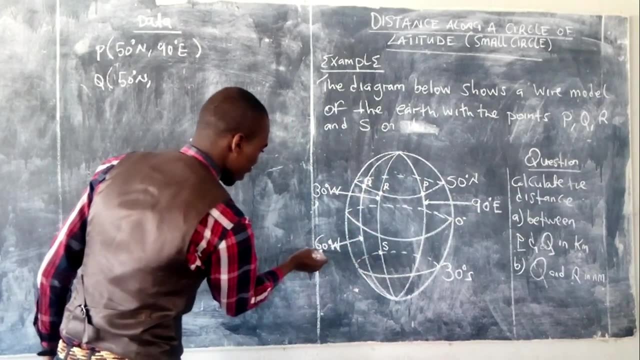 So this one is 50 degrees north, 50 degrees north, comma. Then we check the longitude here, where q is, We check the longitude and we mark it to be 60 degrees west. So, comma, 60 degrees, what? 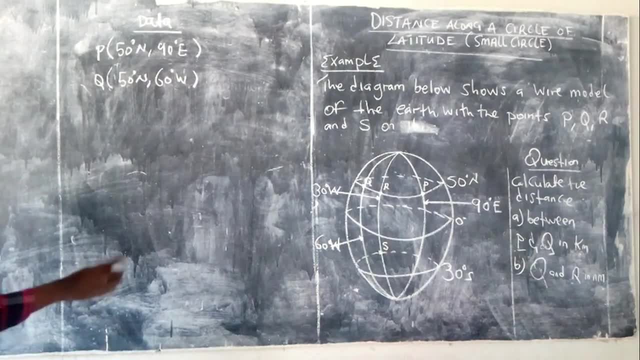 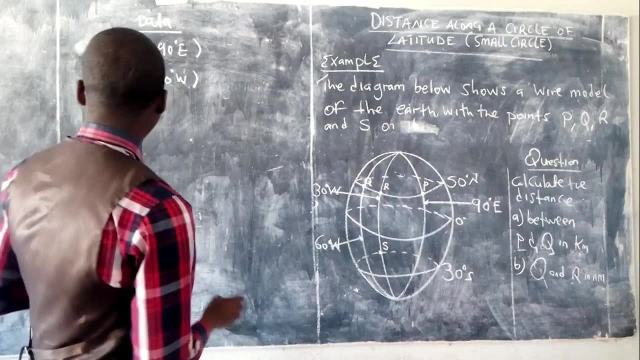 West. Alright, So now how do we identify whether it's a distance, along a latitude, or along a longitude? It's very simple. So here we will check, Since the latitudes here are the ones that are the same. So latitudes are the same. 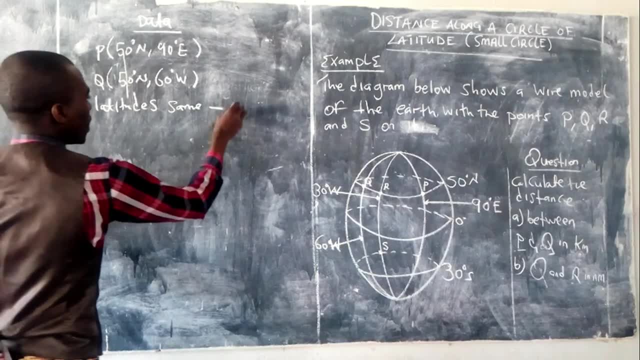 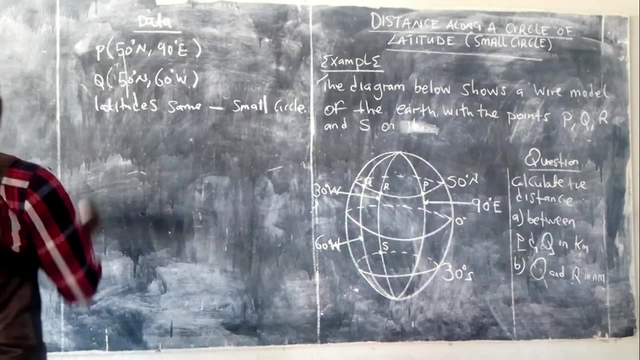 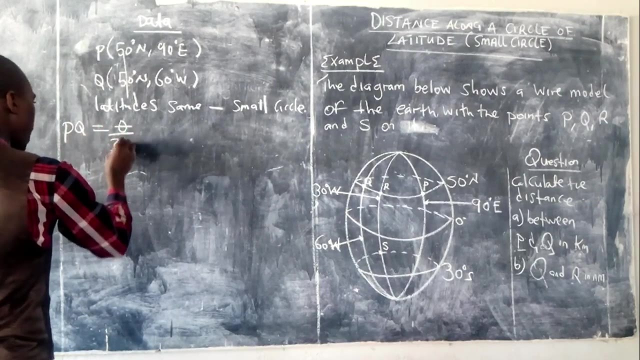 So if latitudes are same, it means you are dealing with a small circle. So you are dealing with a small circle, And if you are dealing with a small circle, then the distance in this distance would be: pq is equal to theta over 350 multiplied by 2, multiplied by. 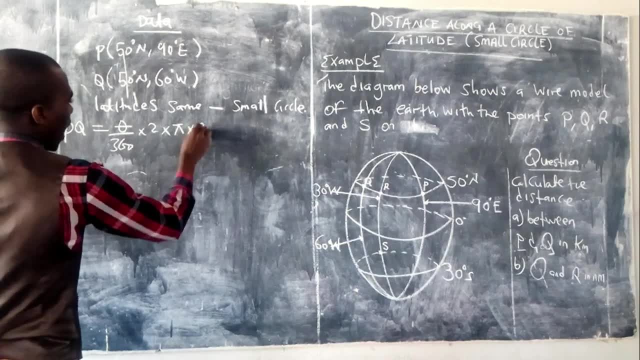 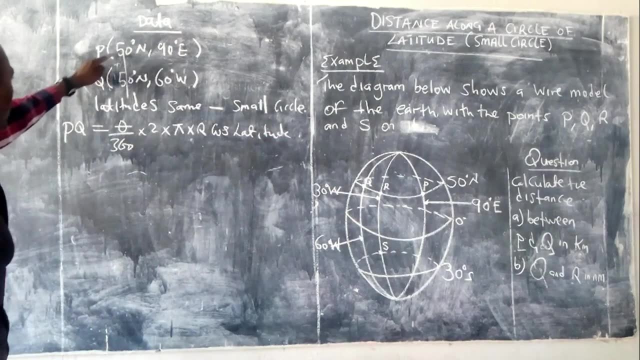 So this is multiplied by pi, multiplied by r. then cos latitude? Okay, Cos latitude? Why latitude? Now, the latitudes are the same. So whether you get for p or for q, it's the same field. So that's what we mean there. 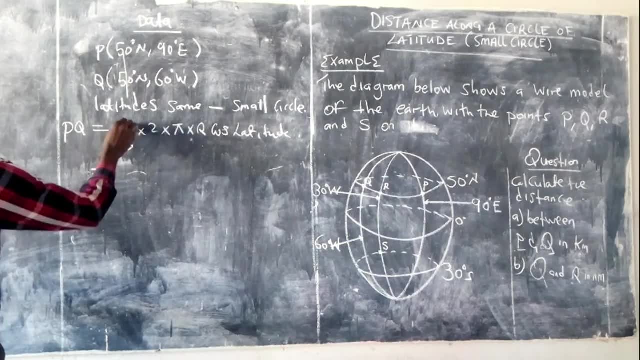 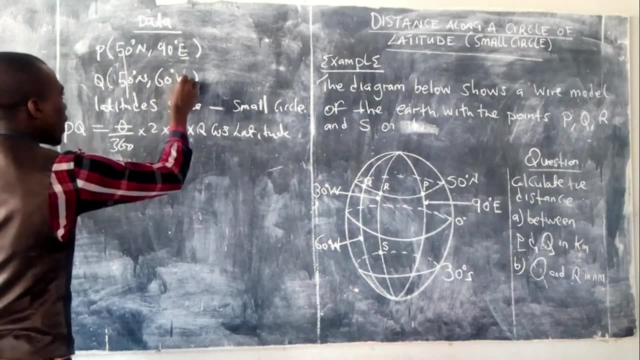 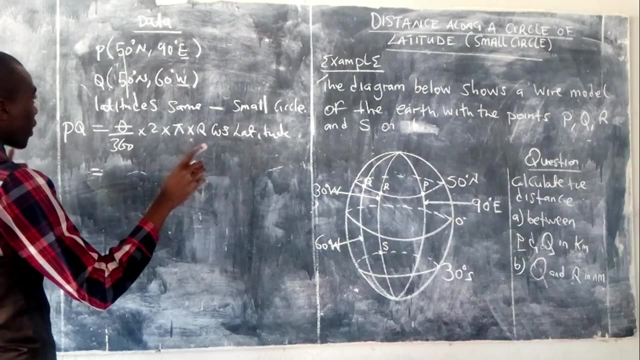 So we substitute this one equal to our theta here to be difference in the longitude. So difference in longitude because we have east and west, we are simply going to add longitude, Because this is different force. we simply do what Add to find the difference. 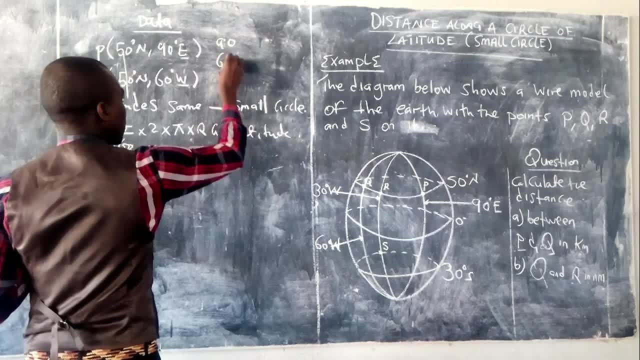 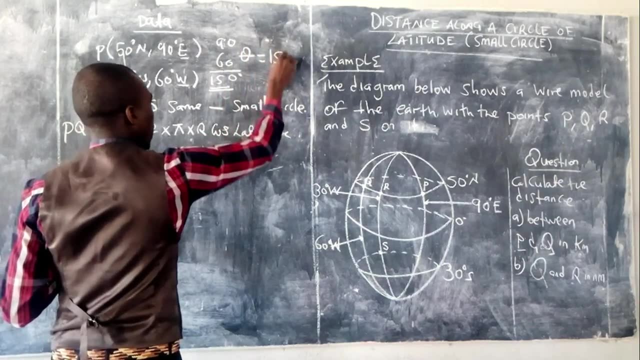 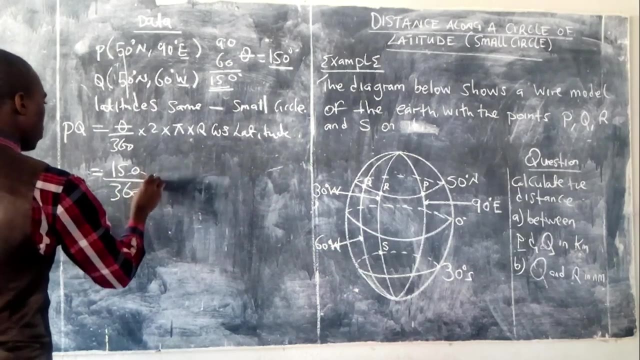 So it will be 90 plus east. So this one is 90 plus east, which is giving us 150 degrees. So that is our theta. We know now it's 150 degrees. So we have 150 divided by 360, multiplied by 2, multiplied by 3.142, multiplied by. 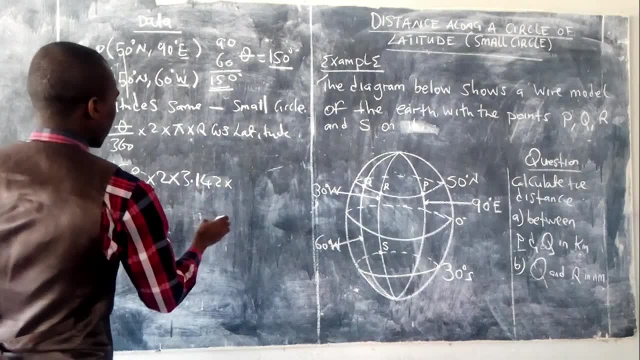 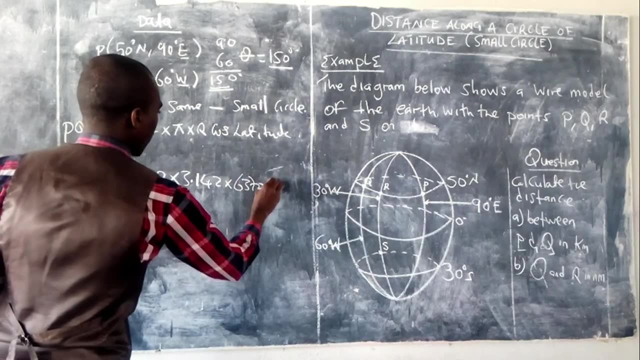 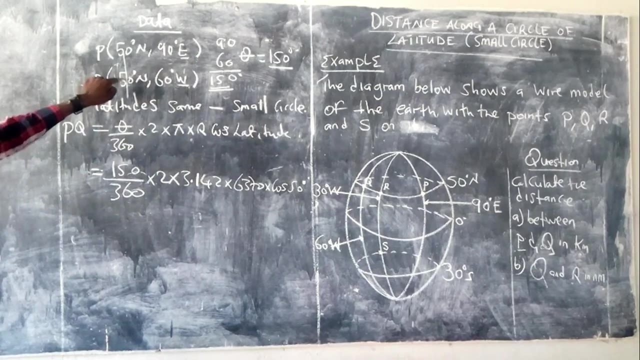 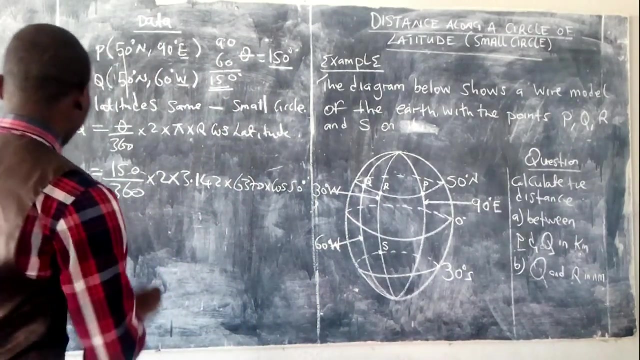 Our r here. our r it's in kilometers, So we use 63,, 70 kilometers multiplied by cos- 50 degrees, because it is cos latitude which is this one. So we substitute, Then now we can get. we can punch that one on our calculator and see what value it is. 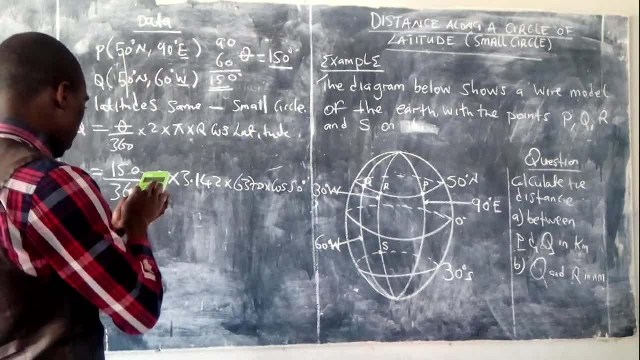 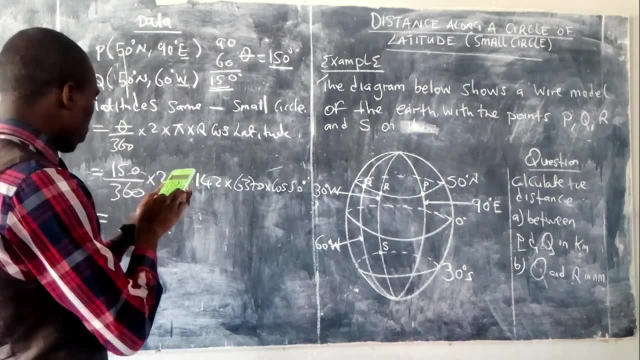 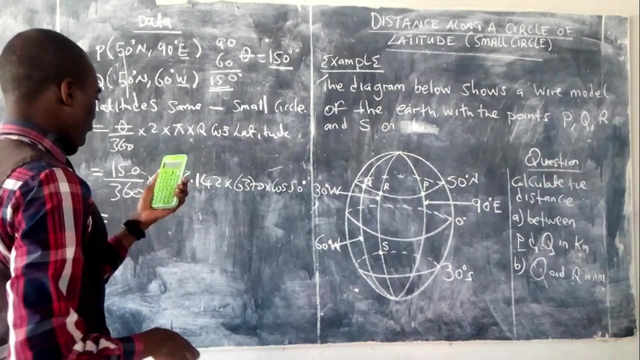 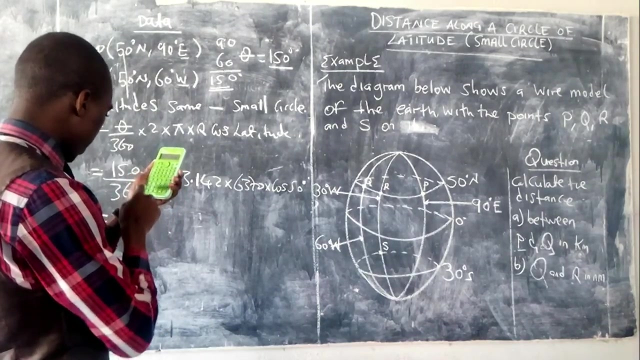 giving us All right. So we have 150 divided by 360, multiplied by 2, multiplied by 3.142, multiplied by 63,, 70 multiplied by cos, 50 degrees. And here, okay, assuming we have punched this, this, let me just start. 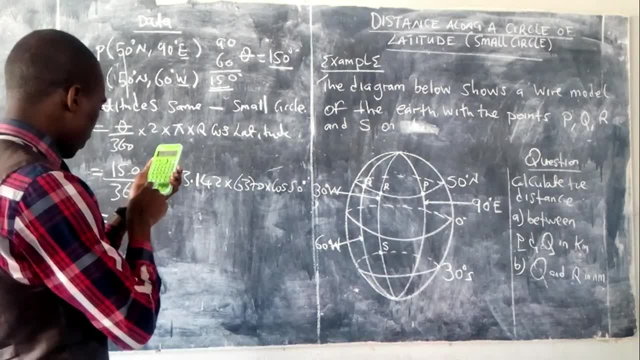 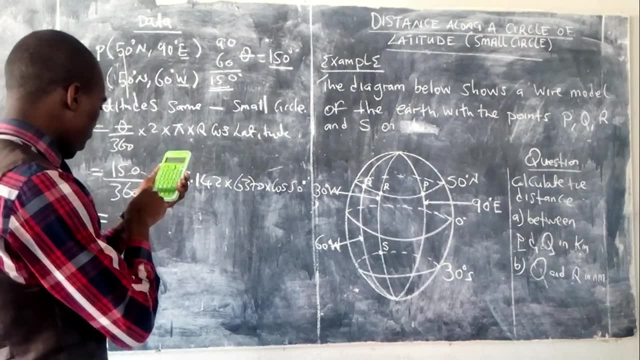 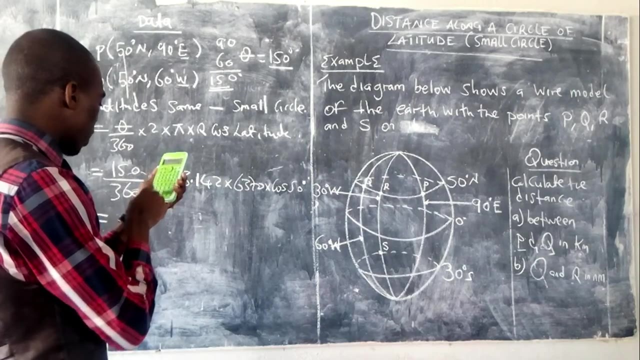 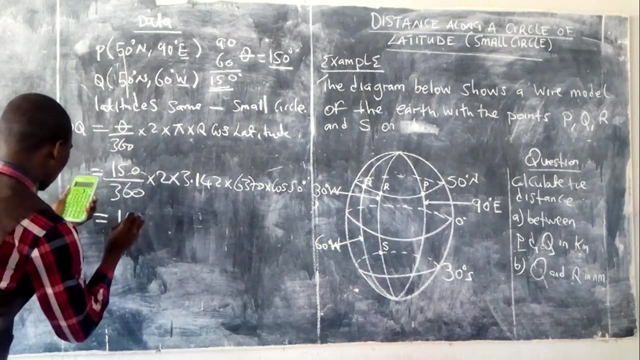 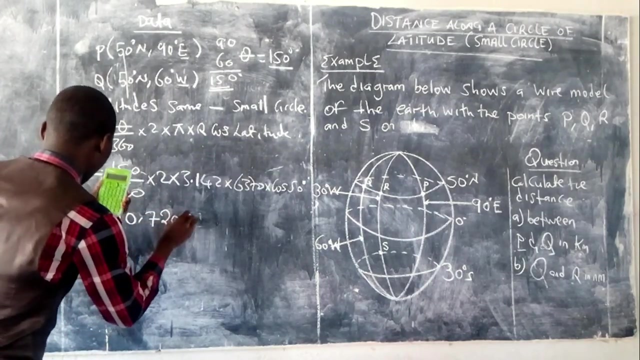 First of all, that is 150 over 360 multiplied by 2.. So we have 150 divided by 360, multiplied by 2, multiplied by 3.142, multiplied by 63, 70 multiplied by cos 50 degrees. So this one is giving us something like 1, 0, okay, 1, 0, 7,, 2, 0, 9, 1, 5,, 6, 7,. 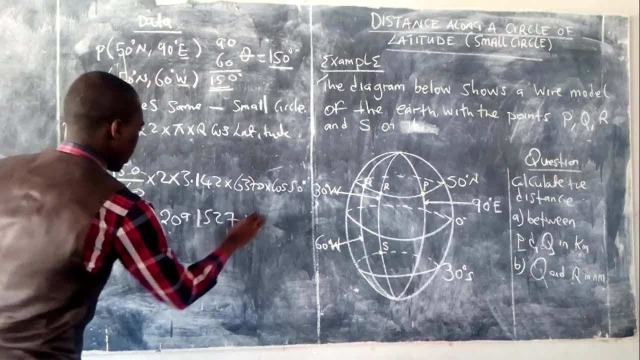 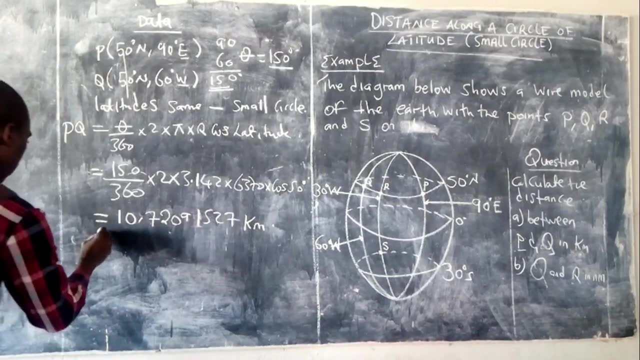 8,, 9,, 10 in kilometers. Okay, so what we're going to do is we're going to round off this one. We can round off this one, Okay. So, since there is a point- okay, actually there is a point after here- there is a point. 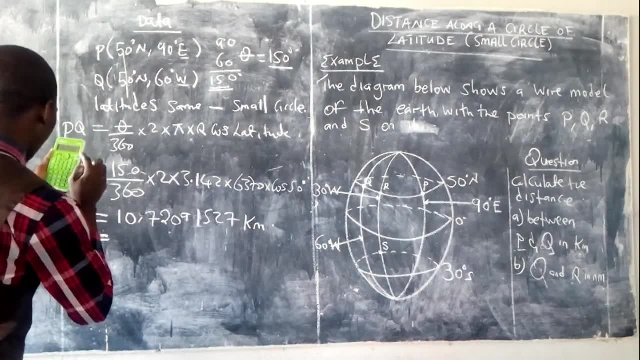 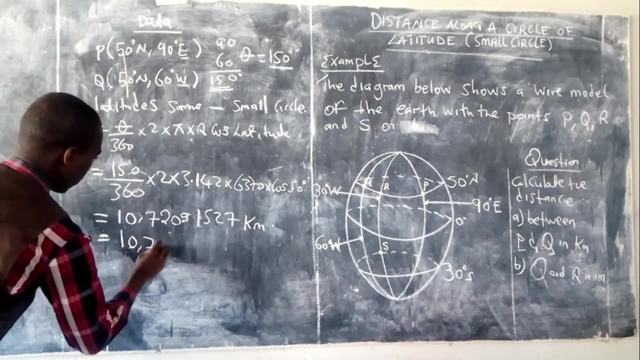 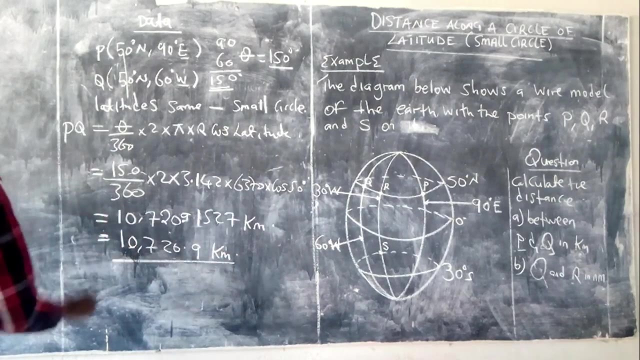 here. So we can just say this is 1, 0,, 7,, 2, 0.9 kilometers multiplied by 60.. So that is our distance between P and Q. That's how it is done, okay. 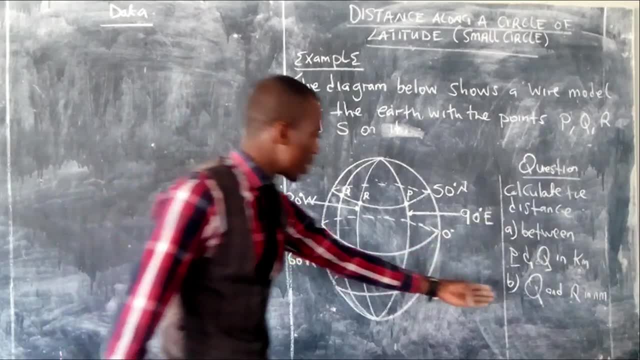 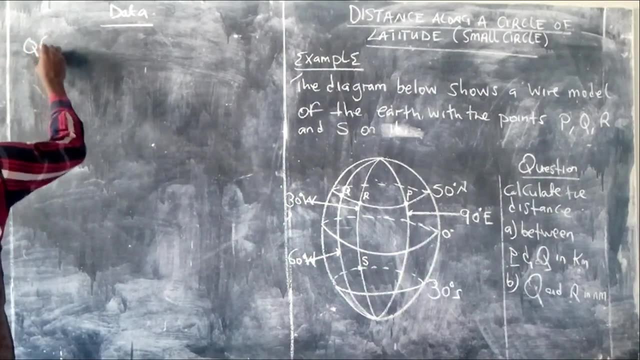 So now let's solve also the distance between Q and R, and this one is in nautical miles. So we are going to collect the data, we write the coordinates of Q, So Q, here we check, this is 50 degrees north. 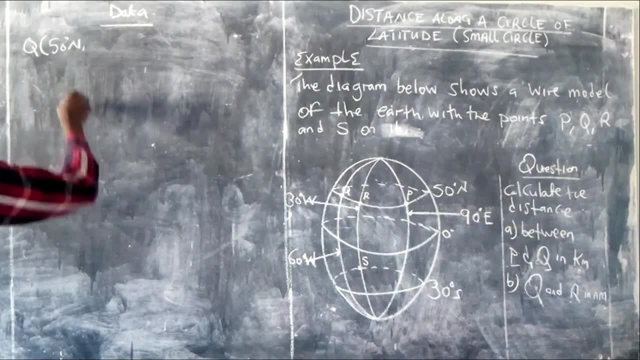 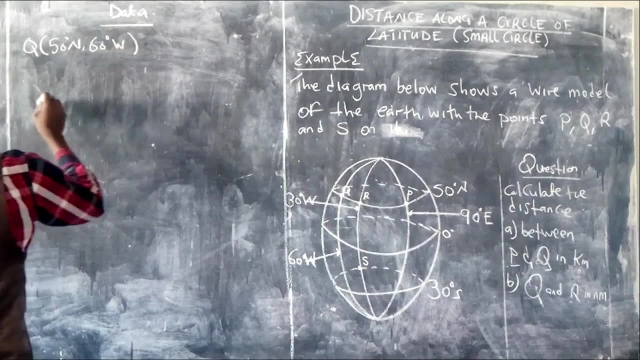 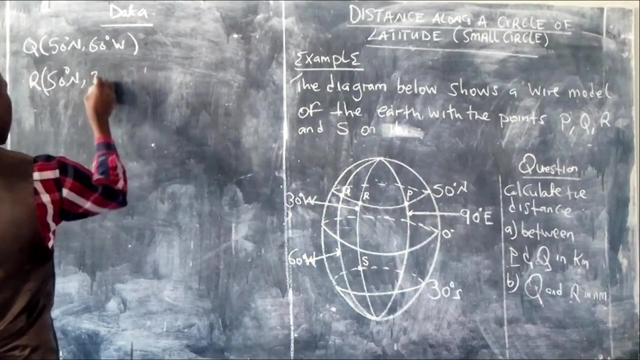 So that is 50 degrees north. okay, So this one is 2.6 degrees west. Then we go to R. okay, So R is this one here which is also still on the same latitude, which is 50 degrees north, 30 degrees west, okay. 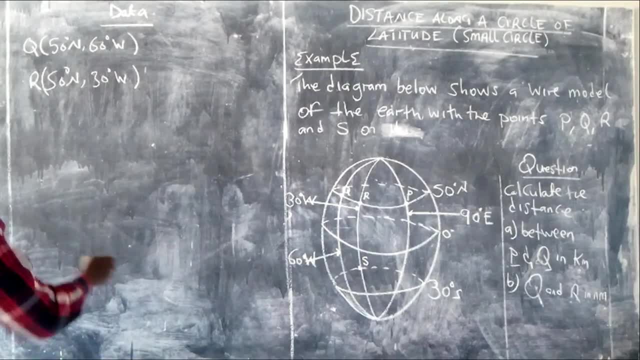 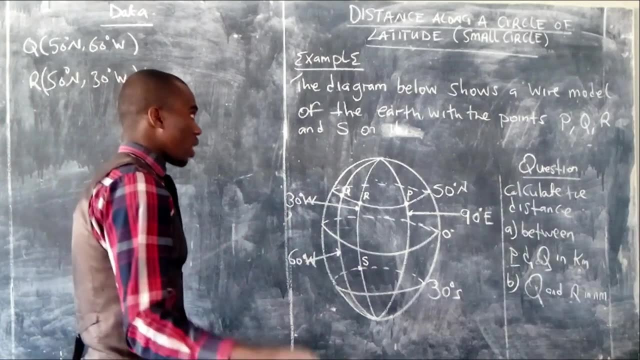 So this is what we have. So again, as you can see, since these two points are on the same latitude, it means that we are dealing with a small circle. So this is distance along a circle. of what Latitude? 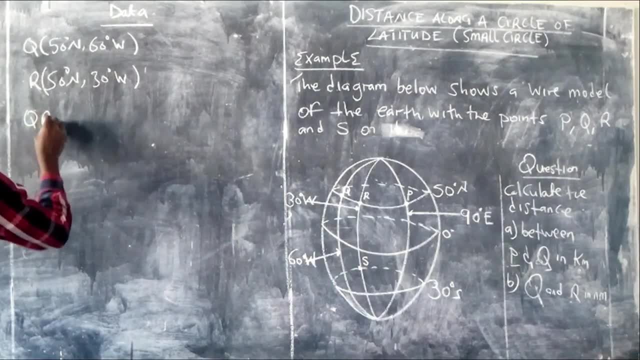 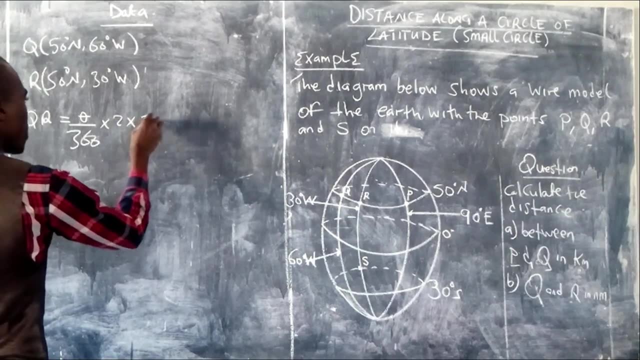 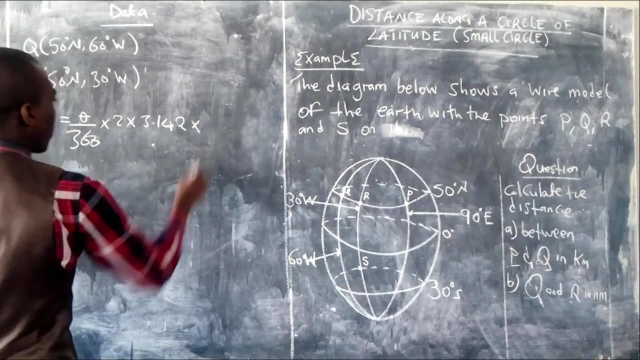 So therefore, the formula is going to be: Q. R is equal to feature over 350, multiplied by 2, multiplied by 3.142.. That is our pi, then multiplied by. because now, where there is R, where there is R, 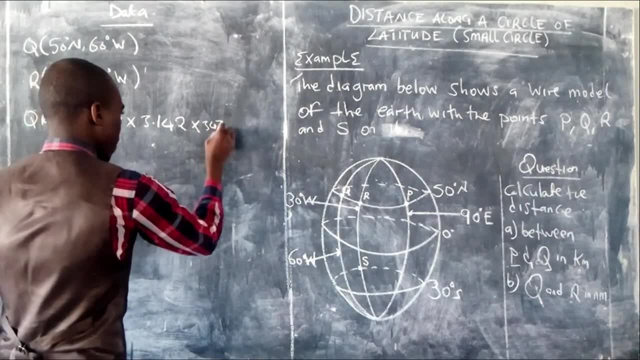 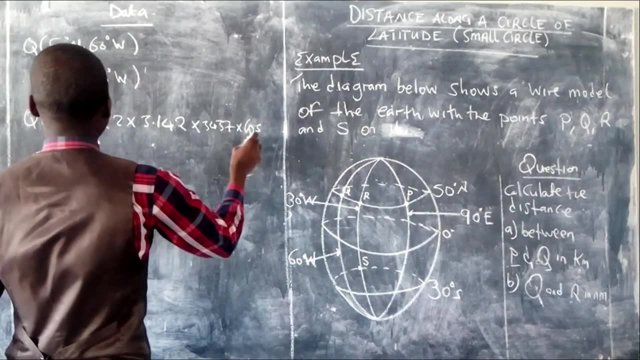 we are going to put 34,, 37, because we are finding the margin in nautical miles, Then this should be multiplied by 4c. okay, This one will be 4c 50, because this is for latitude. 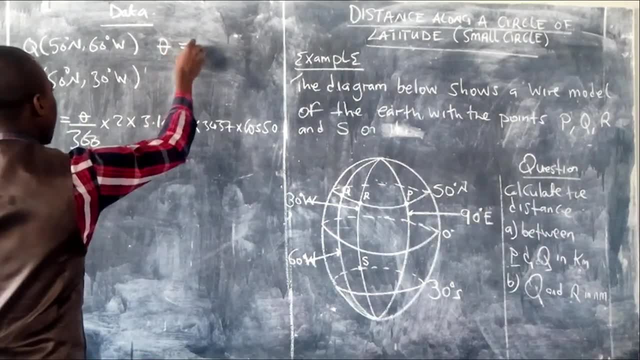 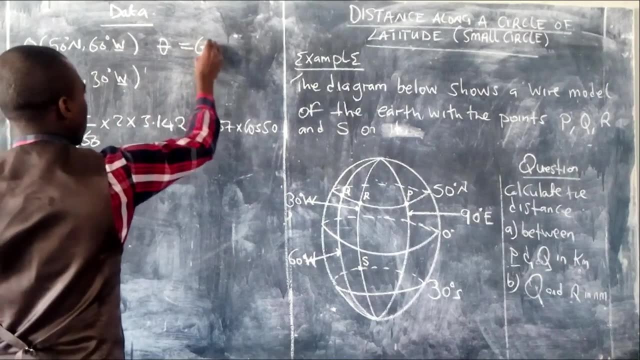 Then here on theta we are going to find the difference in e longitude here and now, because they have the same sign: west. west. it means we are subtracting, So this one will be 60 minus 30, which is equal to 10.. 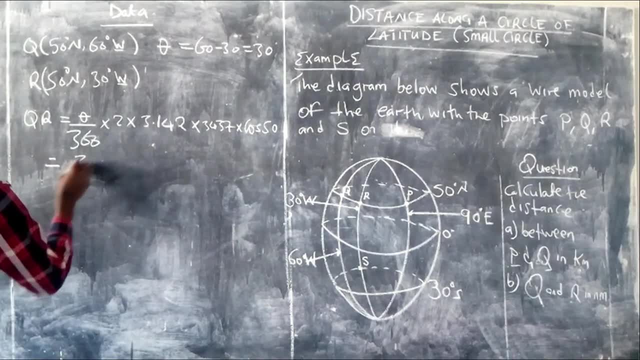 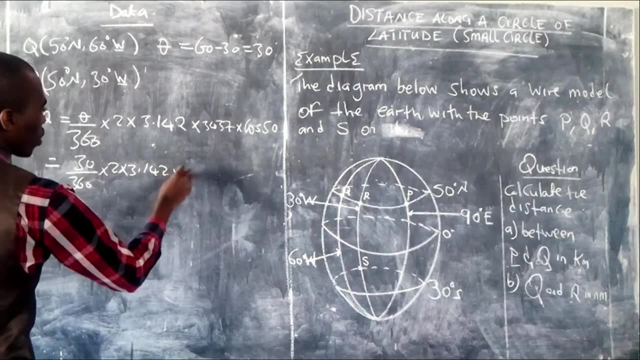 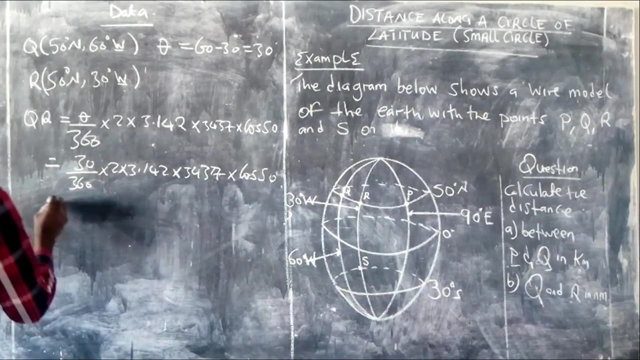 So what we are going to have now is this: one will be equal to 30 divided by 360, multiplied by 2, multiplied by 3.142, multiplied by 34, 37, multiplied by 4c, 50. Okay, 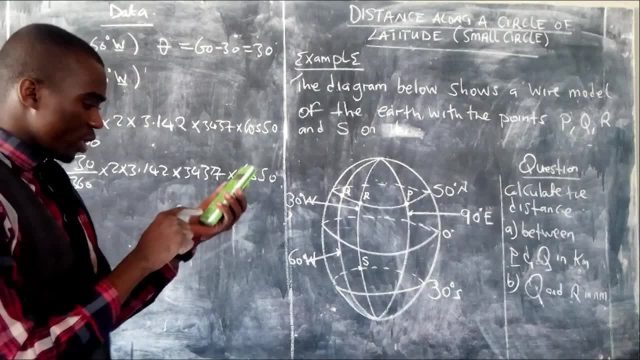 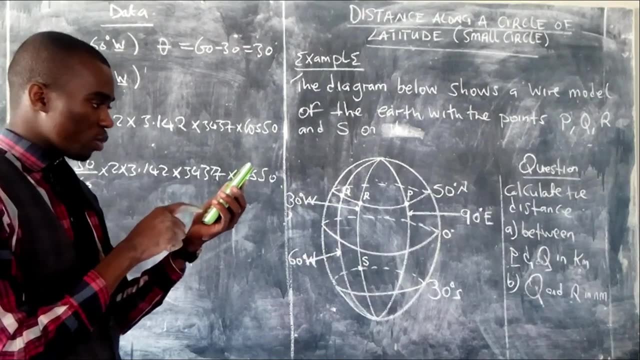 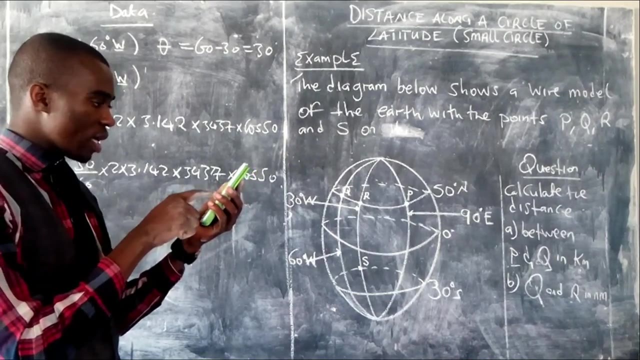 So we can evaluate this one using our calculator, which is 30 over 350 multiplied by 2, multiplied by 3.142.. Okay Multiplied by 3.142 multiplied by 34,. 37 multiplied by okay Multiplied by cos 50,, cos 50,. 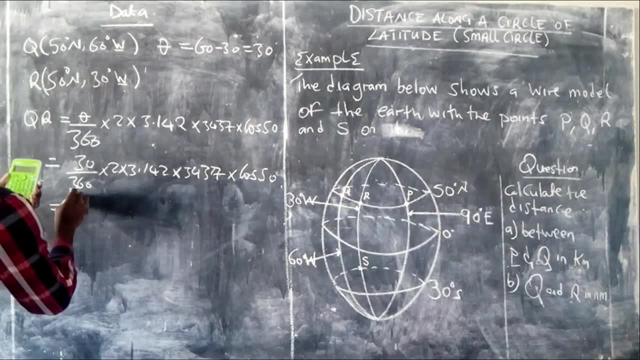 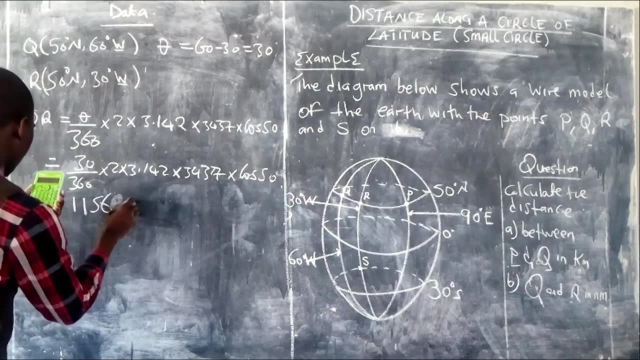 and this one is going to give us 1, 1,, 5, 6,- okay, 5, 6, 0.8, 9, 1, 6,, 3, 5, 1, nautical miles. 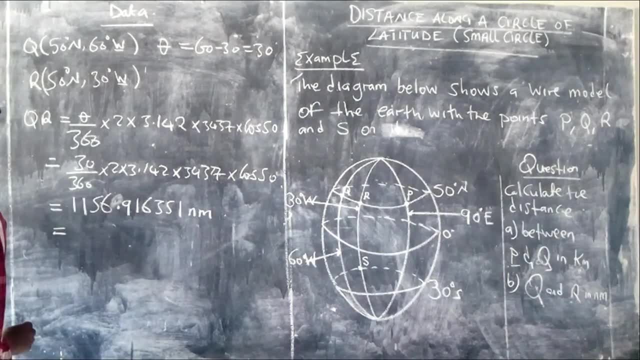 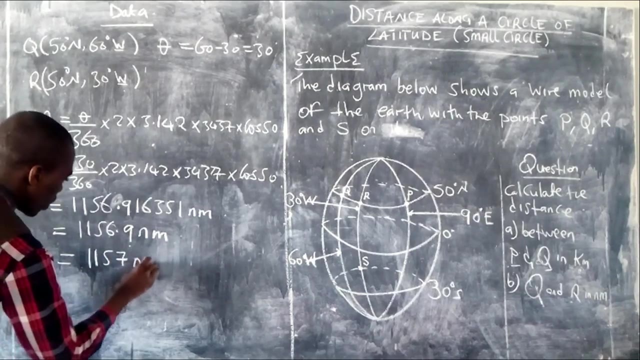 We round off this one to: so we can round off this one to 4c nautical. or we can either write it like 11, 56, 49 nautical miles, or you can say it's 11, 57 nautical miles. 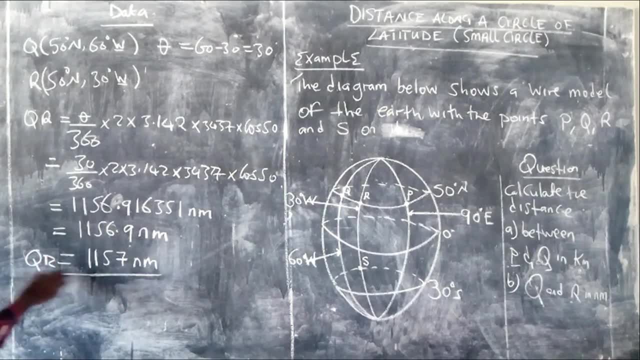 So both of them will be correct. So that is how we will deal with the distance along the circle of latitude. Next, let's remember the two formulas. So the two formulas, we have one, let me just. we have done these two. 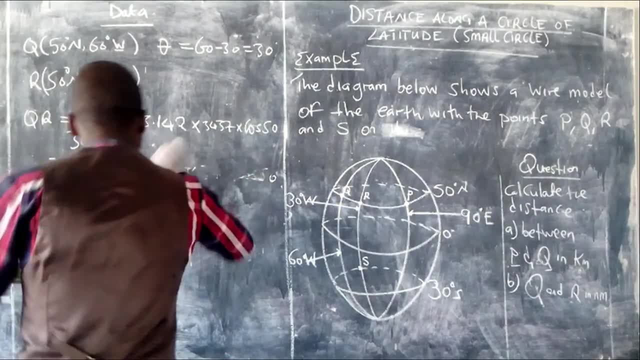 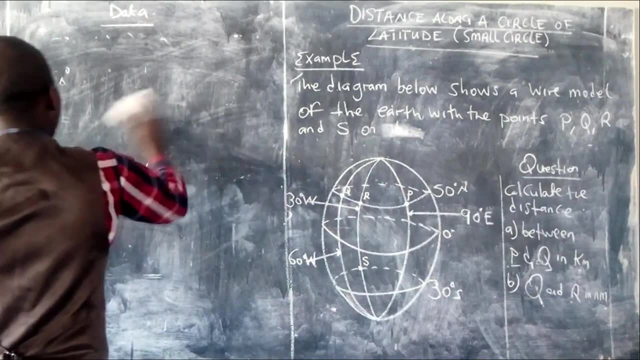 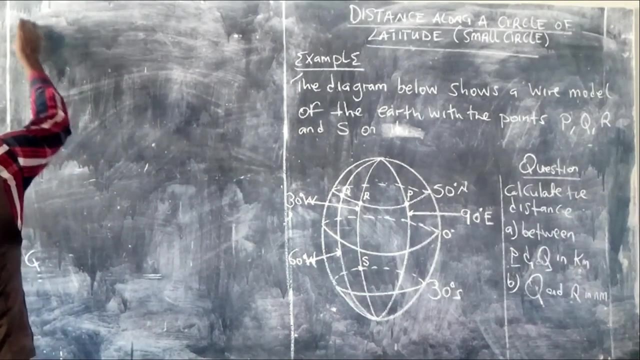 let me just give a recap on the two formulas so that you master them. These are the two important formulas that you are going to encounter when it comes to watching the distance. okay, So I am saying the one for the formula number one to know is where we are saying: 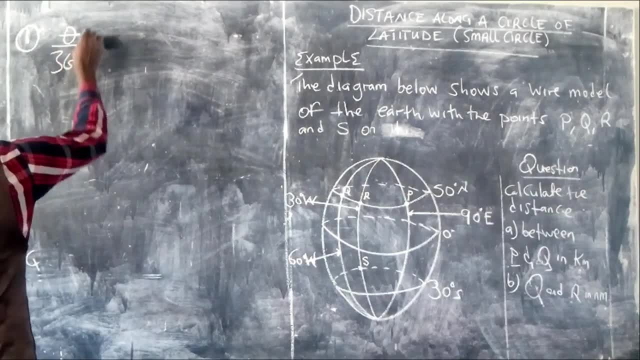 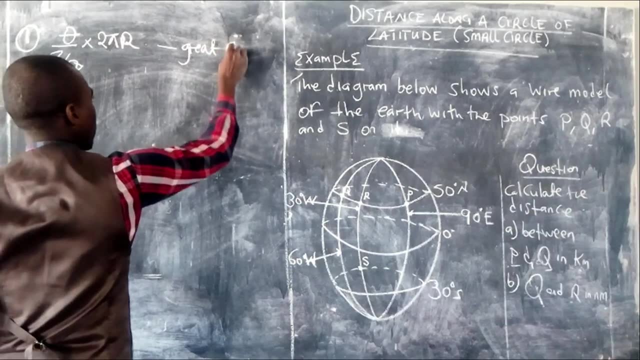 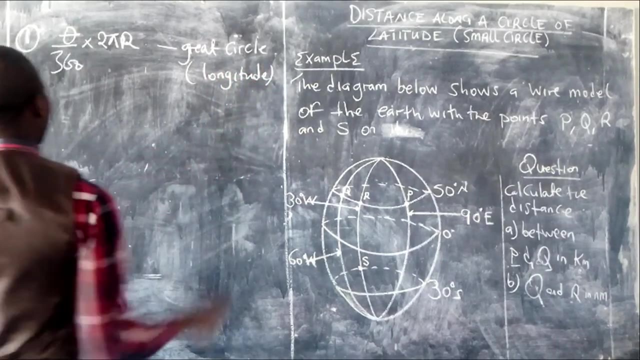 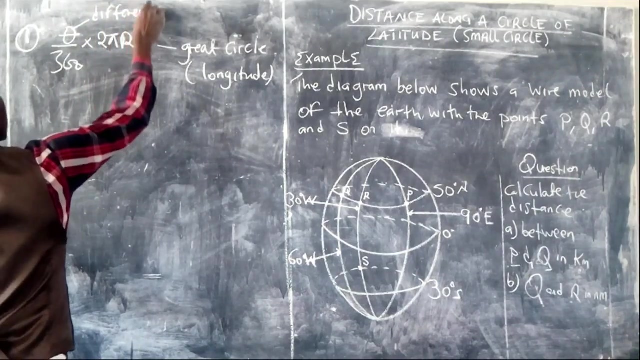 theta, okay, over 360 multiplied by 2 pi i. So this one is a great circle, okay, A great. what Circle? which is a circle along what The longitude? okay, Along the longitude. Then this difference here is the difference in. so this theta is difference in latitude, okay, 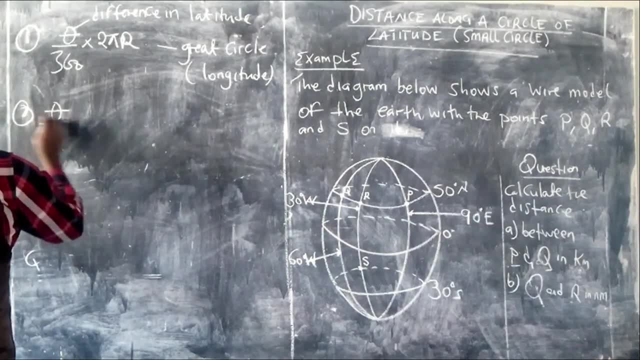 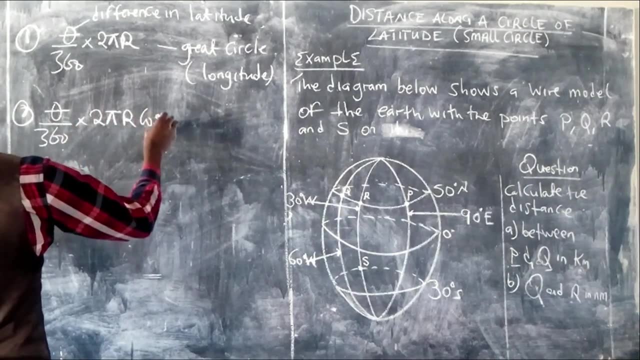 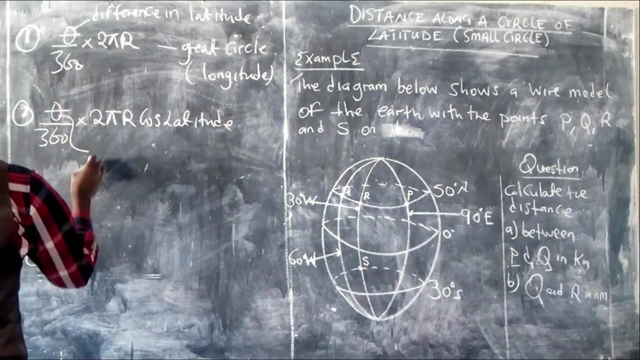 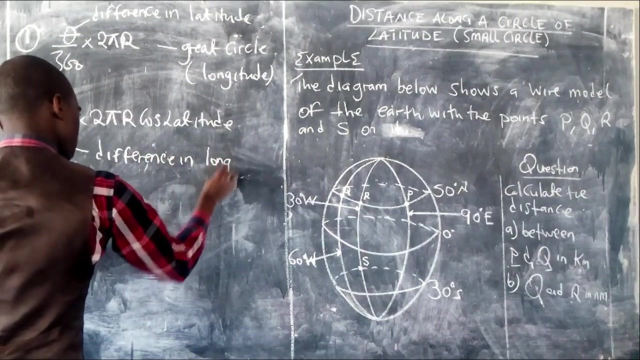 Then the second formula is theta over 360 multiplied by 2 pi r cos. what in Cos in cos? latitude, cos in latitude. So meaning this theta here is the difference, is the difference in longitude, It's the difference in longitude. 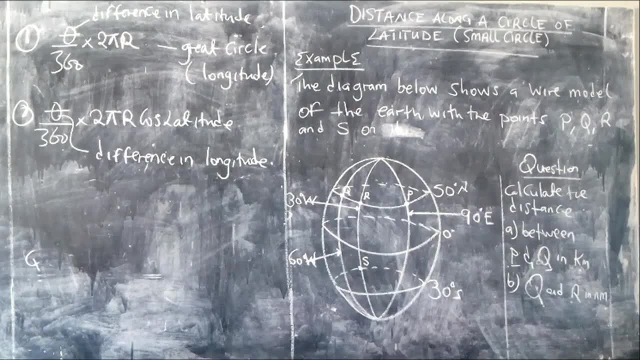 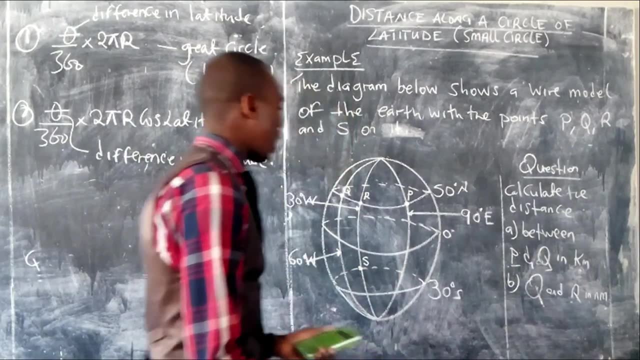 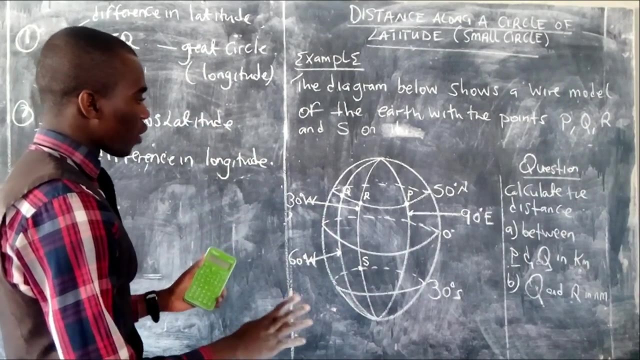 So once we understand this and also the fact that when we are finding in kilometers, the r to use is 63, 70, and when we are finding in multiple miles, the r to use is 34, 37. That one will get you to sort out different kinds of questions, alright. 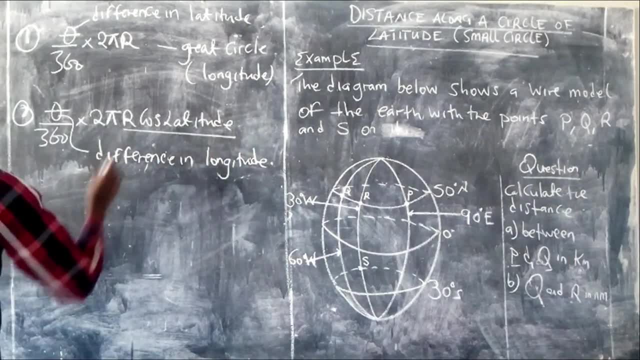 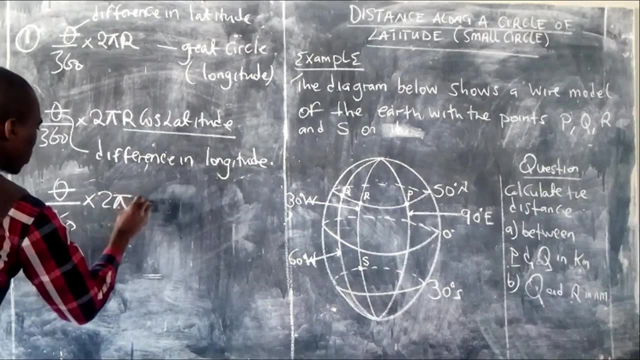 Now, what is the difference here? So this part here. in some other books we find the formula written like this: over 360, multiplied by 2 pi and a small r. So this one, this small r here, is the same as r. 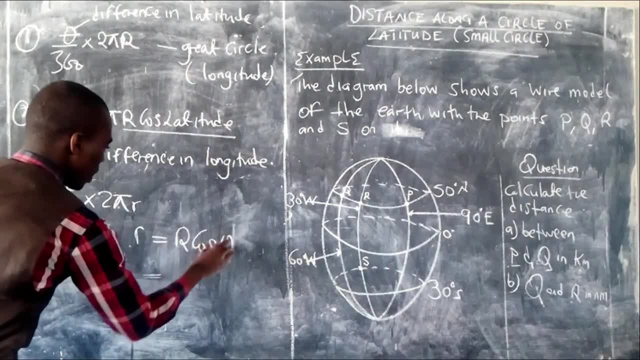 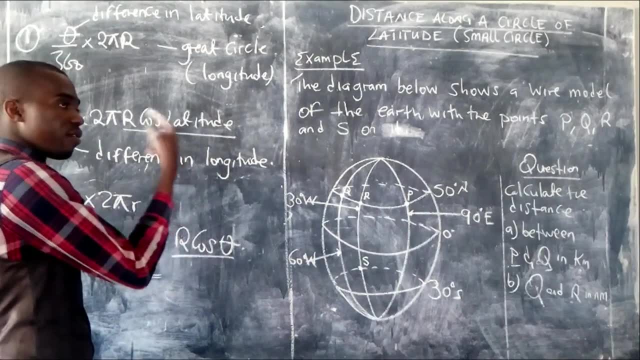 This one is equal to r cos theta. So if you want, you can use the small r, If you want, you can use this one, But I'm strongly advising, write the formula as I've written it, because it becomes simple and straightforward. 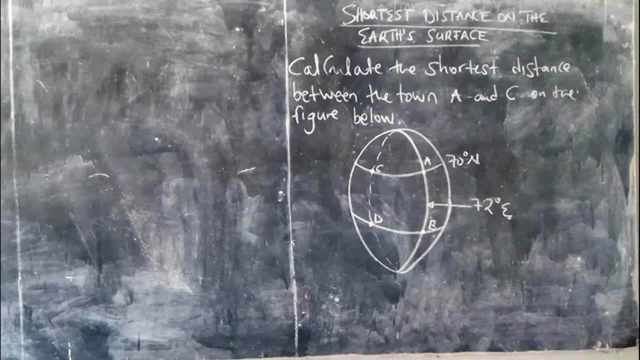 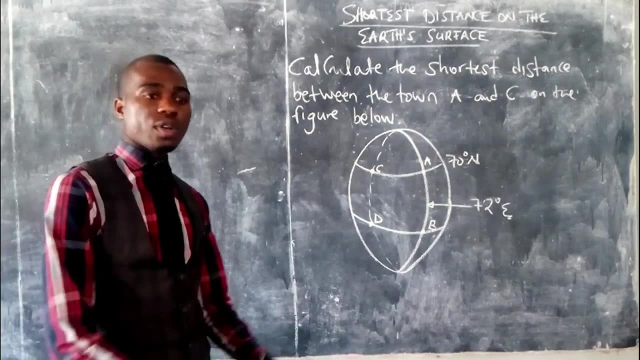 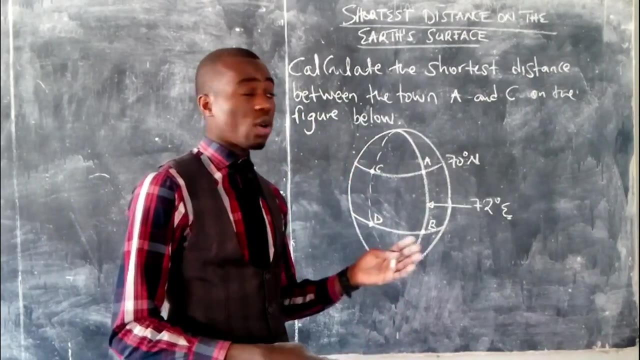 Alright, Okay, So let's also learn about shortest distance on the length surface. Now you know that there are two distances on the length surface. It's either the distance along the break circle or the distance along the small circle. Now, the shortest distance here is very simple. 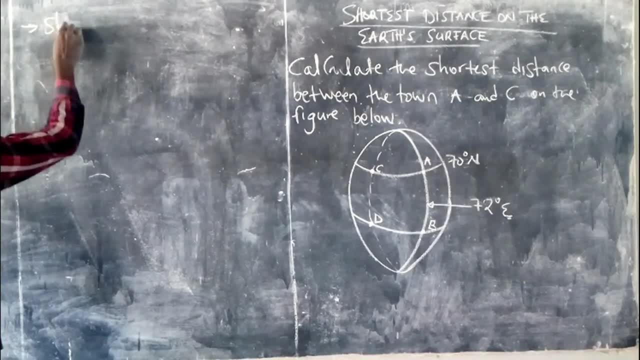 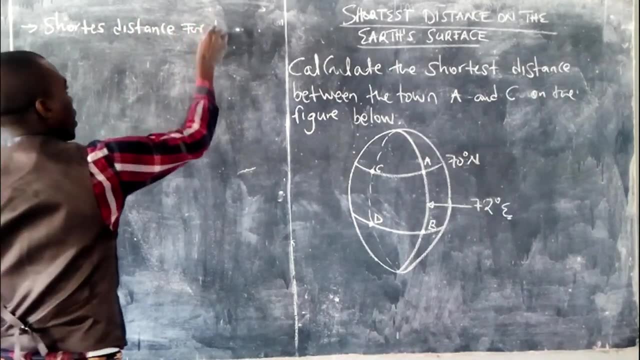 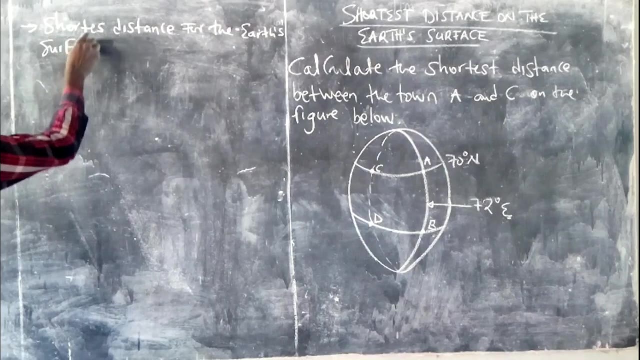 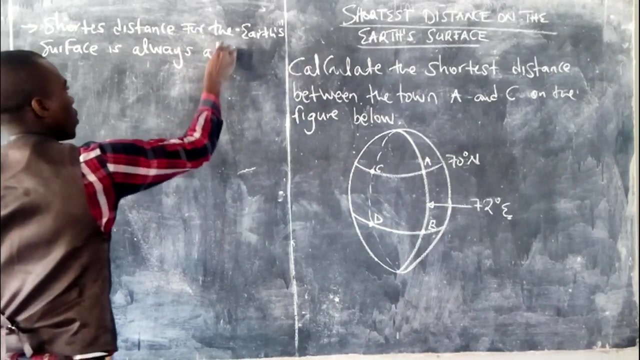 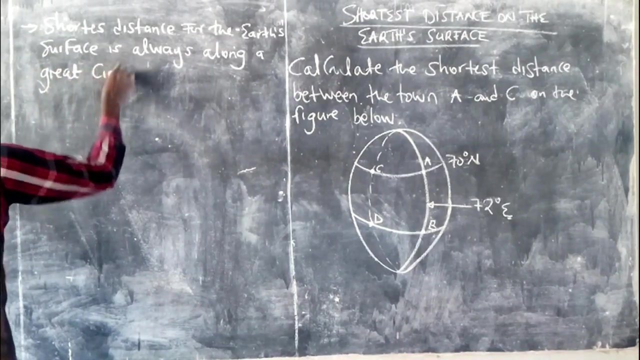 One thing that you have to know is, please note that the shortest distance, the shortest distance for the x surface, so the shortest distance for the x surface, is always along a break circle. It's always along a break circle, Alright. So now, having understood that one. 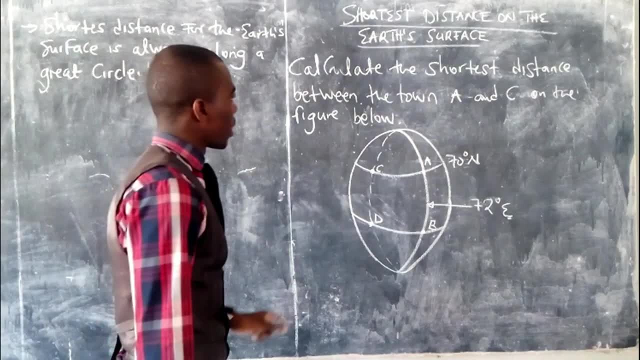 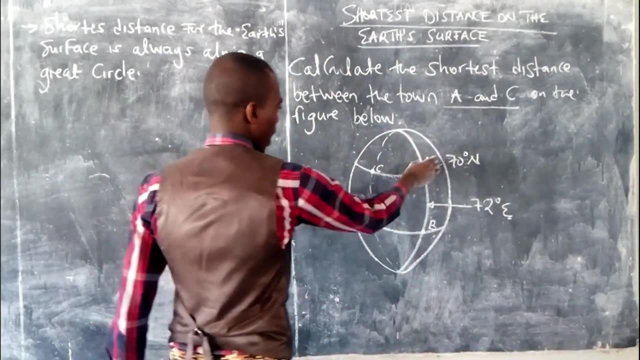 we are talking about. if you want to find it in this distance. we are supposed to find the distance, the shortest distance, between a and c. Now, when we look at a and c, a and c, you might be tempted just to find them. 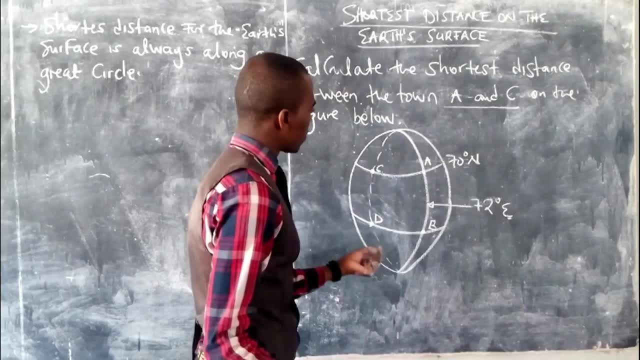 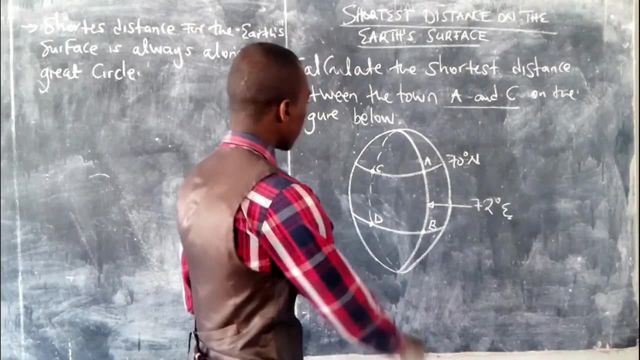 You are not sure. you have to say shortest distance. Am I finding the distance between me? am I finding the distance along this longitude or am I finding the distance along this circle of latitude? Now, since a and c are on the same latitude here? 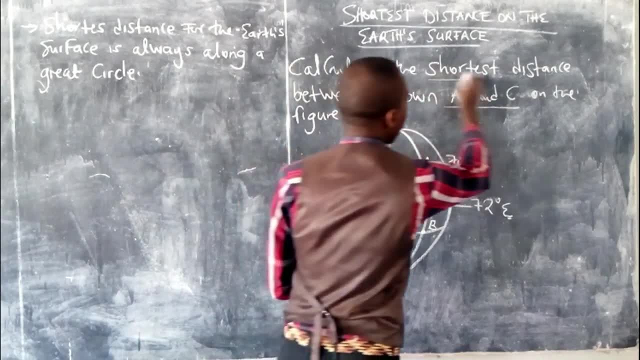 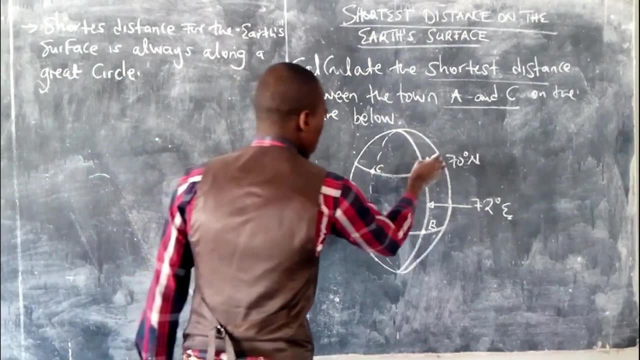 but you in your mind, because you are saying shortest distance, you have to know that, okay, shortest distance, it has to be along the circle of what Longitude. So, because this one and this one are here, meaning they have to form an angle, 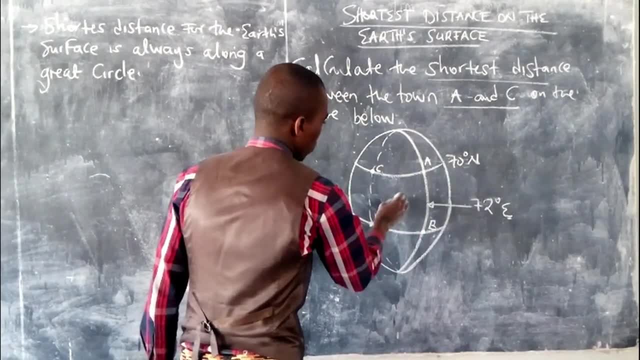 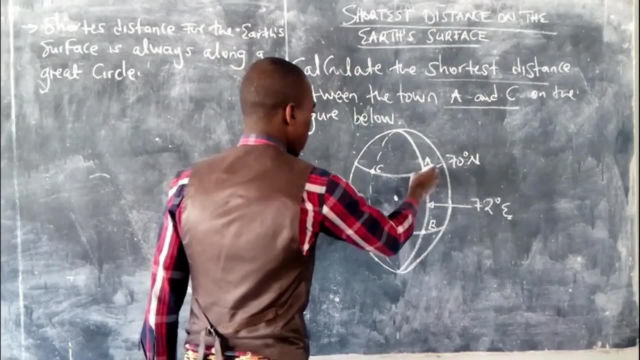 So here it is going to be like this. Here they should be in the center of the head, because all these angles, here they are written with respect to the center of the head, So meaning from there in the center of the head. 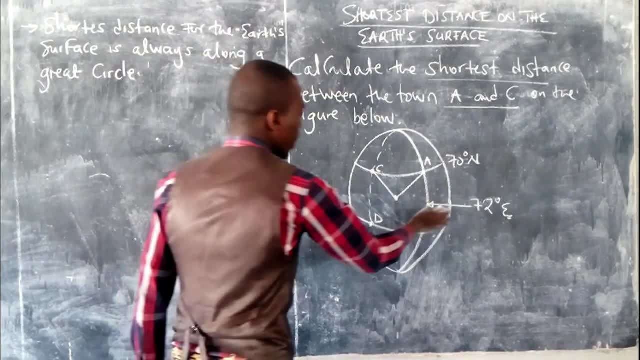 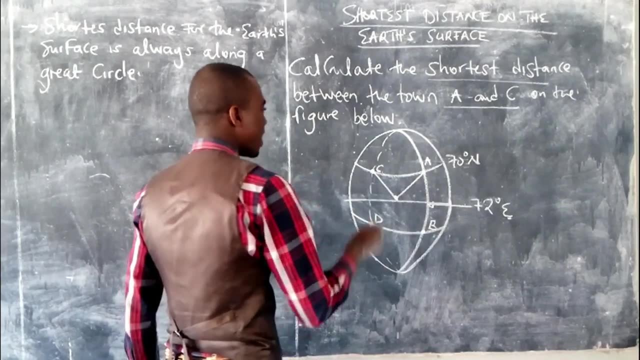 also this one from there, center of the head, and then the equator. here you are going to assume that it is a stretching line. So meaning what we are saying here is the distance now here, okay, so the distance between here and the center here. 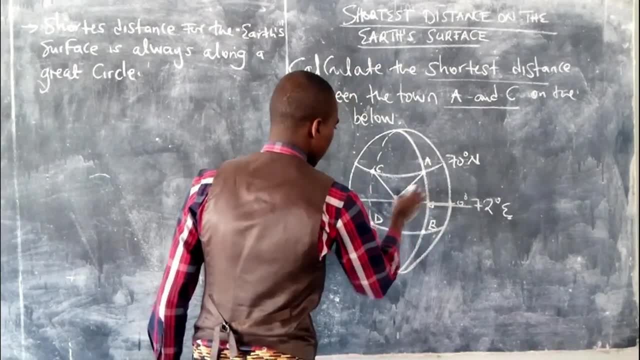 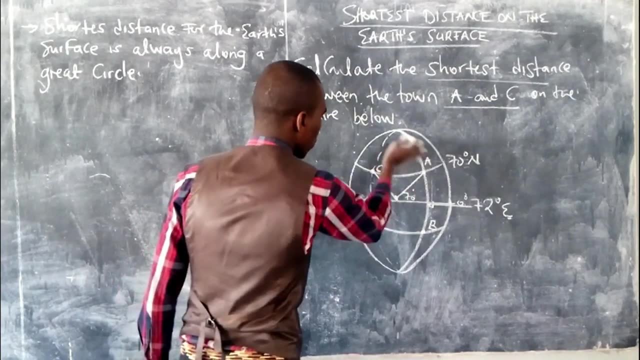 which is the equator, is 0 degrees. here we have 70 degrees even here, because longitude is in the past, this is in front and this is at the back. So since it is the same longitude here, even here, 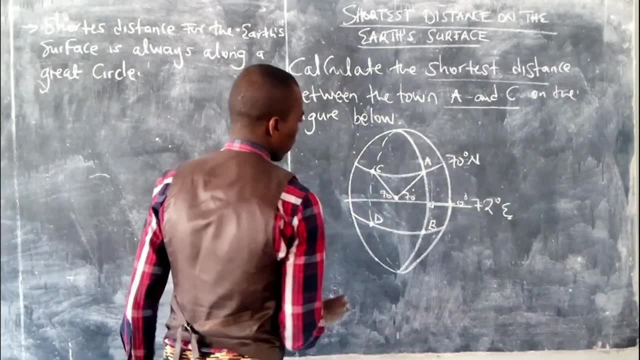 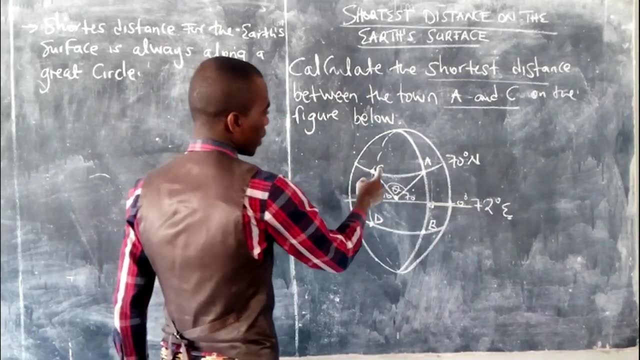 it is still the same severity. So even here we are going to avoid severity. So this angle here, this is the difference in it, the difference in latitude between it. this to here, Okay, So the difference between this one and this one. 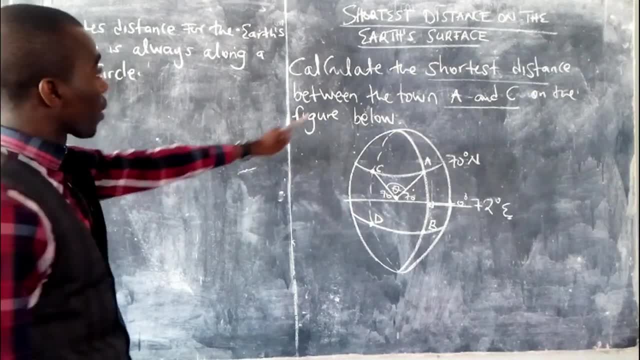 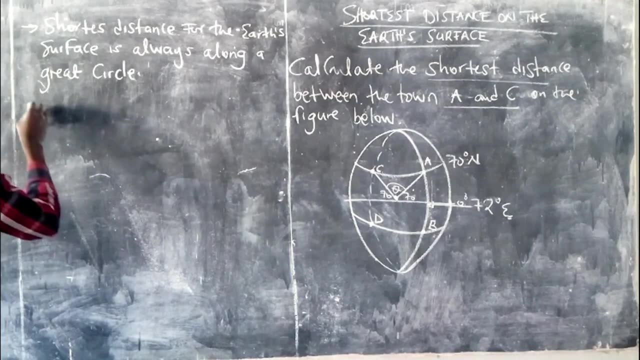 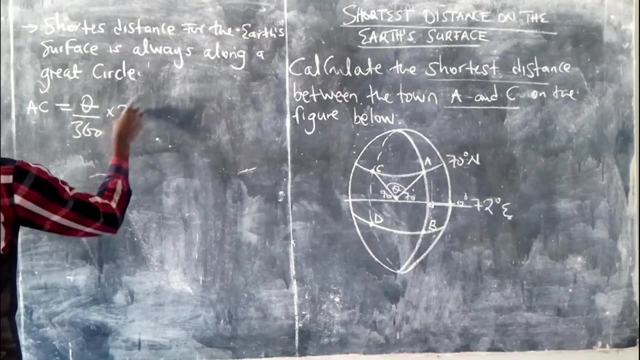 this is it what we are going to have here. So, because we have already figured out that shortest distance is the distance along a great circle, So automatically, given the formula that we are looking to, we know that AC is equal to theta over 350 multiplied by 2,. 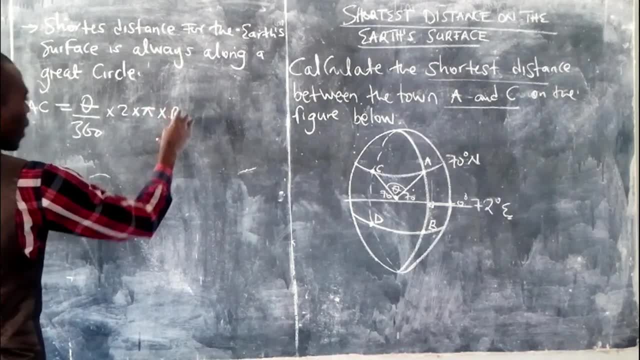 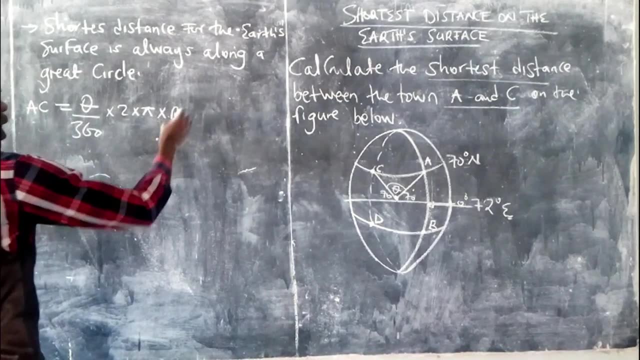 multiplied by pi, multiplied by what Ara? Okay, Yeah, so this is the way it is supposed to be. Now, here let's just find it in nautical miles. So the Ara we are going to use is 34,. 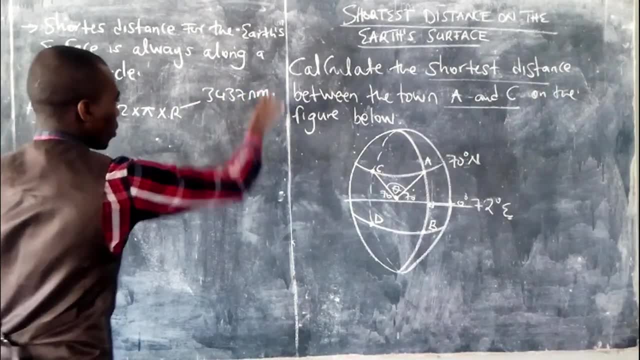 37, nautical miles. but the questions will always be clear. Okay, So, having known that one, so where do you get the theta? Because, remember, I was advising the issue of collecting data. So if we write the coordinates, 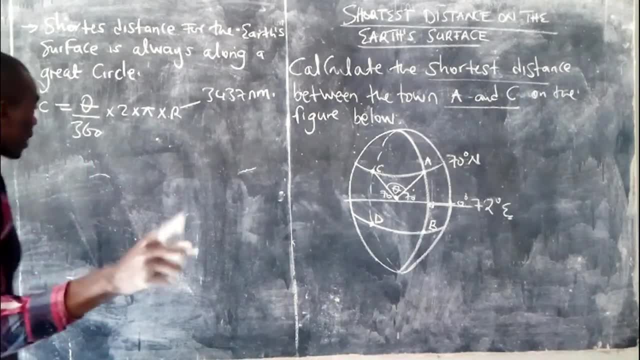 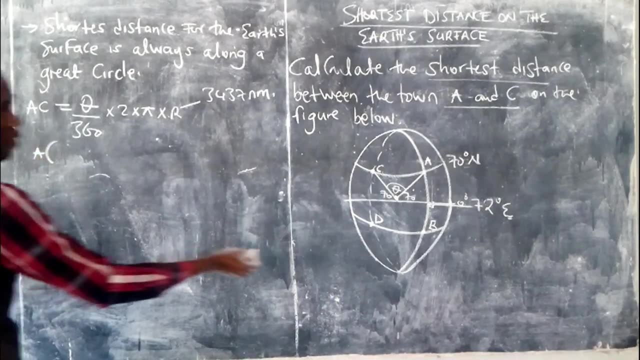 let's just write the coordinates. So the coordinates for A here, for this A, we have got it: 70 degrees north, okay, 70 degrees north comma 72 degrees. what is East? Okay, So if we write the coordinates, 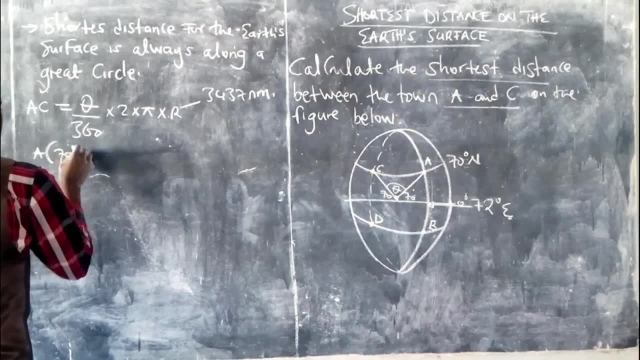 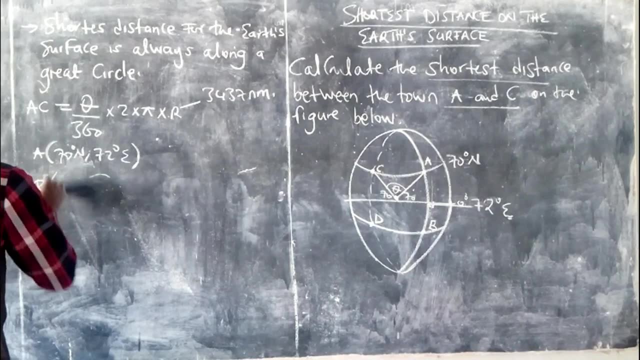 let's just write the coordinates. So the coordinates for A here. for this A, we have got it 70 degrees north, okay, 70 degrees north, comma east, all right, Then we go to B, okay. 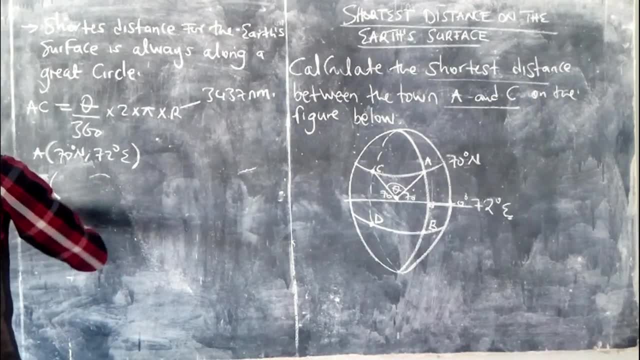 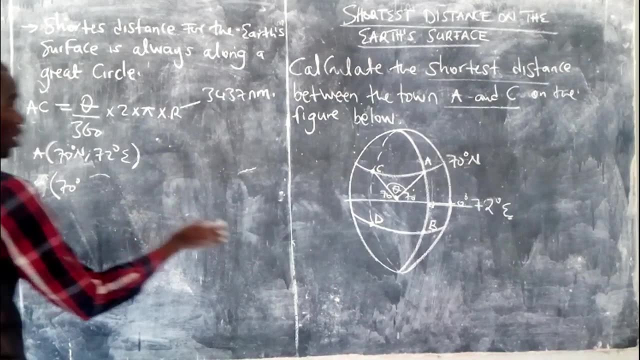 B, so to C, since we are doing A, C so to C, C is there, which is it's 70 degrees. okay, Now that this one here, it's on the other side, so actually. 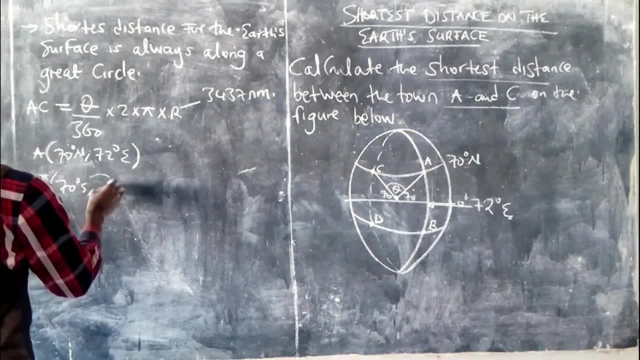 it's 70 degrees south comma, what we don't know, So we don't know So meaning. we cannot find the difference. we cannot find because here it is the same here, So this one cannot work. 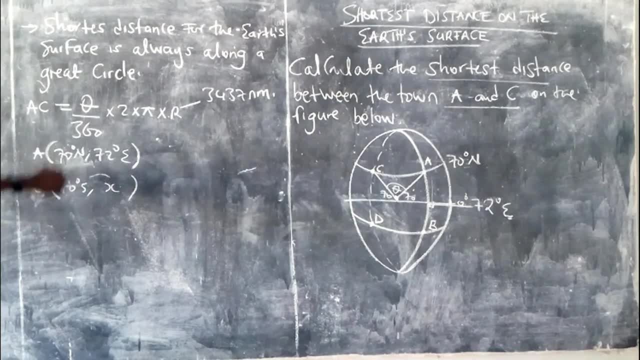 it is the same here, So this one cannot work. it is the same here, It is just confusing. So this method of collecting data, it cannot work here. So what you have to bear in mind all the time is this: 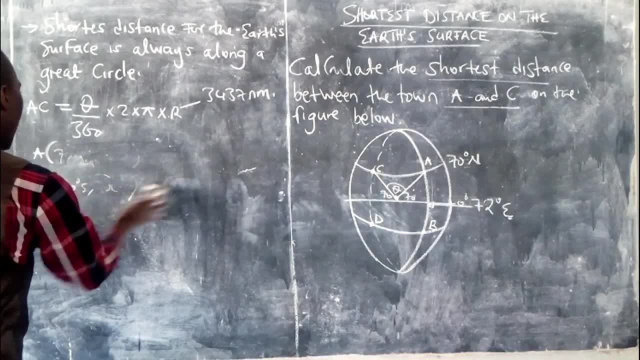 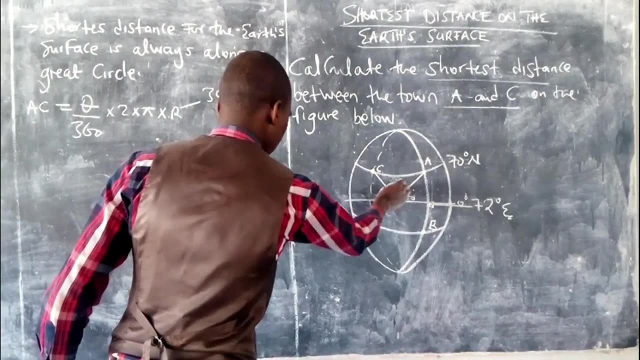 whenever you are finding the shortest distance on the edge surface, please always remember that there is an angle involved. okay? And when you collect data and you find yourself in a situation like what happened here, just know that that procedure cannot work, So what you have to go for? 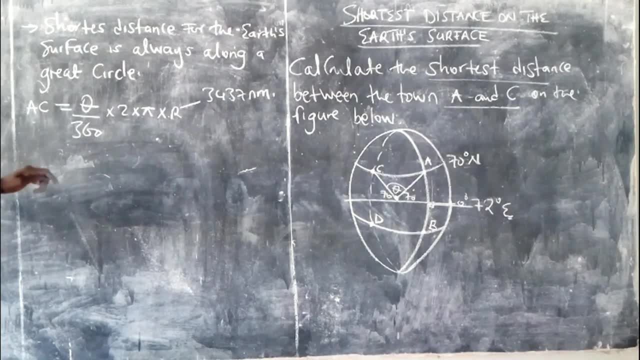 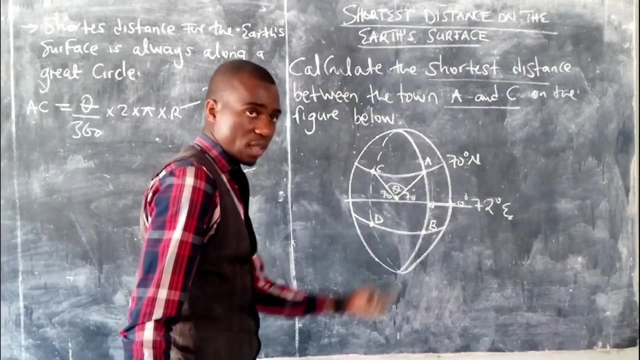 is actually this where you are now, So let's go back to the first one here. we have to make this angle here in between. okay, Now, look at this is a straight line. So a straight line angles on a straight line. 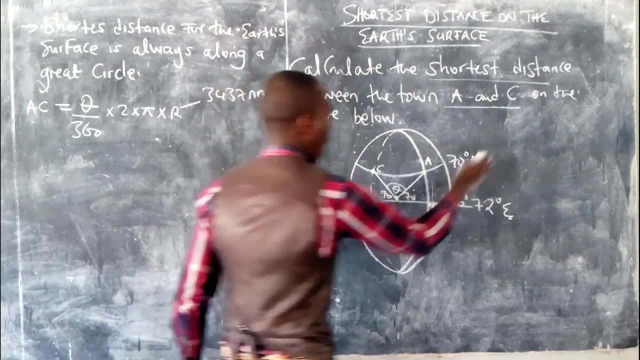 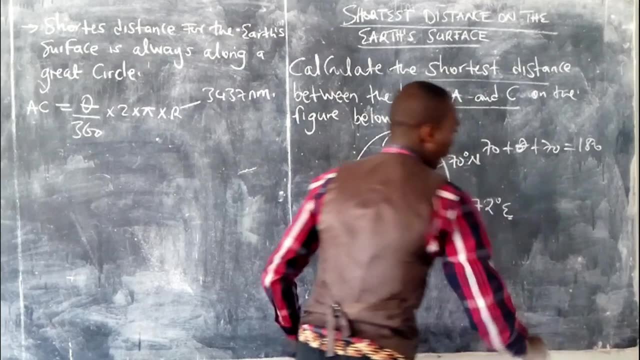 they add up to 180.. So what you are going to do is you are just going to add 70 plus theta plus 70 is equals to 180, because angles on a straight line, they add up to 180, okay. 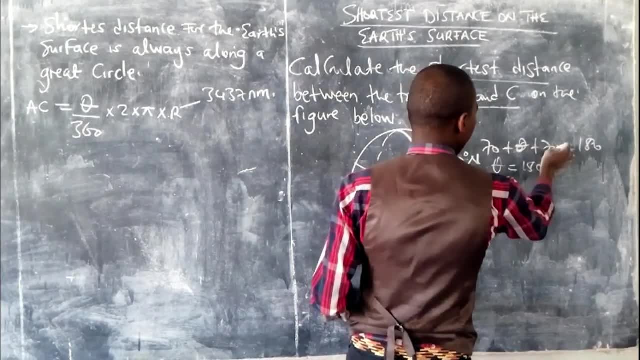 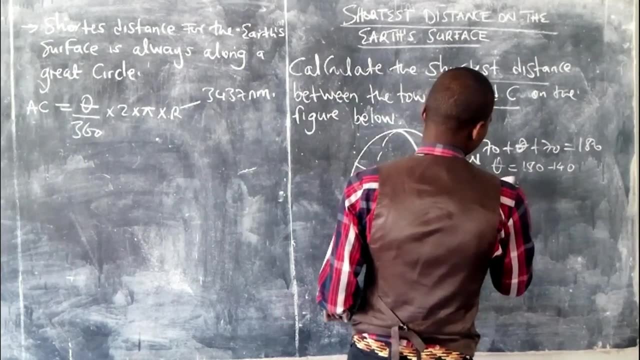 So this one in theta is equals to 180,. when it crosses to the other side it is going to be minus 140,. okay, So we subtract that one, our theta is going to be 40 degrees. okay, So we have found. 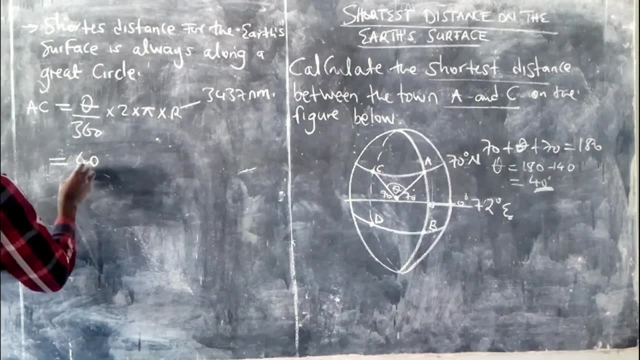 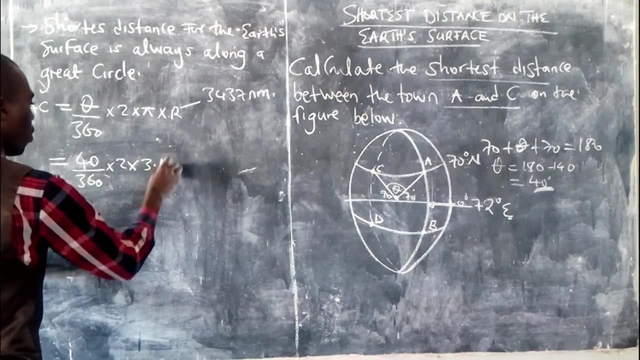 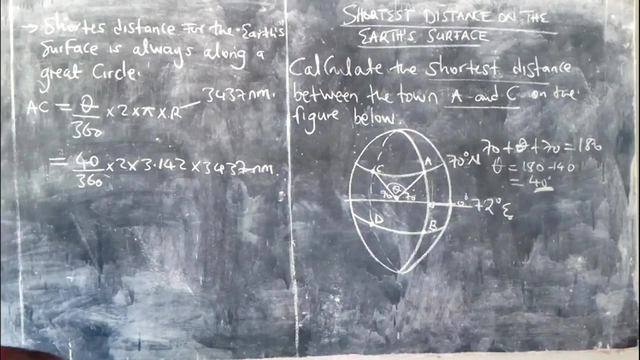 that one. Now let's see if we can substitute in here. So we are going to have 40 divided by 350, multiplied by 2, multiplied by 3.142, multiplied by 34, okay, So that is what you do. 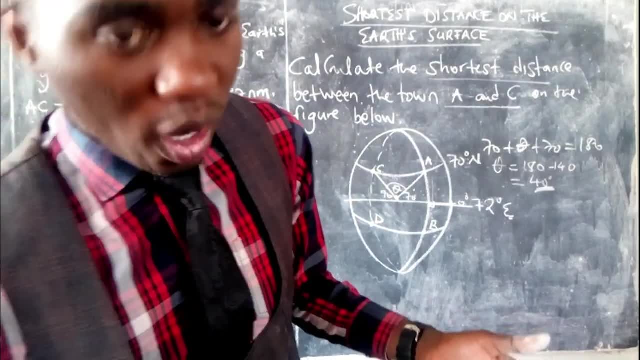 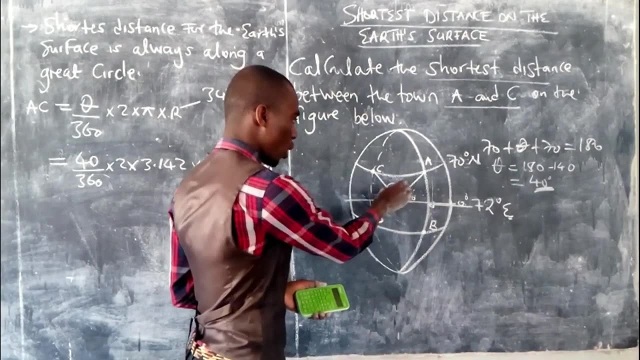 Please remember, whenever shortest distance is involved. what you have to do is whenever shortest distance is involved. just know that you have to find this in handling. okay, What I am telling you is what you are supposed to do And how you know that. 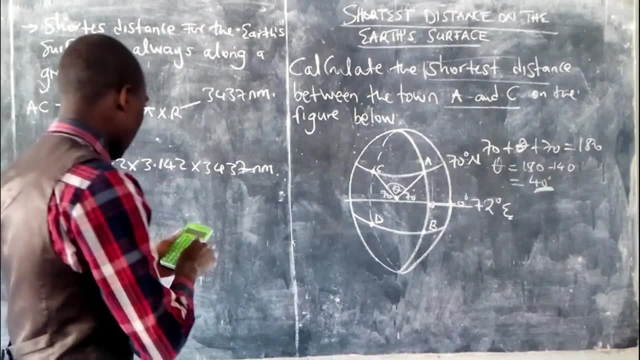 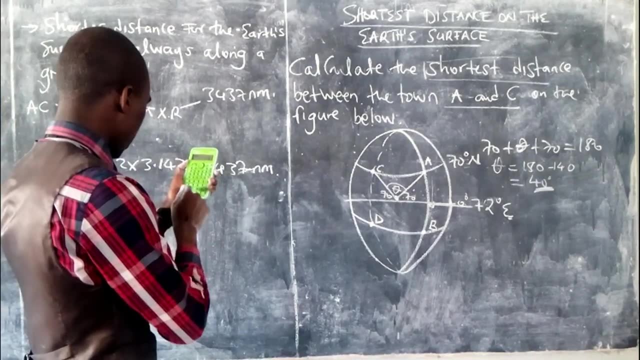 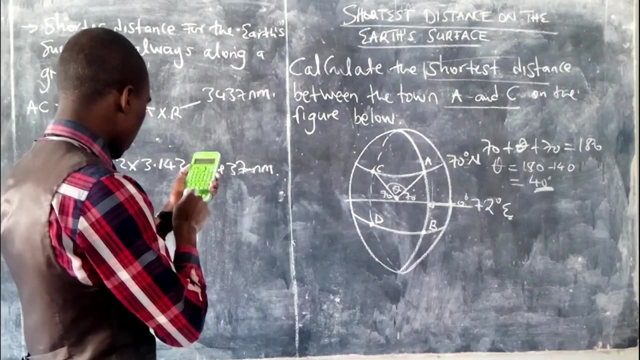 is when, every time, this is involved. okay, So let's patch on the calculator and see what value we are going to come up with. so that is over 350 multiplied by 2, multiplied by 3.142, multiplied by 34, 37. 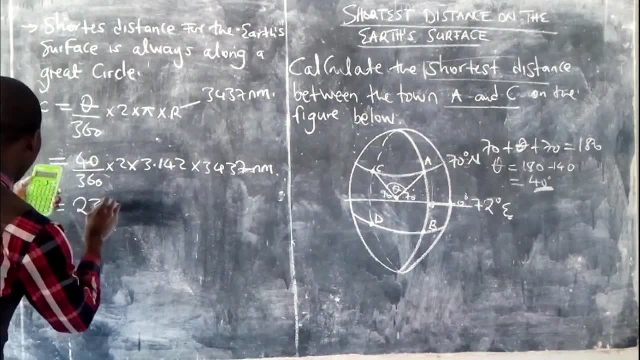 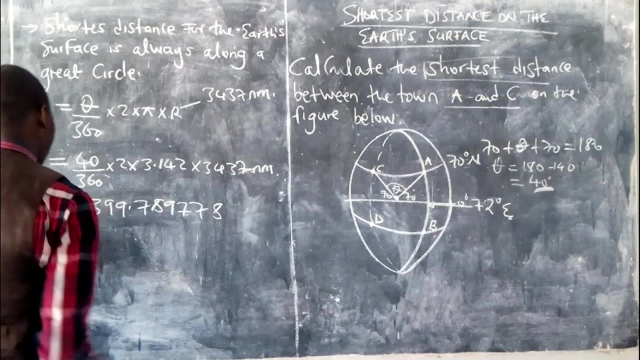 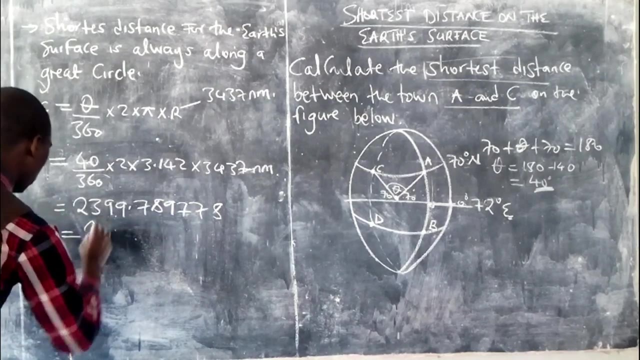 and this one is giving us 23,, 9,, 9,, 4,, 7,, 8,, 9,, 7,, 7, 8.. So round off this one, If you can round off to 24,. 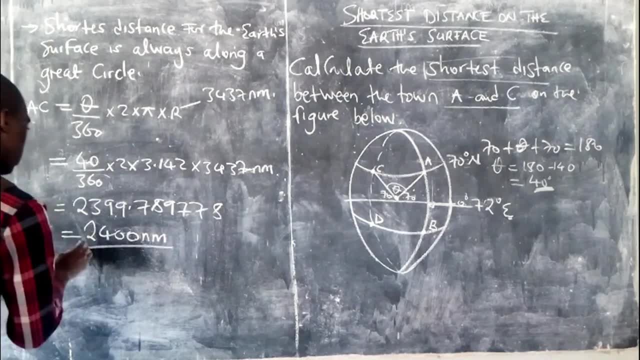 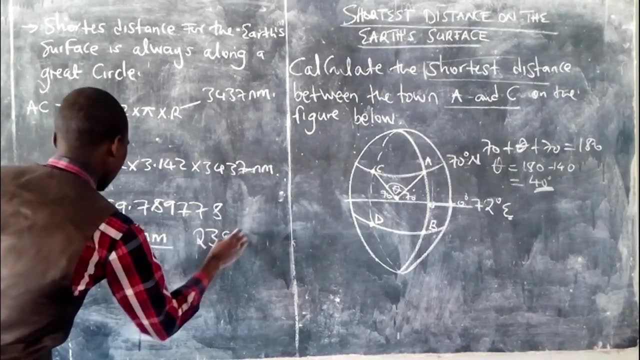 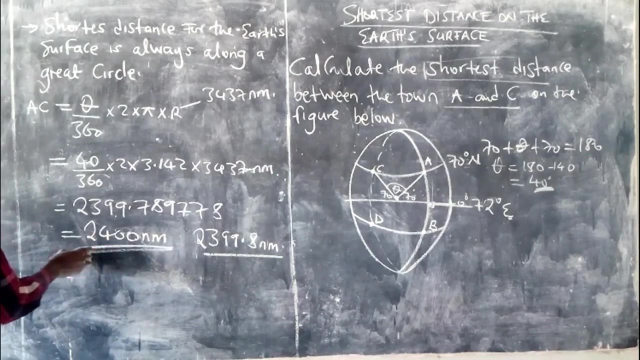 4, 100 nautical miles, But for those who apply into one desk in place, even this one will be accepted. 23, 99.8 nautical miles. even this one will be okay. All right, So that is how. 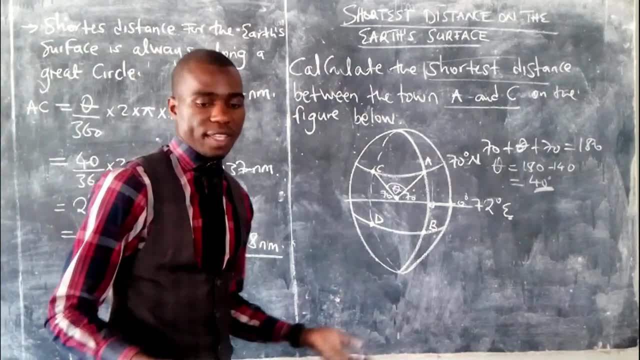 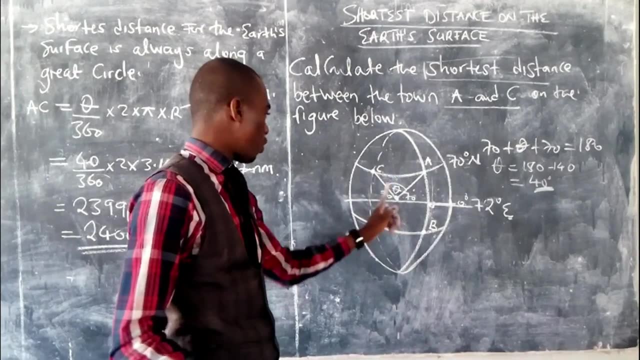 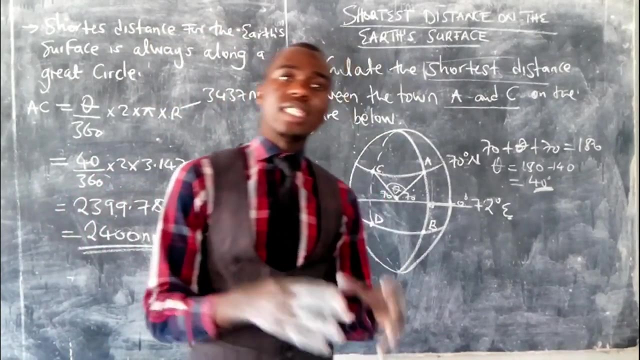 you deal with the shortest distance on the head-swatting surface. Please remember, whenever you are dealing with shortest distance, you are supposed to find an angle in a similar manner like this one, And distance shortest distance on the head-surface is always the distance. 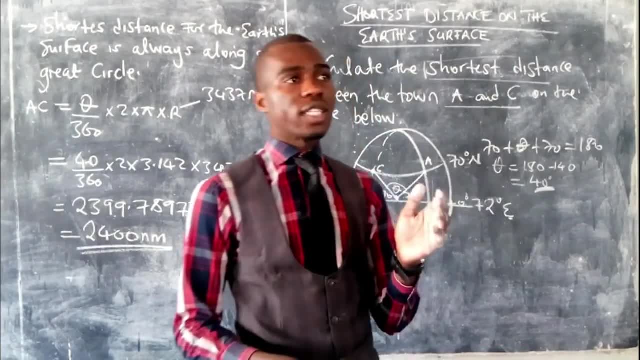 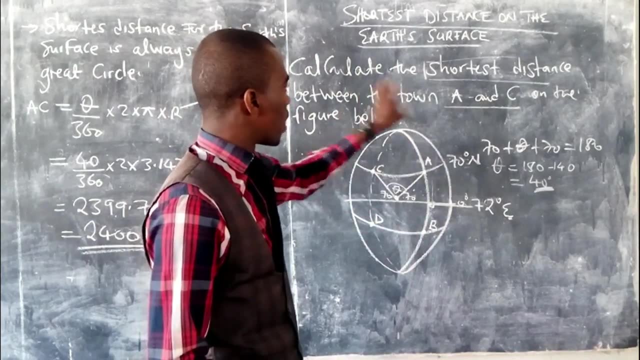 in a great circle. So a great circle is a circle of what Is a circle, along what Longitude. So that is how you handle with it and that is how you handle this one. So I am sure of this concept that we have. 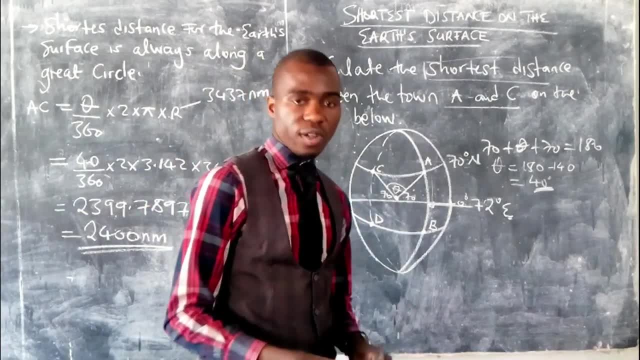 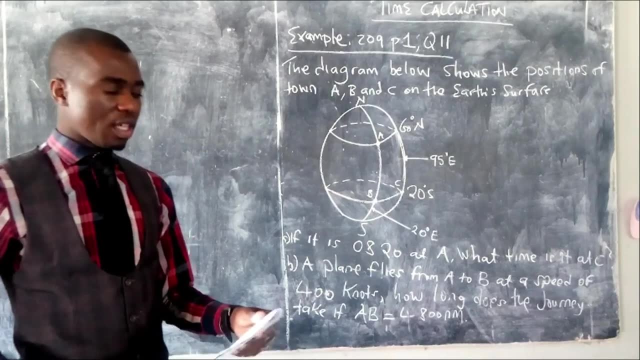 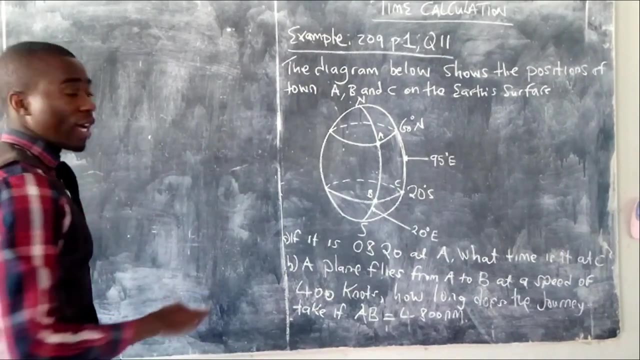 made, you have no problem with success in the exams. Okay, So we now look at the time calculation. So now the few things that you have to know about time calculation is: whenever you are trying to find time, you always use longitude. 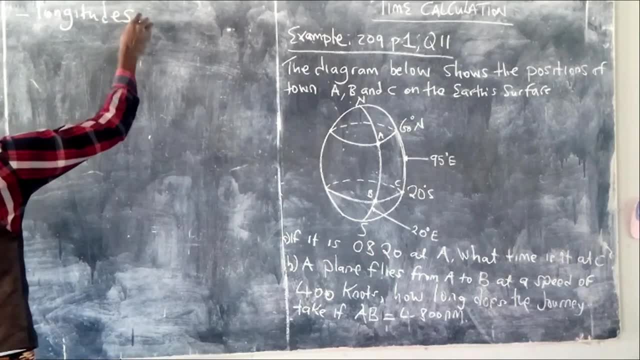 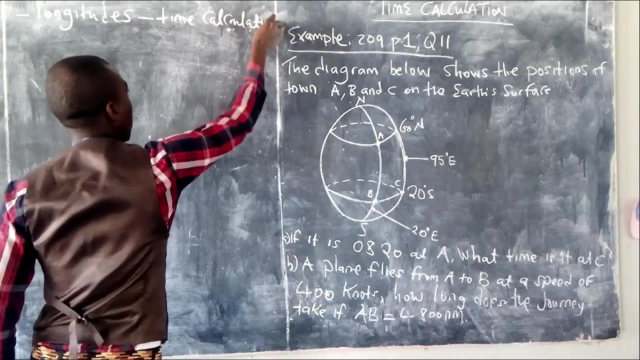 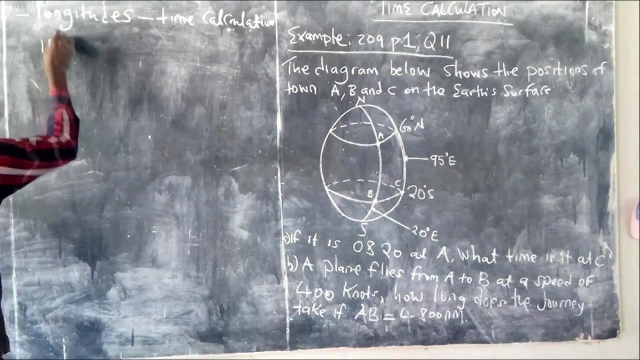 So longitudes are the ones that are used in time calculation. So these ones are used in what? in time calculation? Okay, So according to the standard measurements that we have, if you have to know that 15 degrees is equivalent to one, 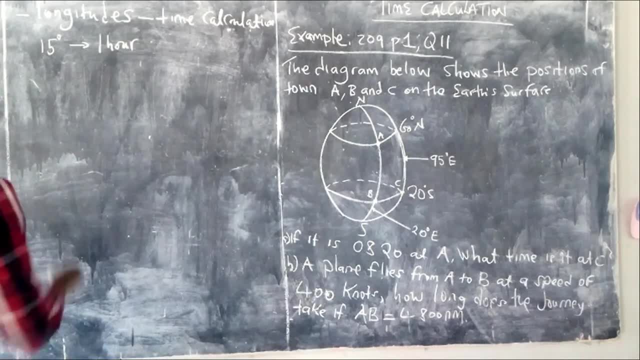 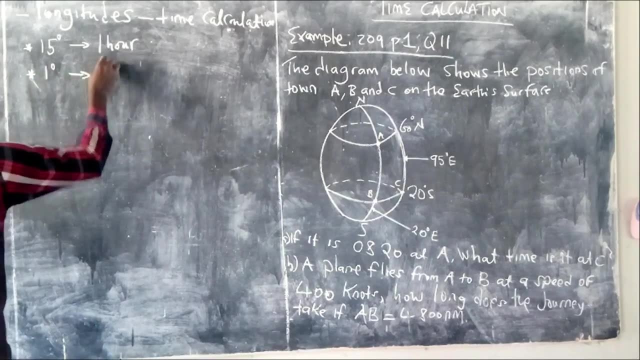 hour. So 15 degrees is equivalent to one hour. These are very important points that you need to know. Then you also have to know that one degree is equivalent to four minutes. Okay, So one degree is equivalent to four minutes. 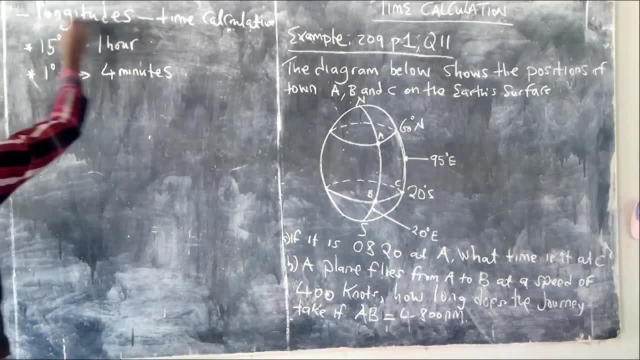 Okay, So having that knowledge then, also since we are dealing with the longitudes here. So whenever we are dealing with the longitudes, I'm sure you know that we have the east and the west. Okay, So the pose to consider here. 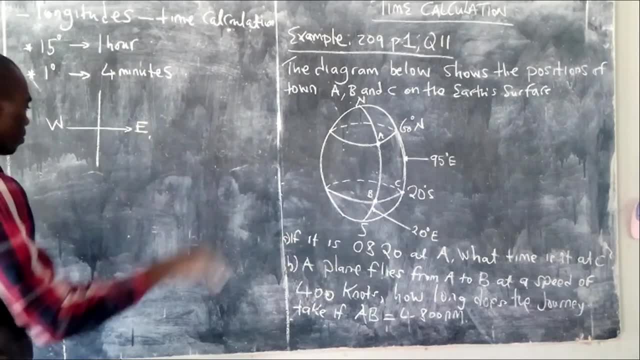 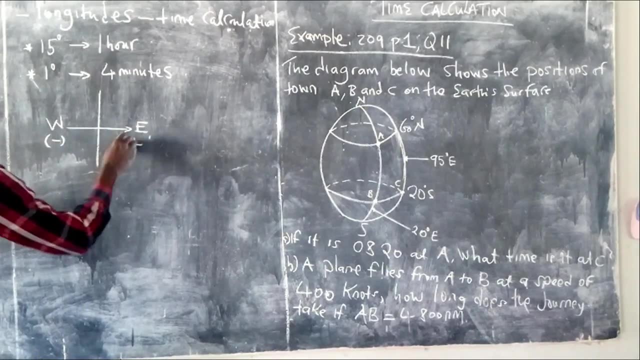 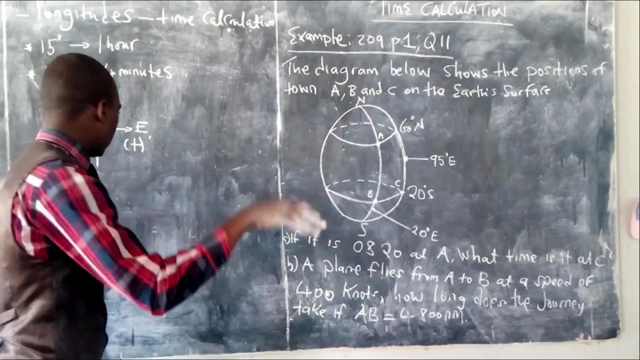 is the west and the east Now, just like what it is on the number line. when you are going to the west, you are losing what Time. When you are going to the east, you are gaining in time So that you should bear. 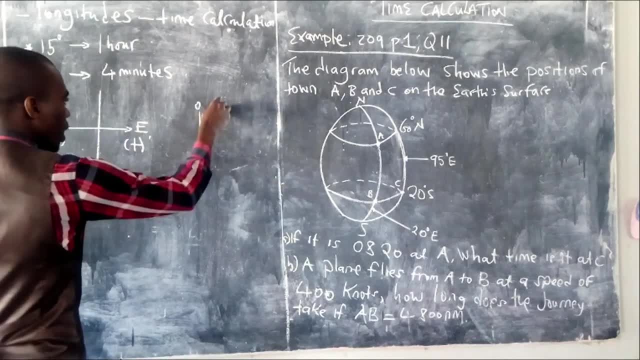 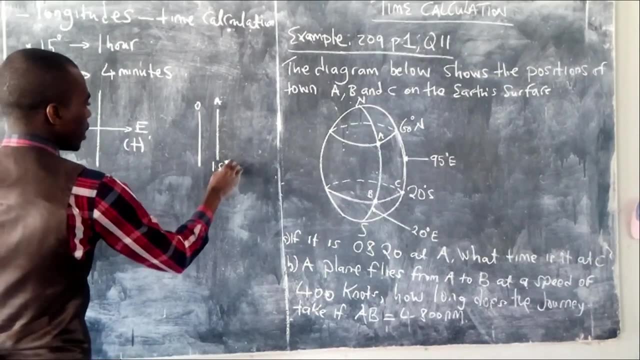 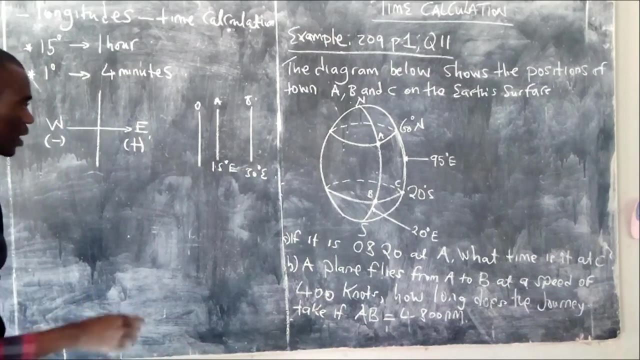 in mind. So what am I talking about? For example, if I have this is the GMT zero degrees, then I have this position here, which is maybe, let's say, 15, this one is 15 degrees. So what is happening here? 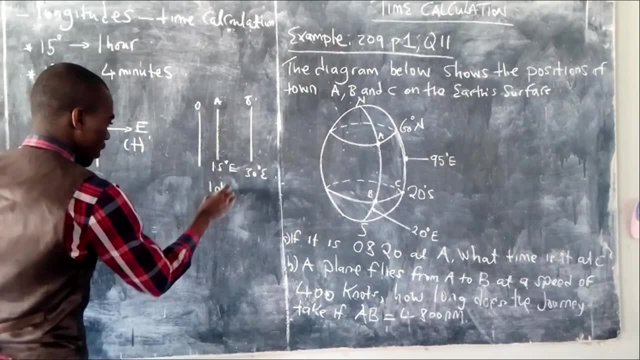 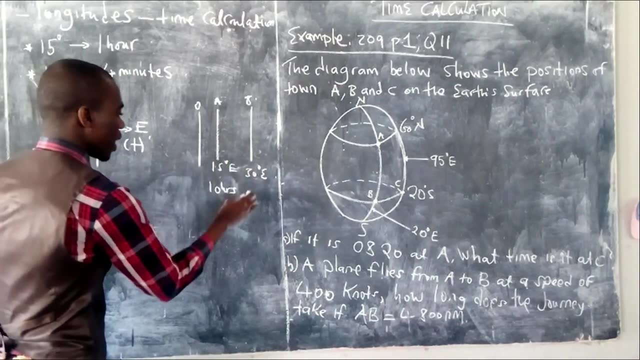 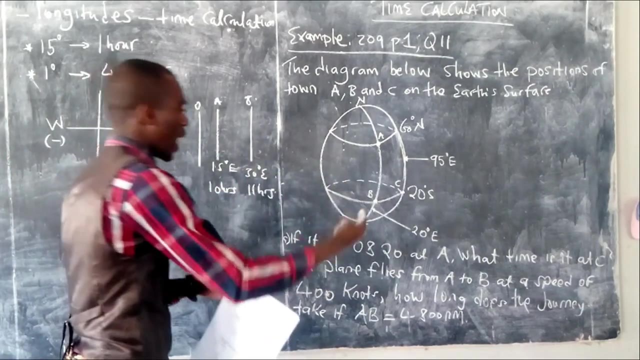 is this: When the time here at 15 degrees is, let's say it is 10 hours. Okay, So since you are going towards the east here, meaning at 30 degrees east here, we expect that here it is going to be 11 hours. 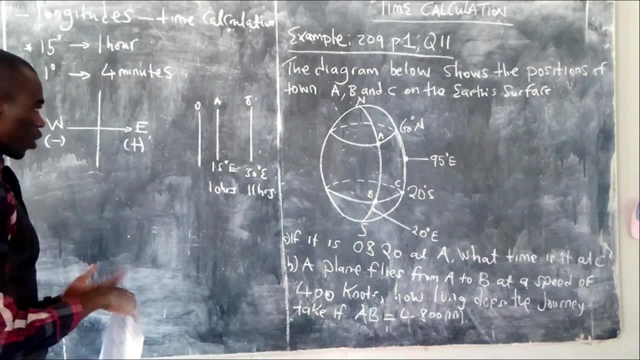 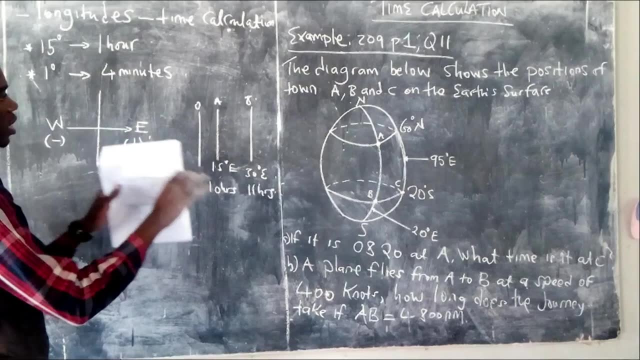 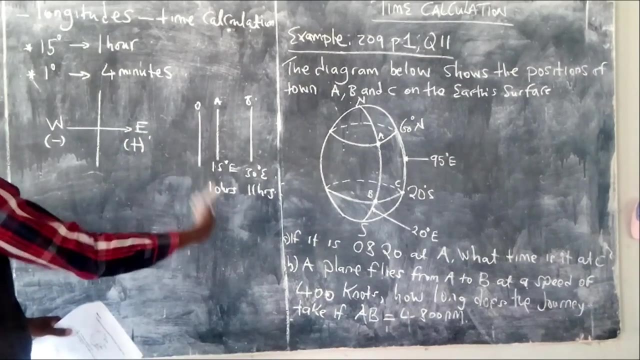 So you are gaining in time. So, as you are going to the east, you are gaining in distance just before we dive into the wadi, into the calculations. Okay, So we have had some knowledge about how to calculate distance. Now we are. 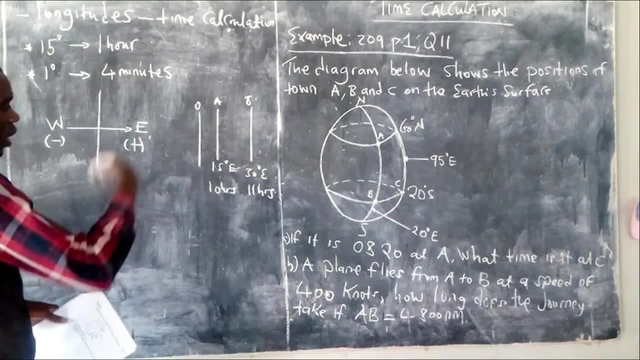 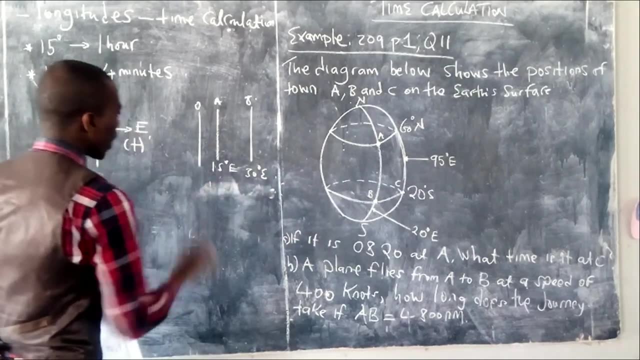 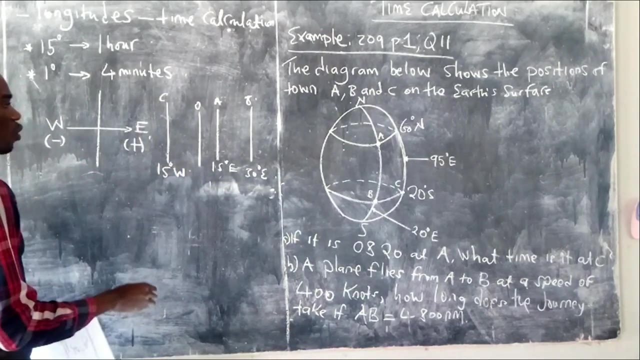 talking about how to calculate time. So, after knowing how to calculate time also, let me just remind people, like what we did in distance, we were saying: whenever you are calculating, for example, this west. so if you want to find the difference in longitude when you are on the, 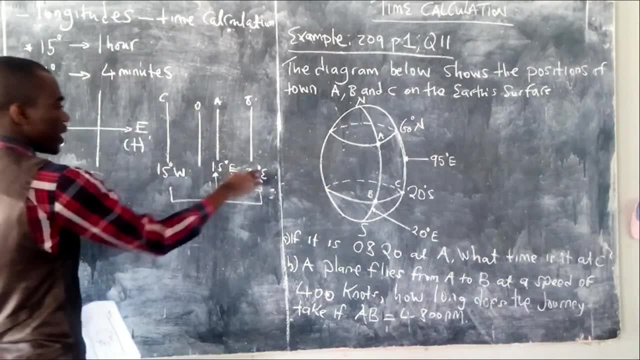 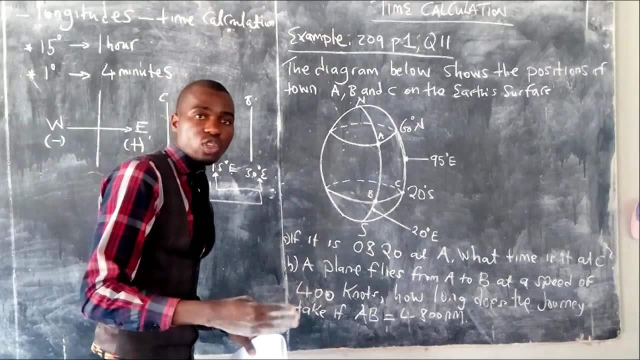 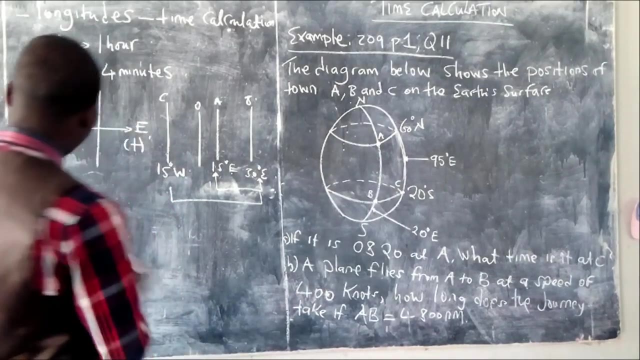 same side, the same side as in east-east- you subtract, but when you have two different sides- west and east- to find the difference in degrees you are simply going to add them. So that point is very important and it is going to work out very well. 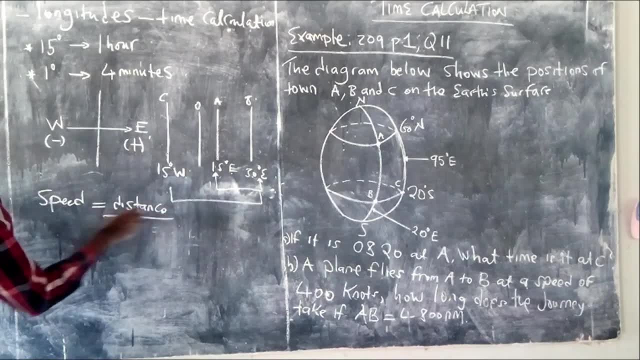 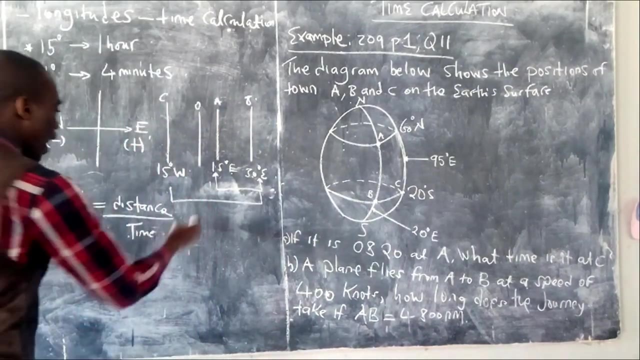 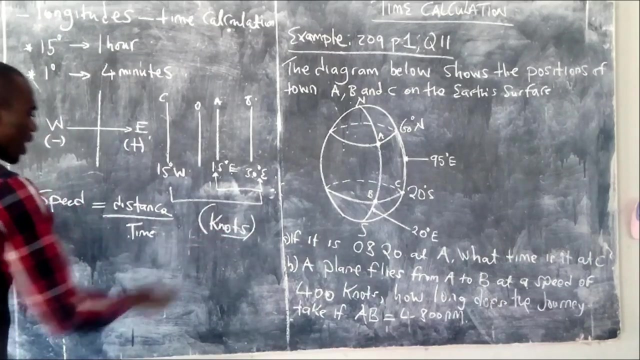 Speed is equal to distance over time. So speed is equal to distance over time. So now, when it comes to geometry, the speed is usually recorded in what we call knots. Speed has got the SI units knots, So these are the knots that 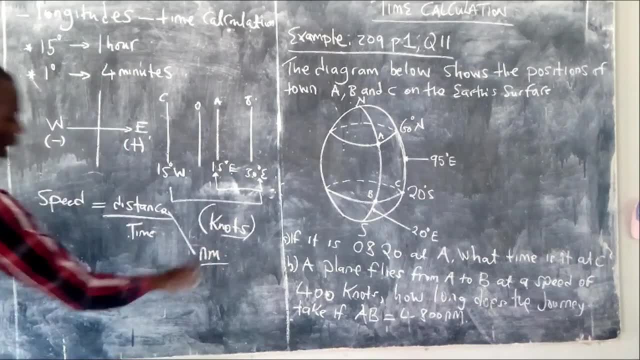 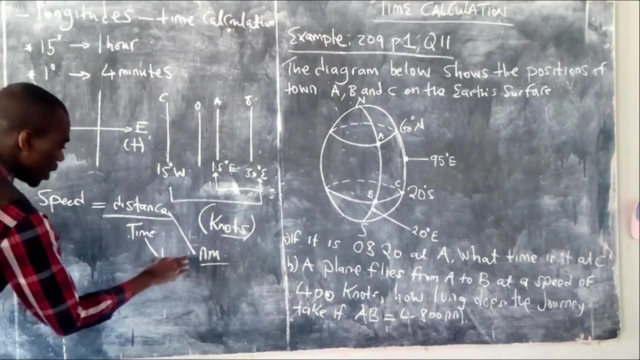 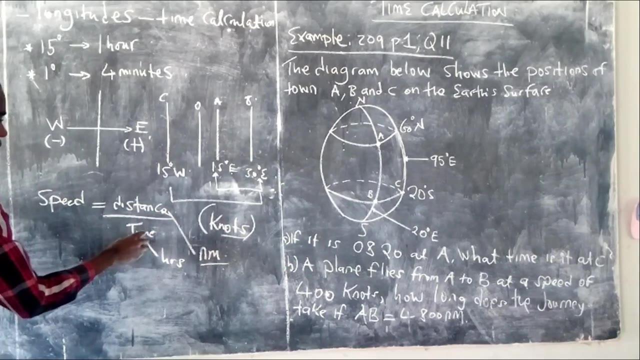 you are using here. The distance that you are using here is in nautical amounts. Make sure that the distance that you are using is nautical amounts and the time here should be in hours. So when you divide these nautical amounts, divided by the. 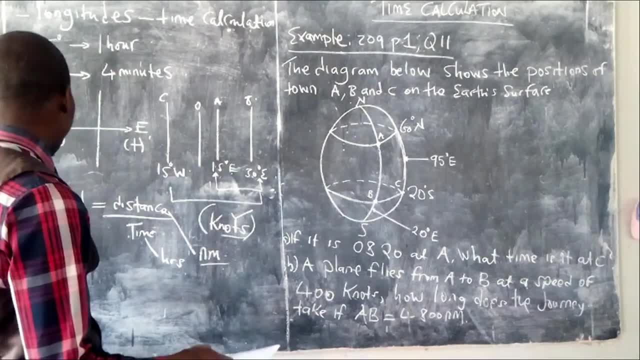 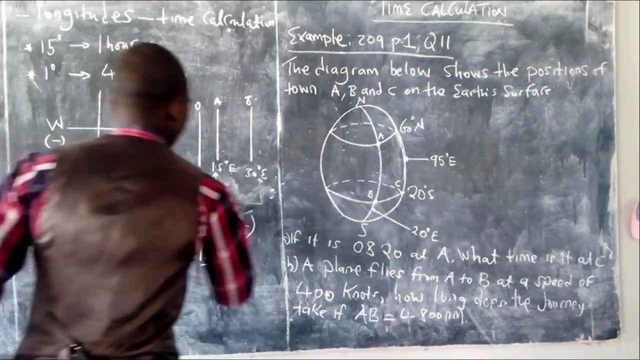 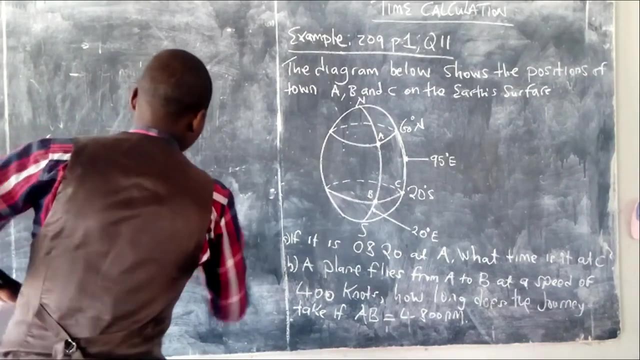 hours, you will be able to calculate speed and distance. Alright, So let's look at the example that we have on the board. This example has been extracted from 2019. mathematics, paper 2.. Mathematics paper 1, sorry, question 11.. 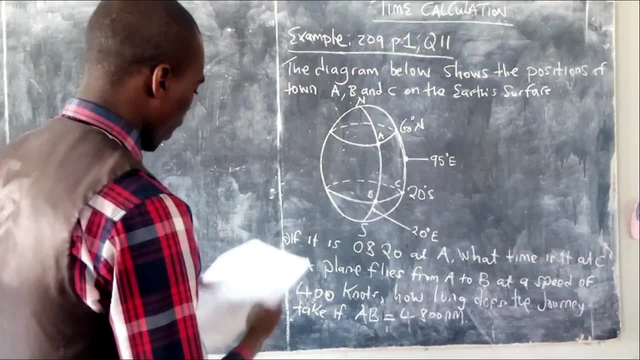 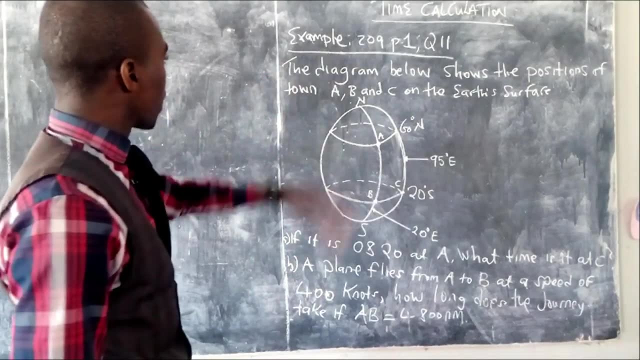 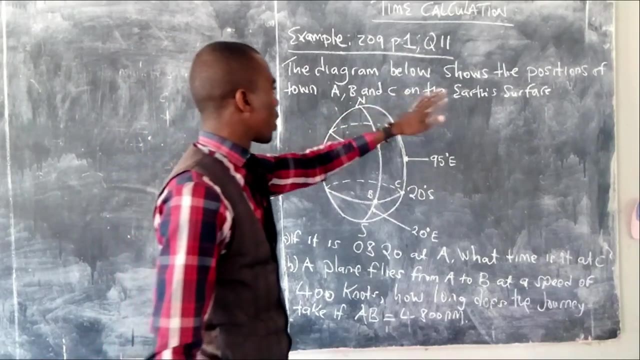 So this is paper 1 and we don't usually use a calculator, so we are going to do a calculator. so the question reads: the diagram below shows the positions of towns A, B and C on the earth's large surface. So this: 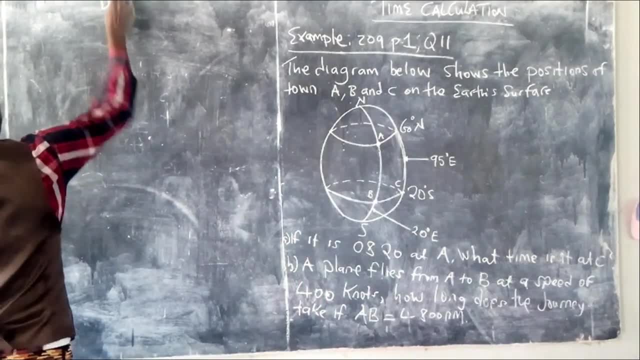 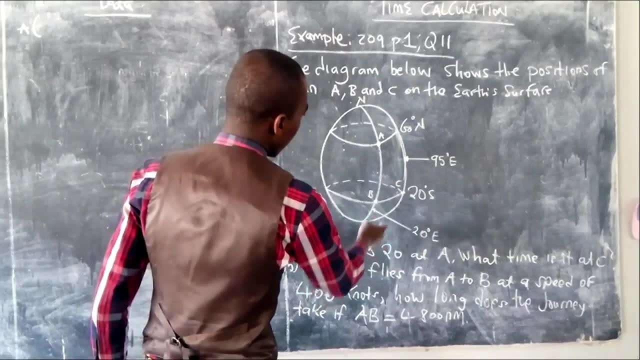 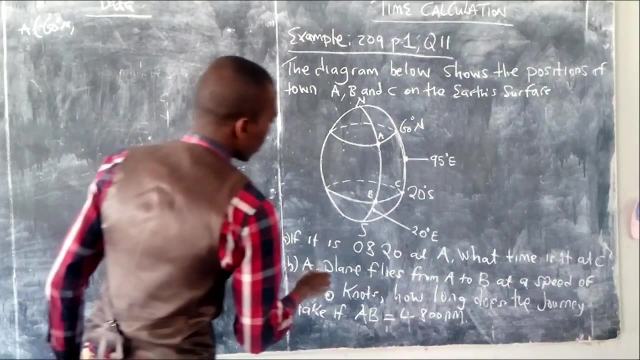 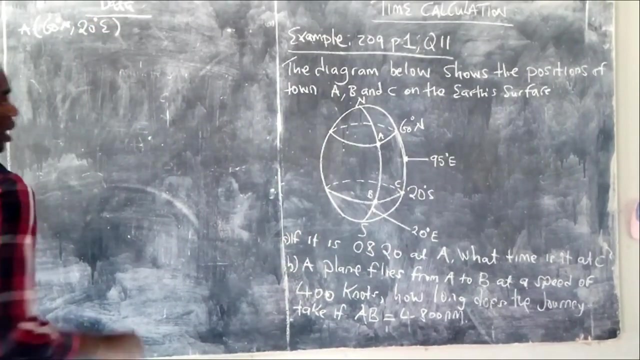 is what we have. We have a town, A, here. So if we are just to collect the data here, let's try to collect the data from the east. this is the east, this is the north. so here this is A it. 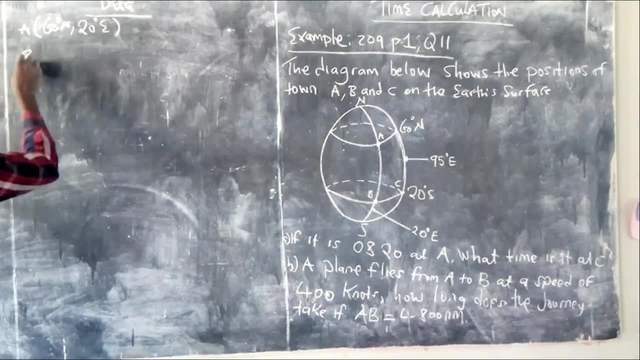 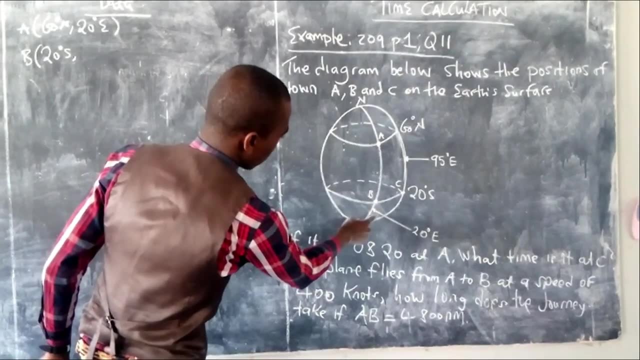 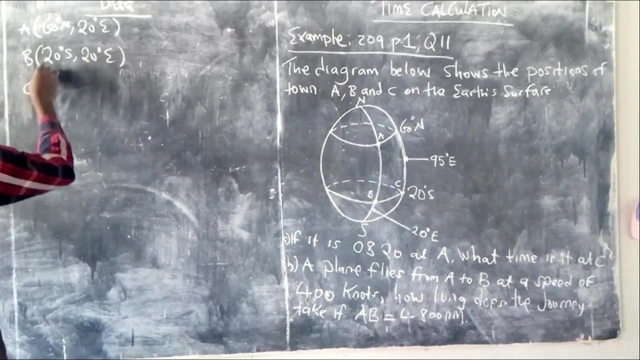 is on 20 degrees east, So this is 20 degrees west. Then let's go to town B. Town B is on 20 degrees south, So town B, you can see. this one you can see here is Gwani. 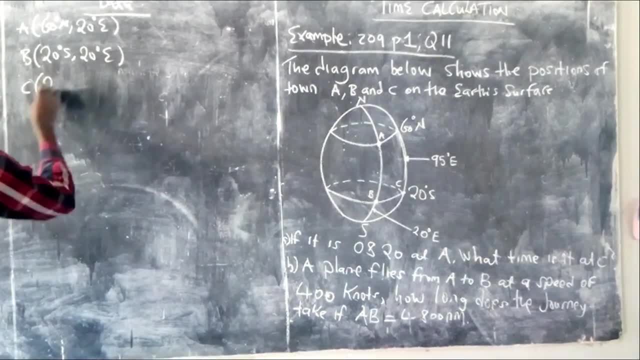 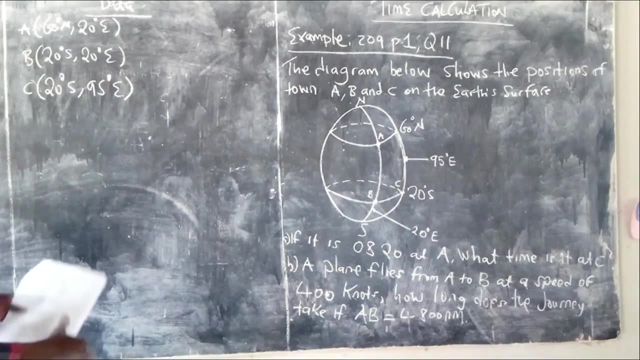 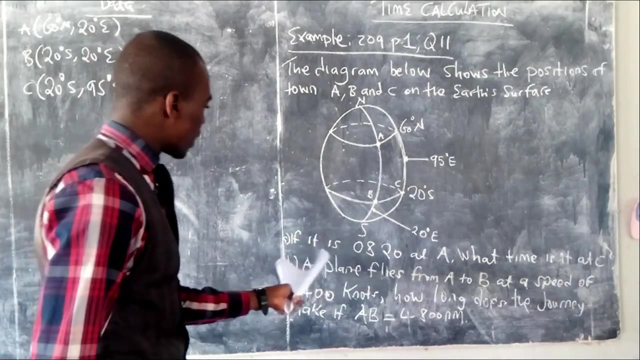 This one is on 20 degrees south, 95 degrees east. So 20 degrees south, 95 degrees east. So this is the information that we have. Alright, let's read the question A if it is 8 hours. 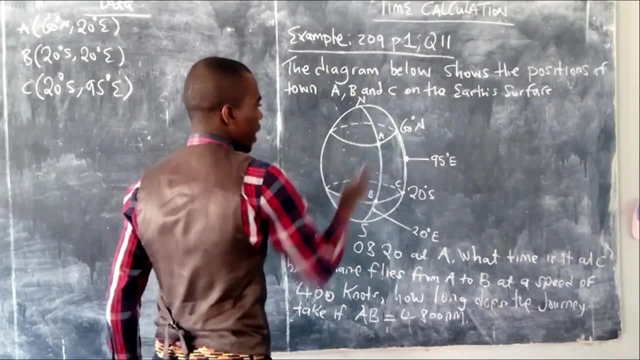 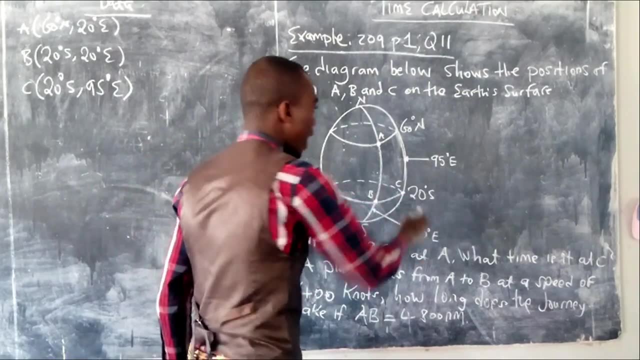 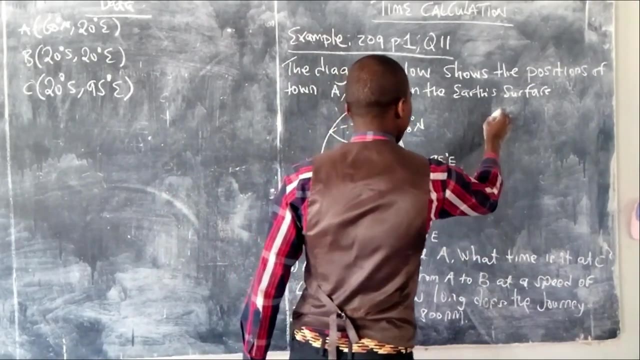 at A, then here at A it is 8 hours, Then here at C. what time is it? So now, if I can just try to interpret this information, it's like this: this is my A is on. 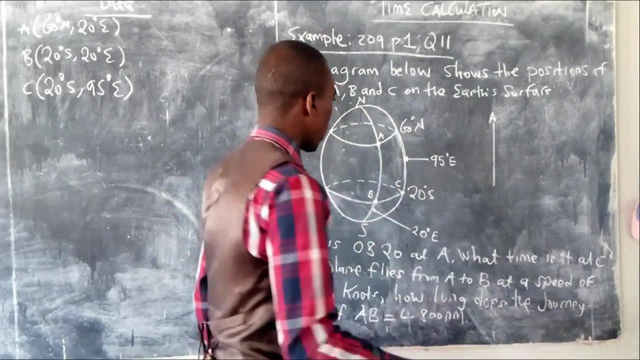 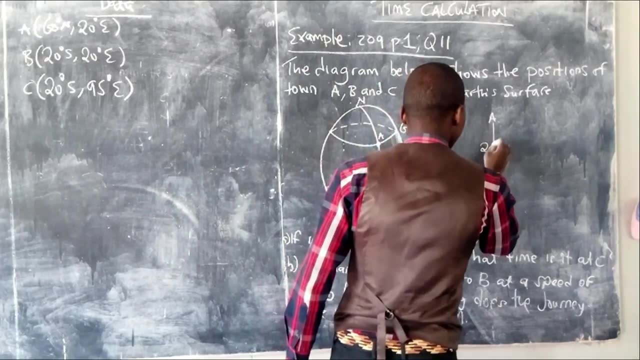 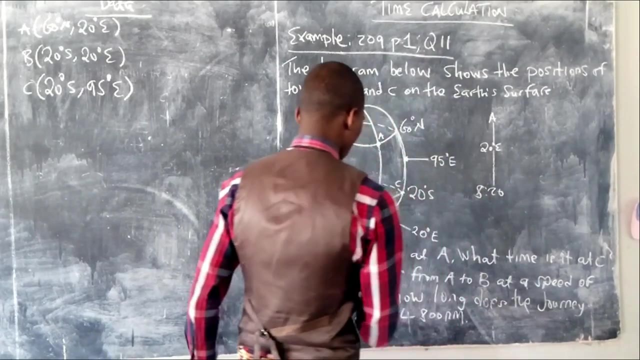 this one, so I write this line down. So this is actually given as this: 20 degrees east, And they've told us the time here is 80 hours 20 minutes, So it's 0820 at A. Then 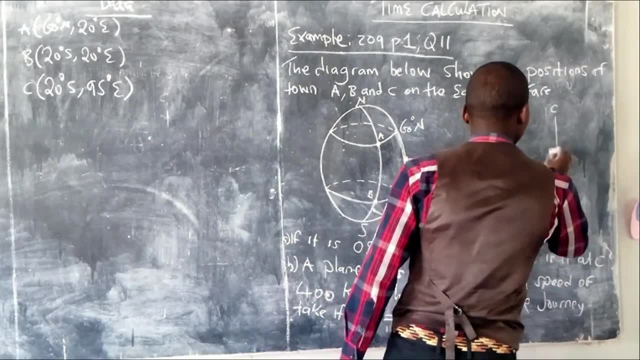 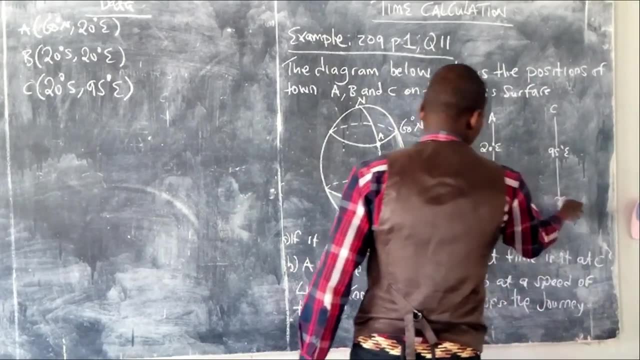 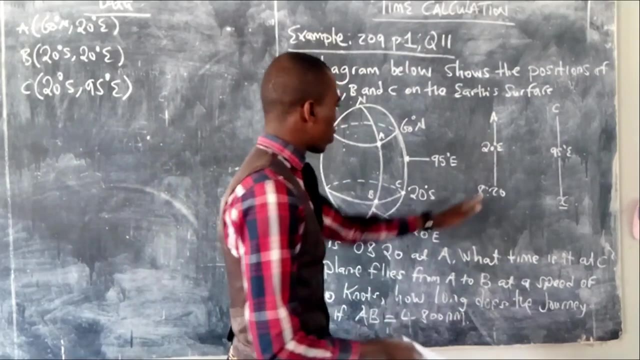 we are going to see. since C is also here, so our C, let me put my C here and this one. they've told me it's 0820 to 5.. Alright, so now, first things foremost, look at, we are still going. 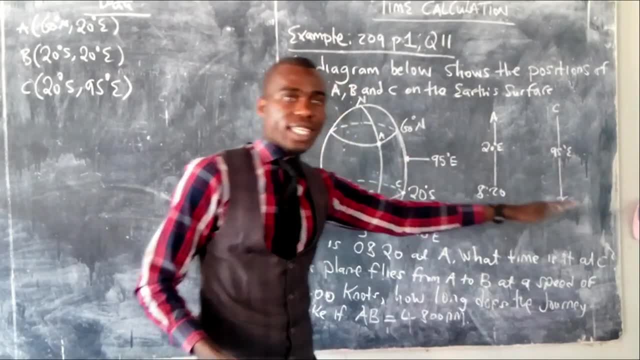 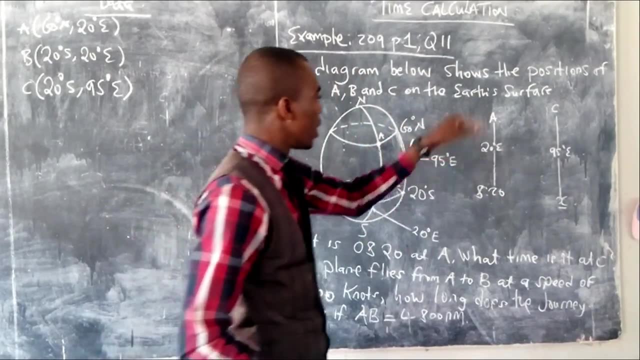 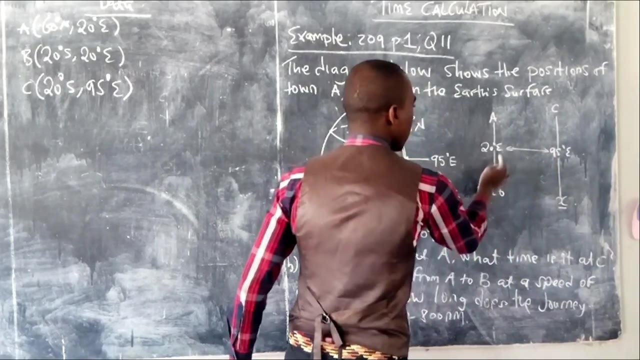 from 20 east to 95 east, meaning we are going towards the east, So we are actually gaining time. So if it is 8 hours, we expect it to be more than 8 hours in, So time always depends. 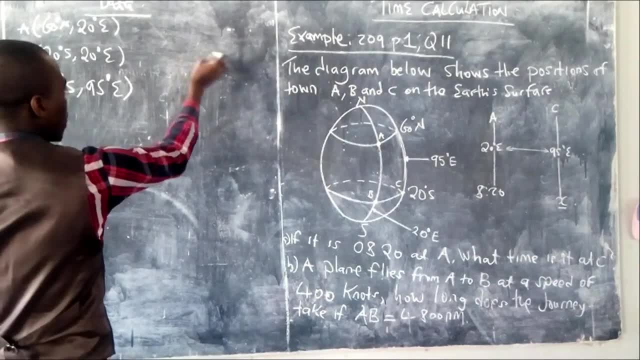 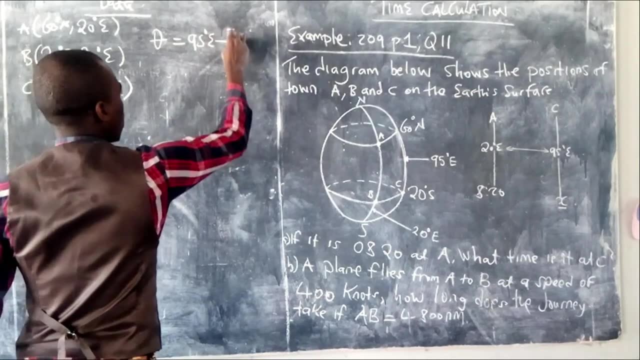 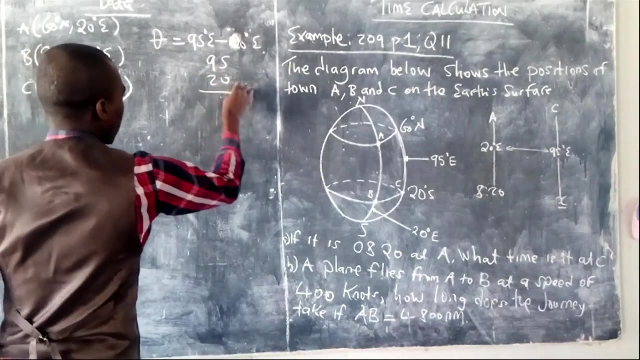 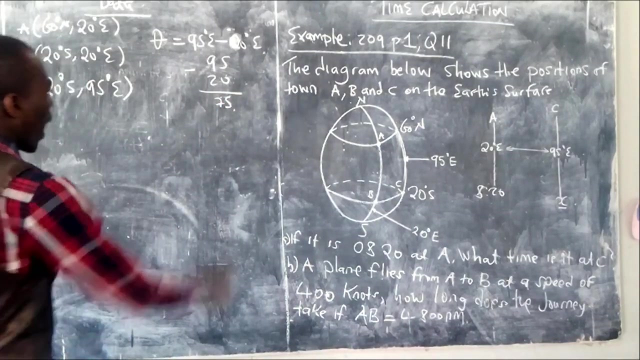 on what to subtract. So there the difference in the longitude should be equal to 95 degrees east minus 20 degrees west east. So because we don't have a calculator, let's try and do it ourselves without the calculator. So 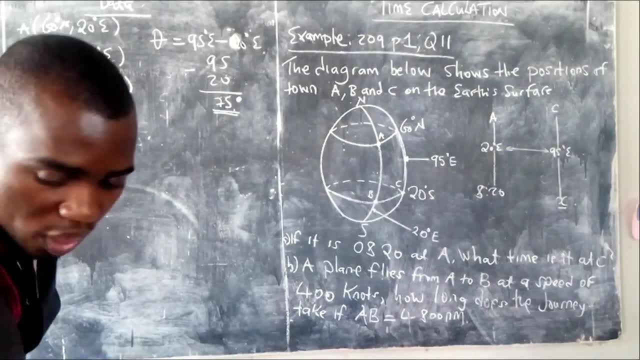 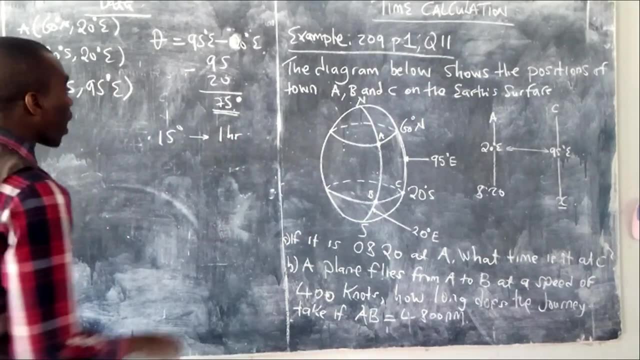 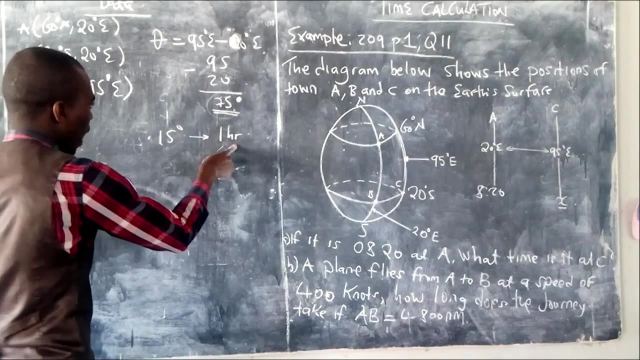 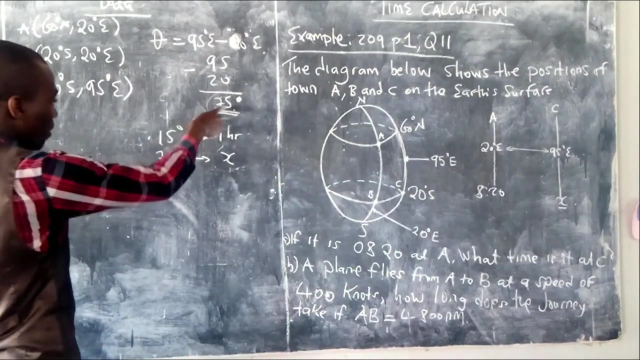 this is 5 there and we get the ratio which we get, which says 15 degrees is equal to 1 hour. Okay, So we are converting now these degrees into hours and using this relationship, we can say: 15 degrees is equal to 1 hour. 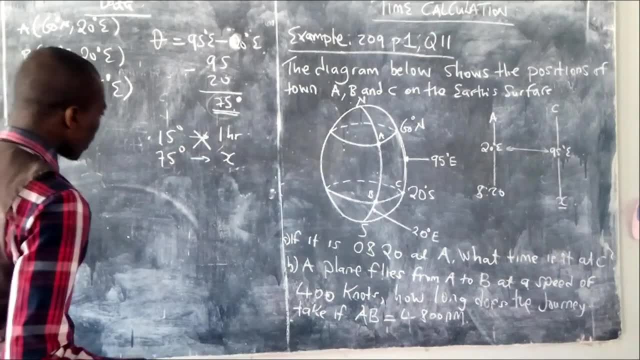 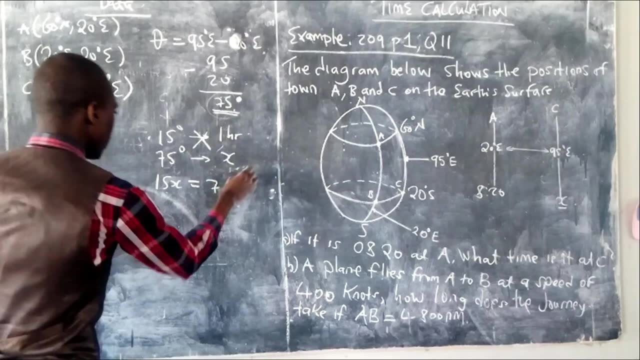 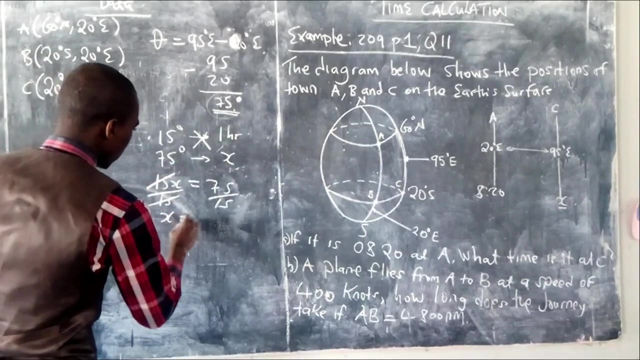 Then how about? 75 degrees will give us what. So if you cross, multiply this one, we are going to have 15x being equal to 75. Then we can divide there, we can divide there. So the secret. 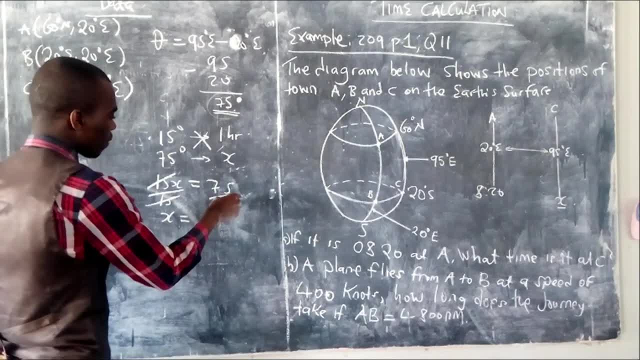 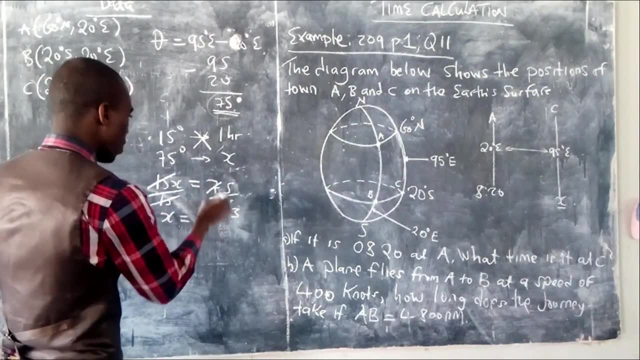 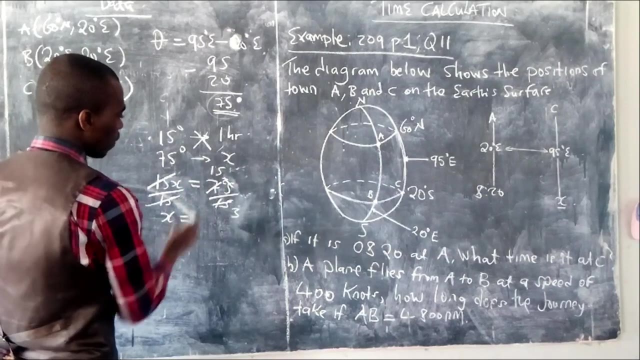 here is: if you are not sure about something, you can reduce these numbers. So we have 5 in here. we are going to have 1 times 2.. Then 5 in here. we are going to have what? 5 here? 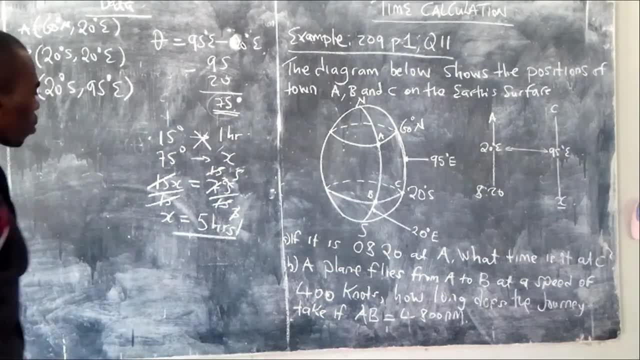 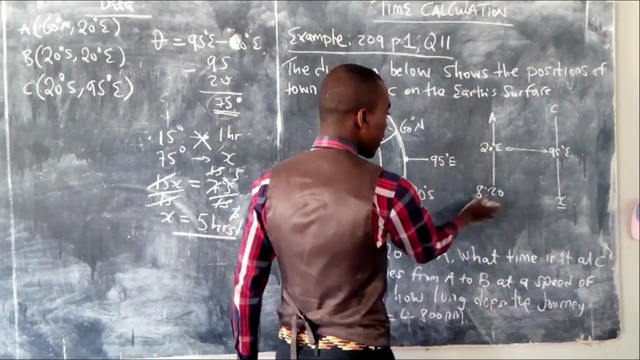 So that is 15.. Then 3 in 3, 1.. 3 in here is 5.. So it is giving us 5 hours. So the secret thing about 1 is whenever you add the time here. 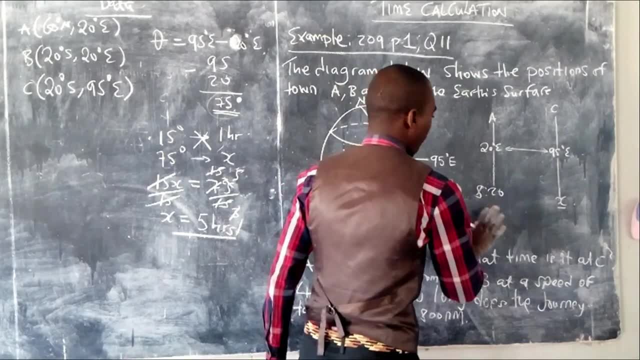 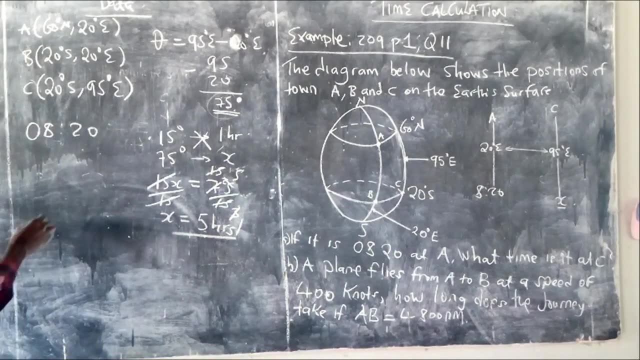 it will be 8.20 plus what. Since we are going to the east, we are adding the hours. So now that is where we add our time. So this is 08.20 here, Then 0 plus. 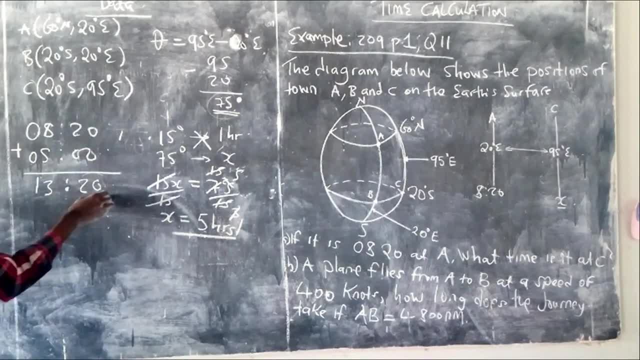 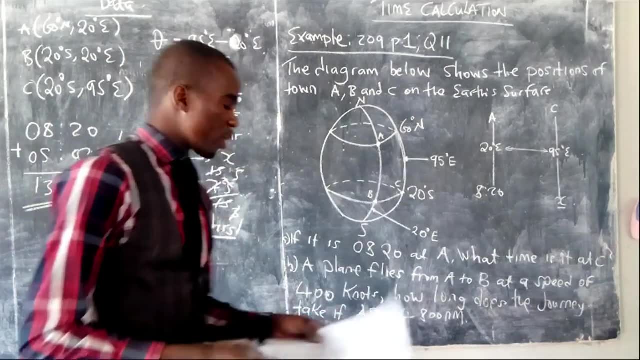 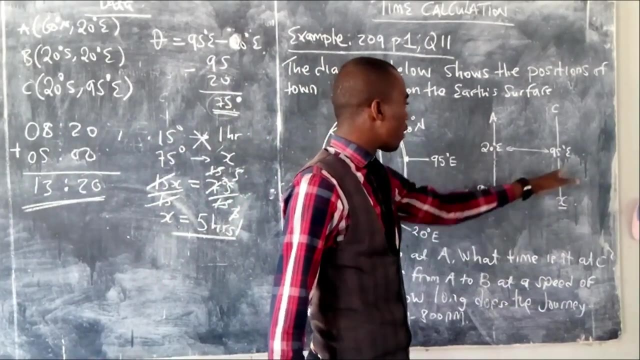 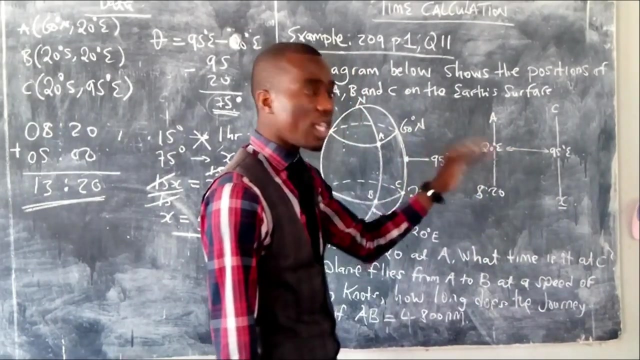 0 plus that one. So this is the time at what t at c. All right, So that is the simple principle that you are supposed to understand. So the first thing is find a difference in degrees, Then you convert. 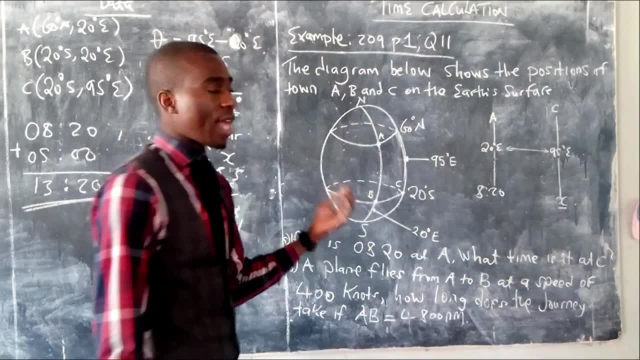 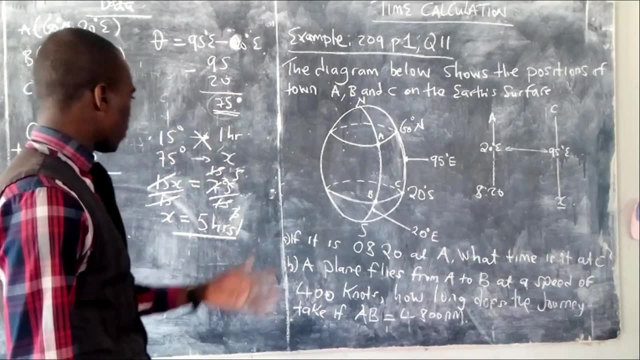 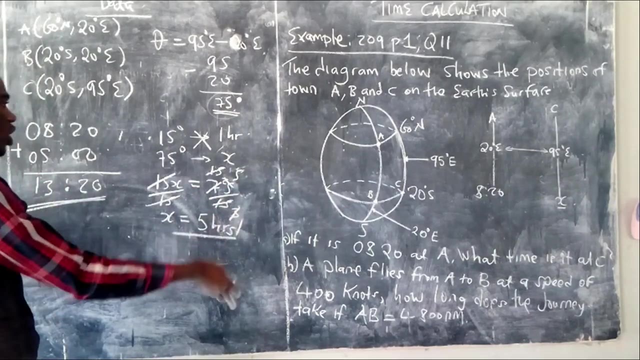 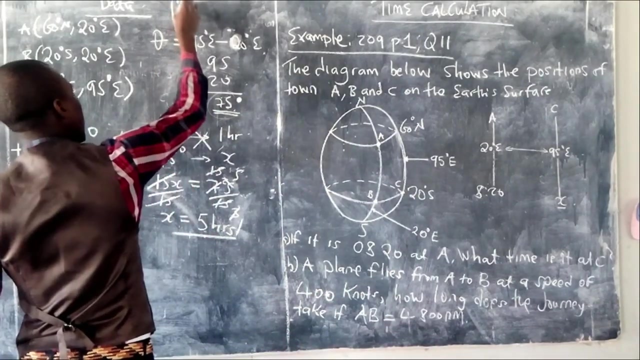 the difference in degrees you are going to subtract that time. So that is the simple concept that you need in order for you to successfully calculate what t time Supposing after dividing here you add some remainder, So that remainder you can just 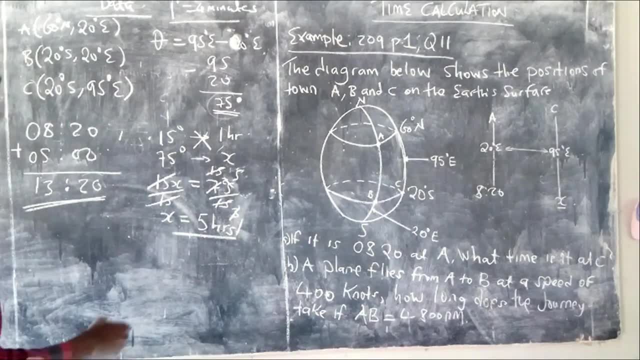 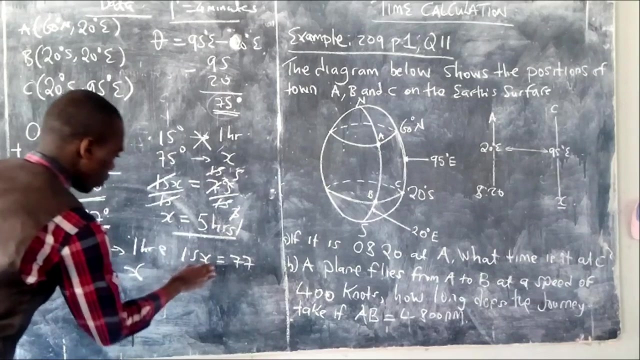 multiply it by the number of degrees you have in the time. So you can just give an example of that one. So supposing we had 77. Supposing we were saying 77 was the difference in degrees. So we divide. 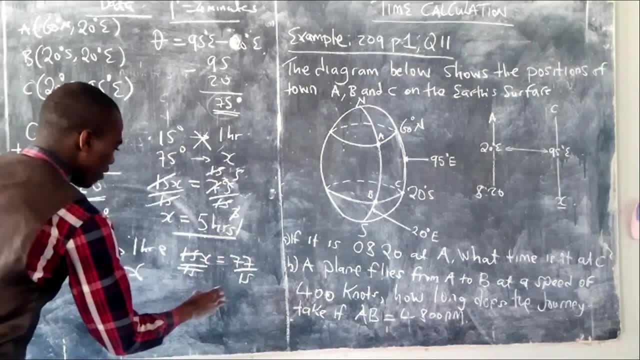 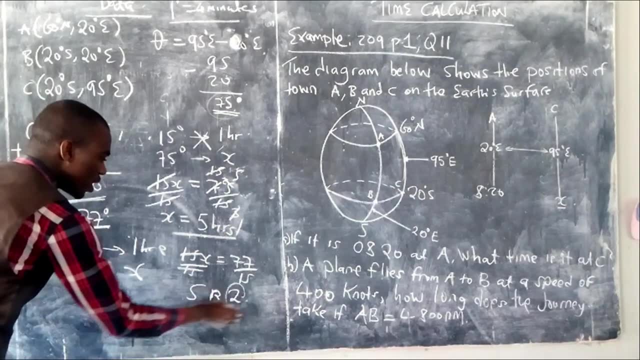 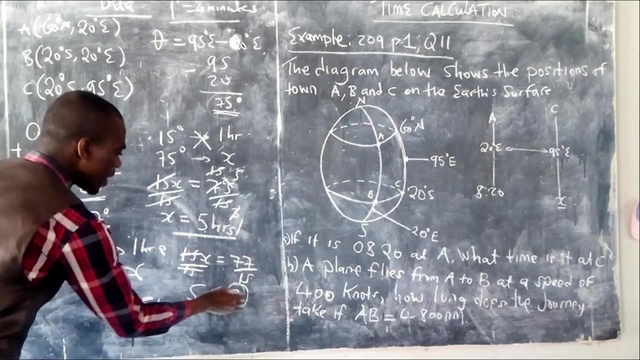 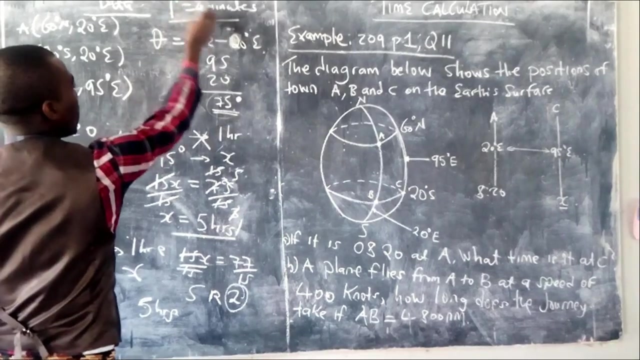 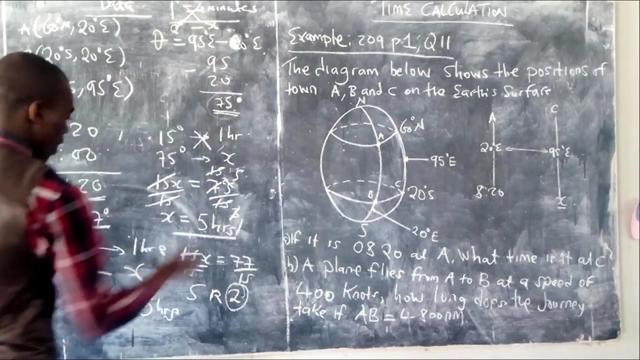 by 15 and divide by 15.. So here the answer could have been 5 b remainder, So 5 remainder 2.. Now what do we do with these two letters remaining? So this is equal to x, So 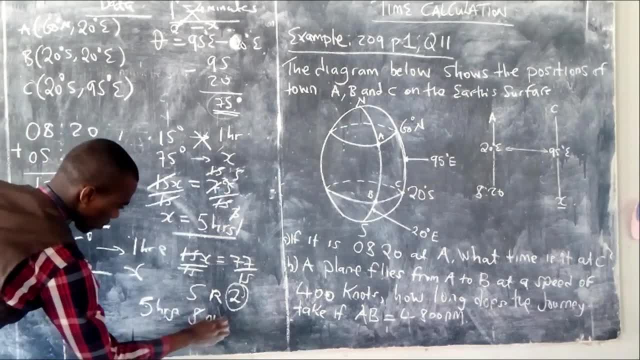 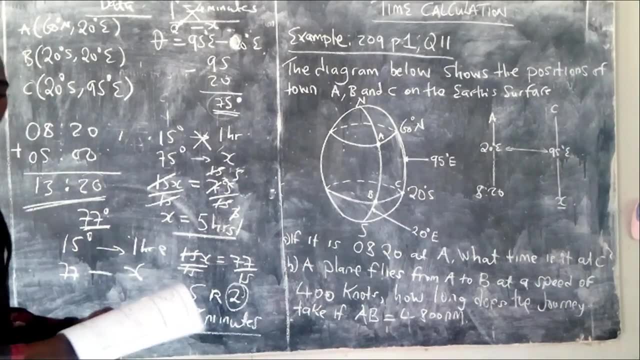 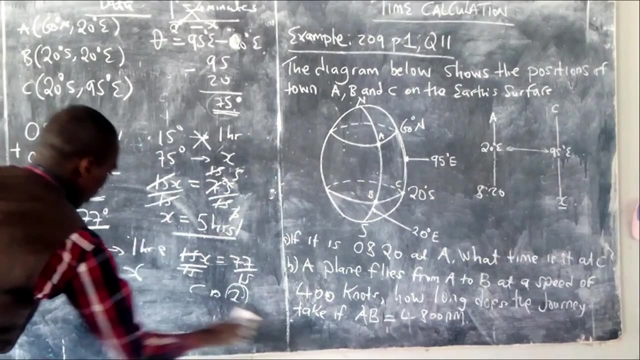 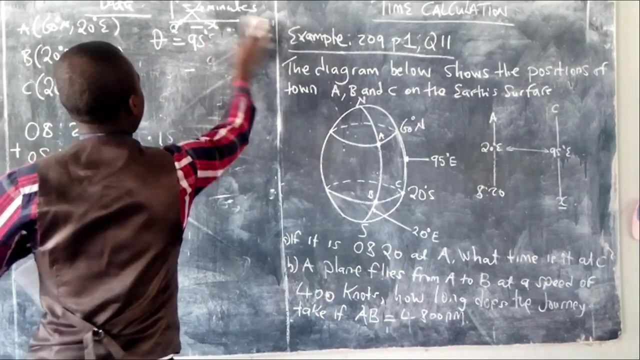 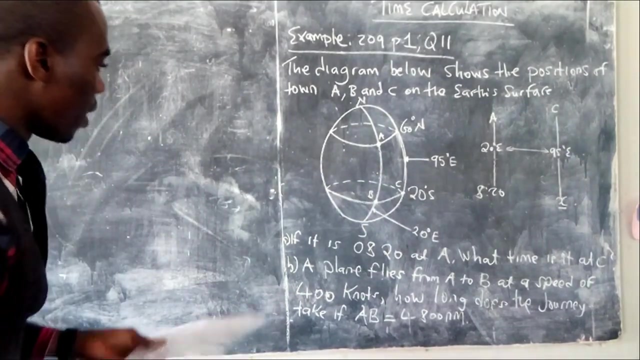 when you cross multiply, there you are going to say 2 times 4.. Then here we are going for 5 hours and 80 minutes. I'm sure you can do that. So what we are going to do is we are. 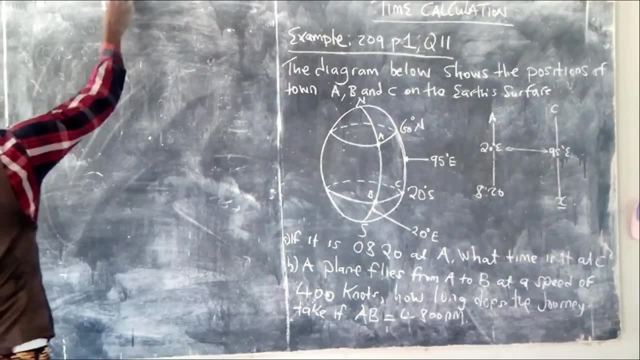 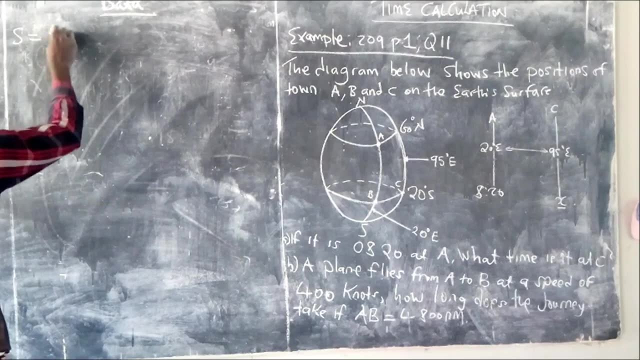 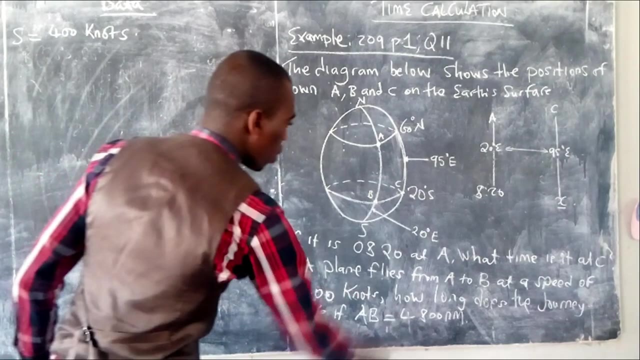 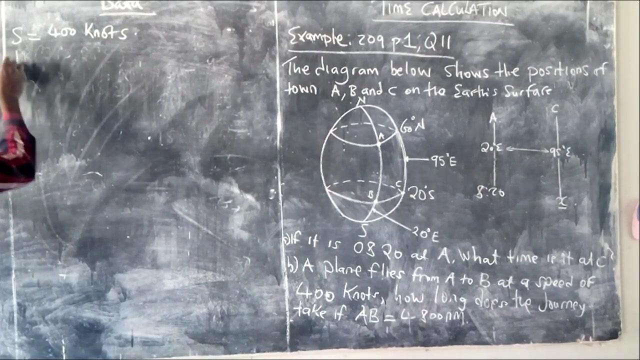 going to calculate the speed of 400 knots. So we are going to calculate the speed of 400 knots. How long does the journey take if mb is equal to 4,800 knots? So we have our distance, which is equal to. 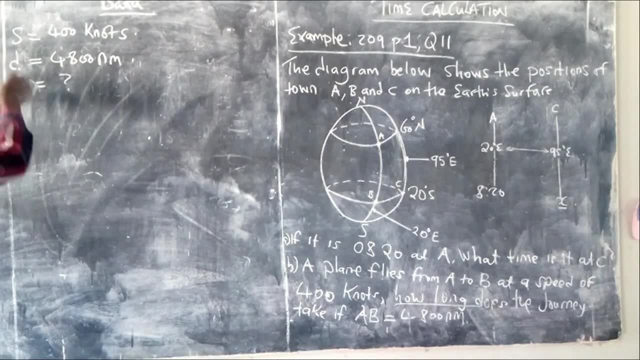 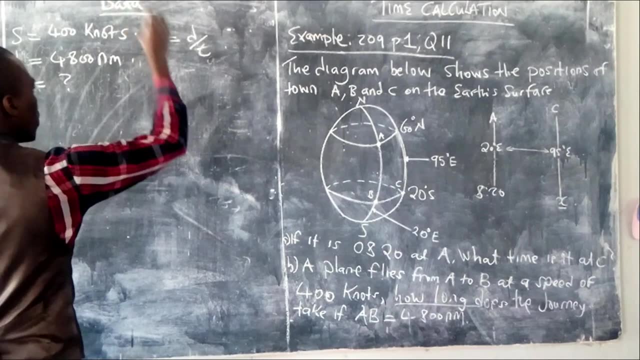 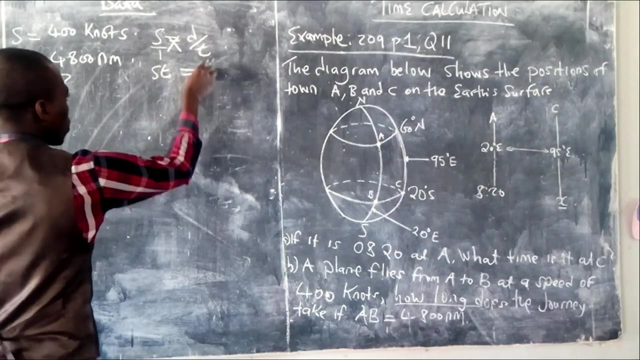 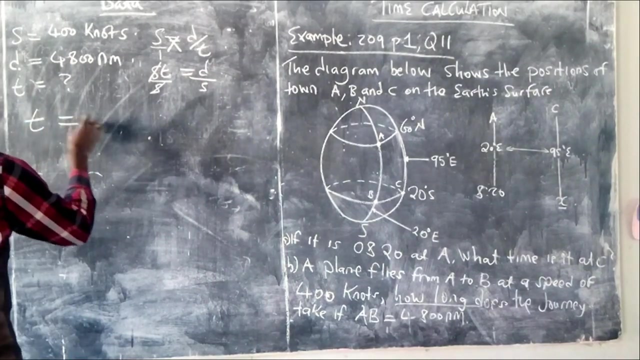 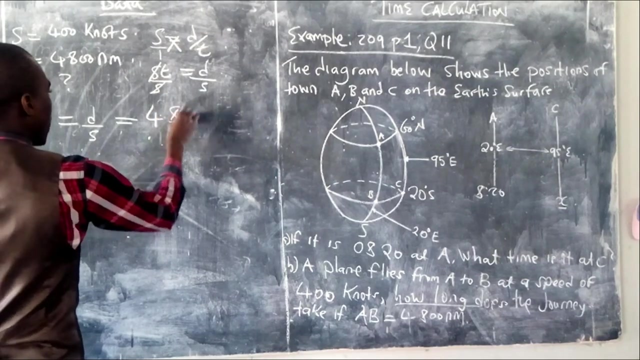 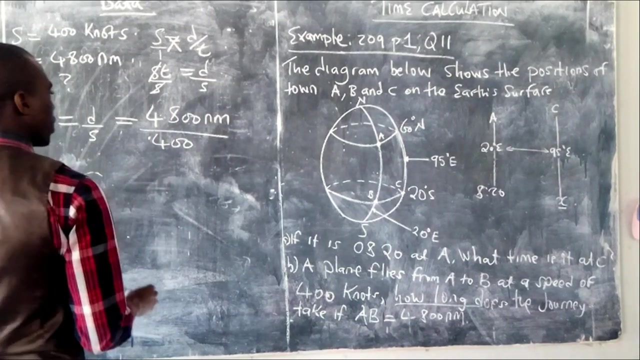 4,800 knots, Then how long is the distance over time? So since we are finding time, we can just make t into the formula. So we do that. We are going to have to calculate the speed of 400.